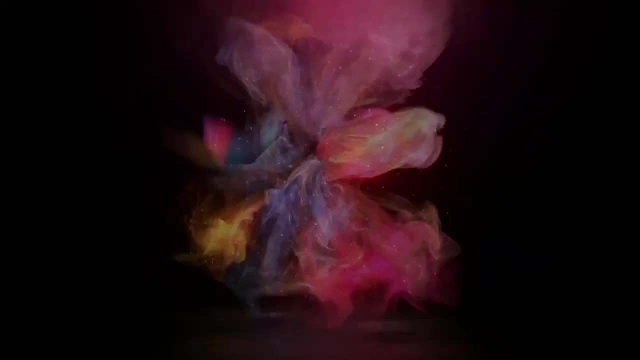 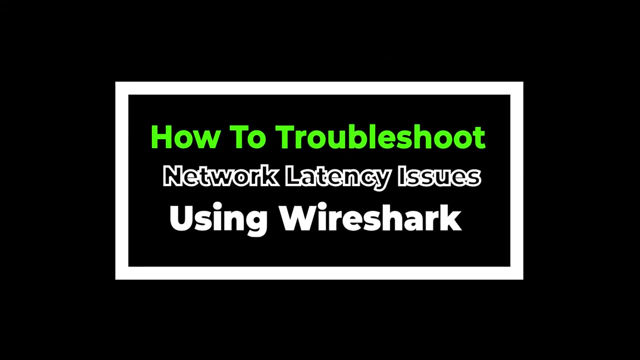 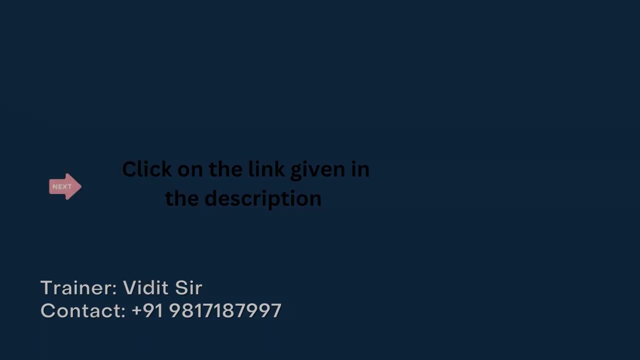 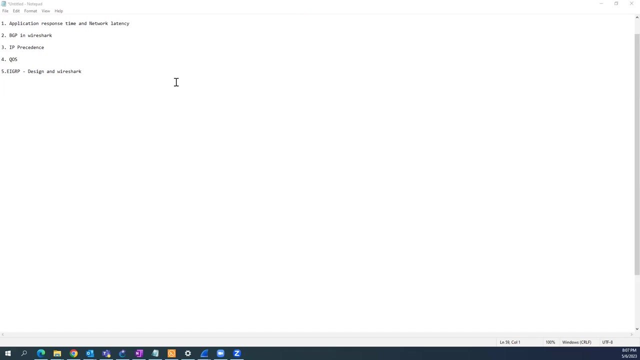 Hello, hi everyone. So today we are going to discuss about how we can find the application slowness, and we have discussed about network latency and now we will do a use case: how exactly we can find a network latency and what are all the key things we have to consider. 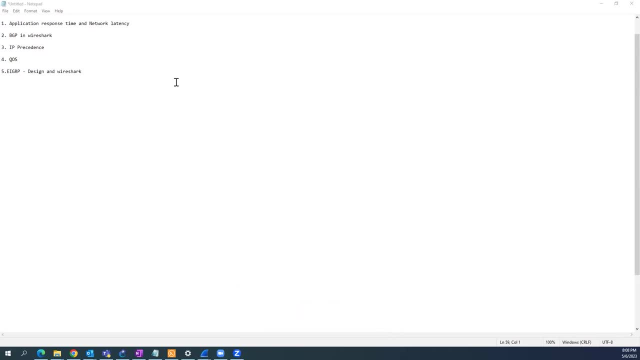 for network latency. So we are going to discuss about that and along with that we will discuss about how exactly we can spot issues with BGP. So what kind of information is being exchanged and how the Wireshark is going to interpret those details in Wireshark? 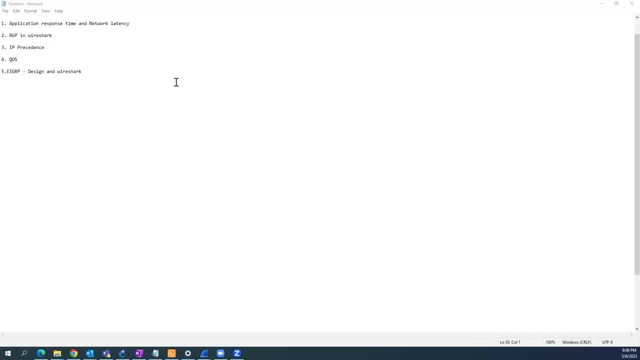 And this is all about not too much with the network topics. So here we can see how we can leverage the Wireshark to see the details for specific protocols like BGP and IP precedence value and what is IP precedence and how Wireshark going to interpret the IP precedence value. 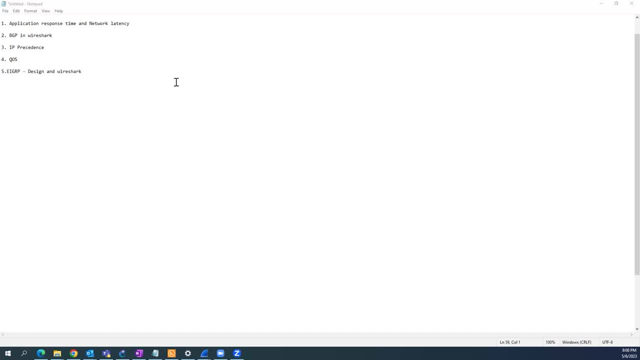 And a little bit background about QoS and the upcoming classes. In the next classes we will do a lab for QoS and we will discuss about how EIGRP exactly works and what kind of information that's been exactly exchanged and how Wireshark is going to interpret those. 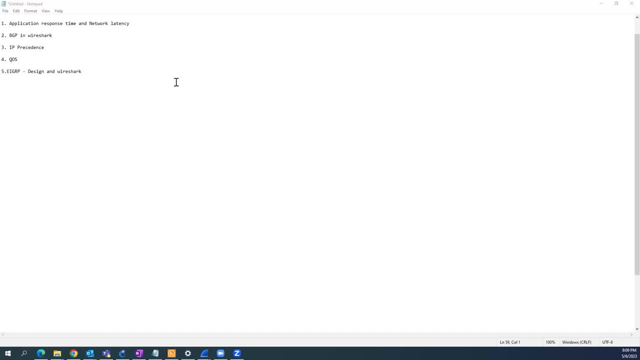 values. So we are going to discuss about everything. So to start with, let me start with the application Response time. So to do that, let me open my paint. So examples here, Let me take source And destination. So we all know that whenever the TCP connection establishment happens, it should be a successful 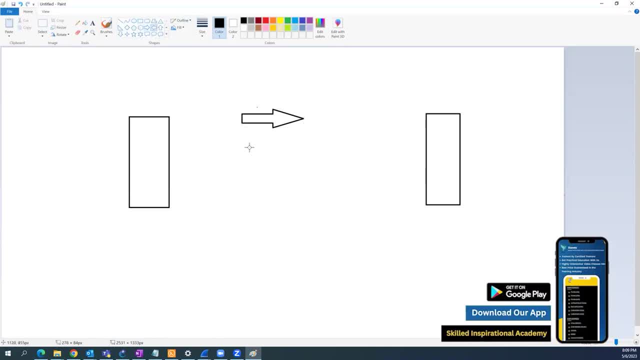 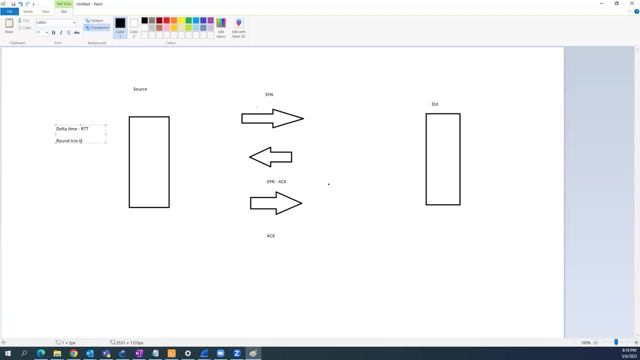 three-way handshake And this is source And this is destination: SYN, SYNAC and ACK. So in the Wireshark we'll look into these values. One is delta time: Delta time Also it is used to calculate the RTT round trip time. 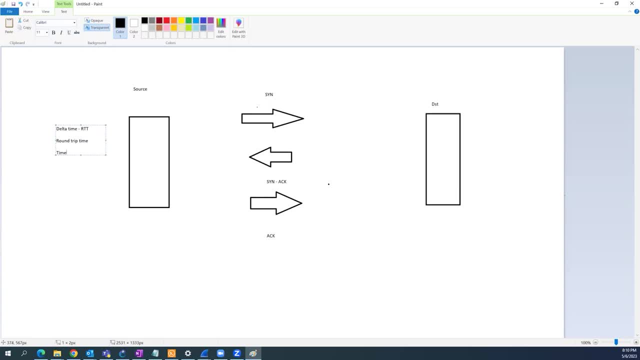 And along with that we use a time value- Time since the previous displayed value- And then we have depth value image- Okay, So per second. So these are the key things we look into in the Wireshark to find the network latency. 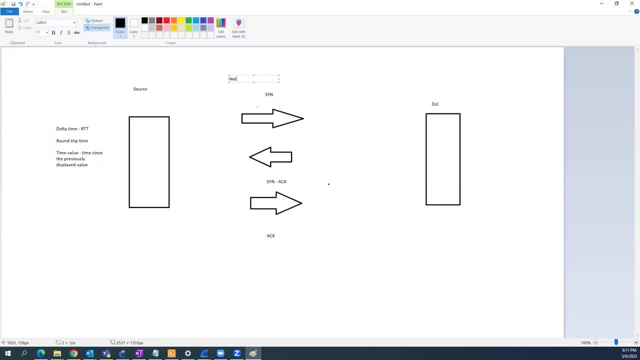 So, along with that, what are the other key things we should know about the network latency? That will be very interesting, So let us jump back to this. So, network latency, So let us look at network latency. So this is network latency. 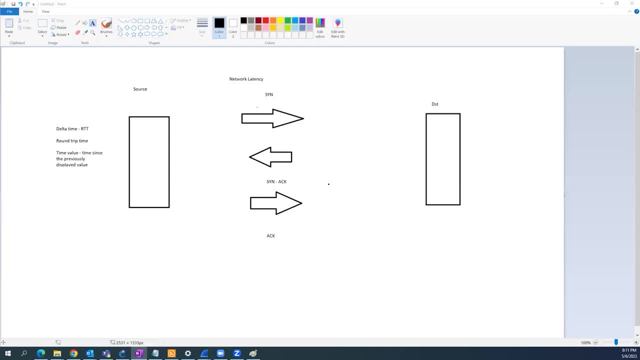 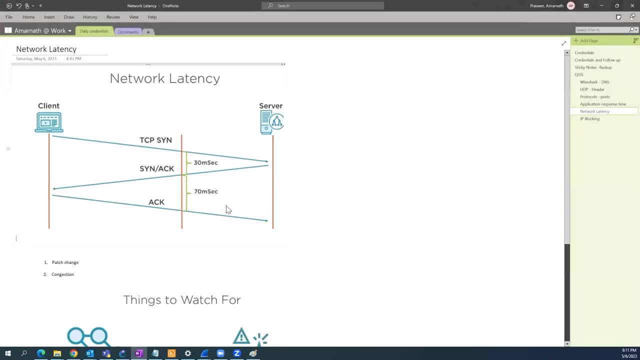 should know about network latency. if you look at this when we calculate the round trip time, so this is a client, so i send tcp sin and to receive my synac. so all it takes is for my complete round trip time. it takes 30 milliseconds. for the complete tcp connection establishment. it's 70 seconds plus 30, so 100 milliseconds. 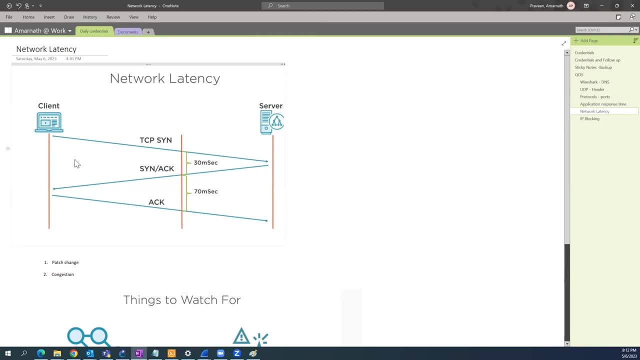 example, i am saying so this: how the round trip time is calculated on. okay, my source, the client, it's an tcp sin and for that i receive a tcp synac. so example: here i started, the connection established with 30 milliseconds, that is the underlay correction over the transport, the tcp. 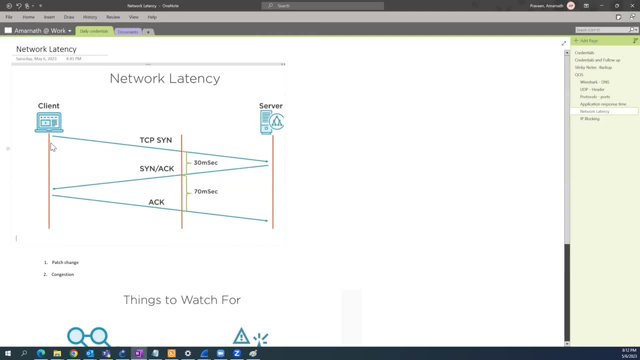 it takes 30 milliseconds, takes 30 seconds, since i send a pack, since i send a tcp sin until i get a tcp synac. so it takes 30 milliseconds. that is my network round trip time. that's how we calculate, so where exactly the application comes in, so how i can find it's an application slowness. 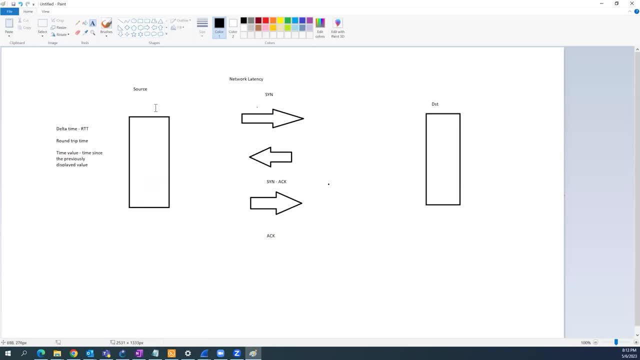 so the logic behind that is something i have to look into: my network round trip time and if my network round trip time says network round trip time, it says 30 milliseconds and after this connection establishment your actual http request happens. so from the client, once this connection is. 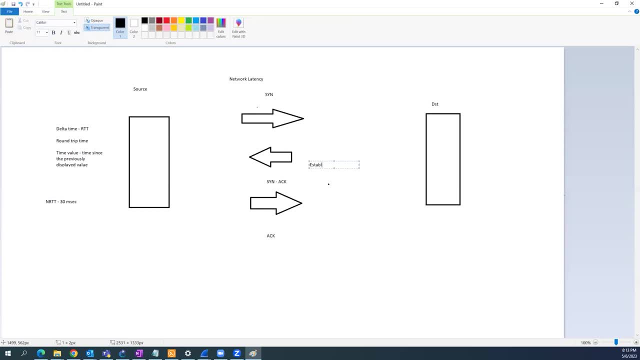 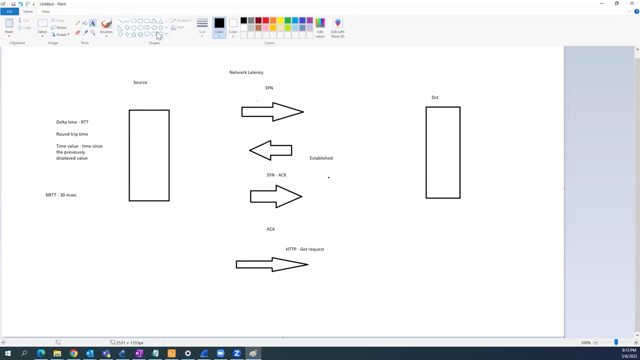 successfully established. next comes your http get request from the client. for this http get request i should get a reply from the server. that is http, okay. so after this, my actual- you know- data transfer happens over http. so this is layer 7 and this is layer 4. 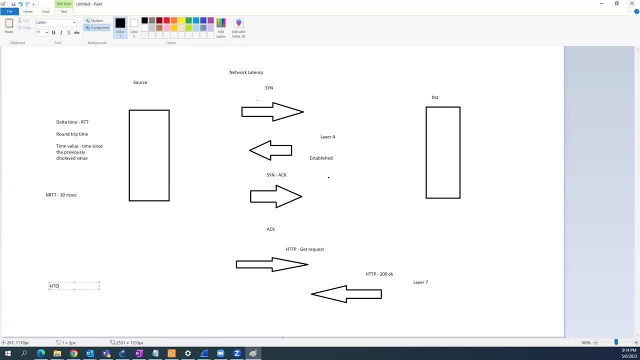 so here my http for my http request. if it takes 20 milliseconds, sorry for for my http request it takes example 50 millisecond. for my http request it takes 50 milliseconds. so my actual network wrong trip time. that is the time which is taken on tcp it is 30 seconds but my connection established successfully. it means that it means. 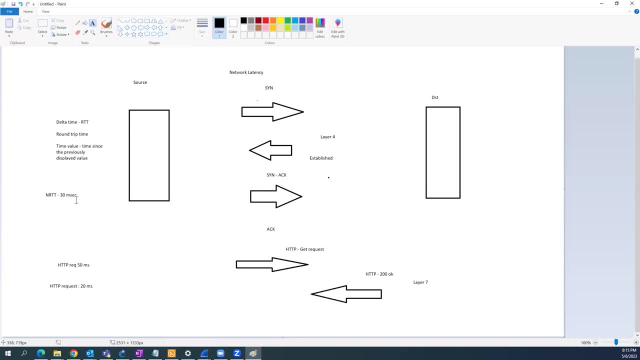 my network is stable and i get this request within 30 milliseconds. my my network round trip time is 30 milliseconds, whereas for my http request it takes 50 milliseconds. so the 20 milliseconds it's, you know, greater than that at 30 milliseconds. so it doesn't mean that my network has some problem, it is not something. 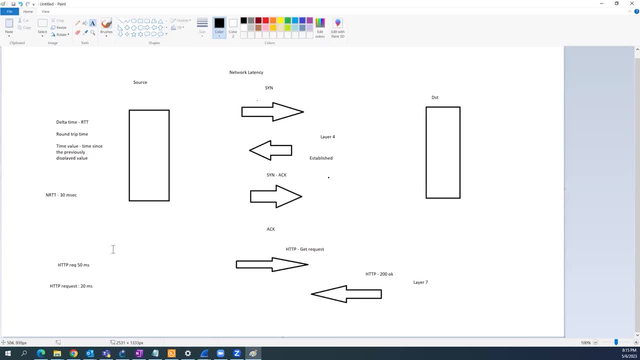 problem with the network. it's something with the application. so this is how we can figure out. so in the caption we'll see how exactly we can differentiate those. yeah, we'll talk about that. uh, so the what i'm trying to say here is: so the network round trip. 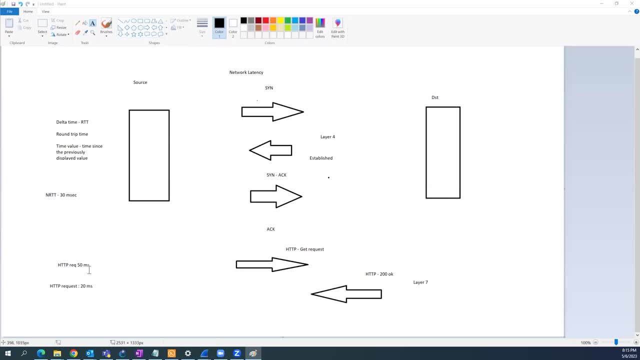 time is different from your http round trip time. so this is a layer seven and this is layer four. so as far as your layer four is good and there is something problem with a layer seven, then you have to check who is taking, you know, longer time to respond. 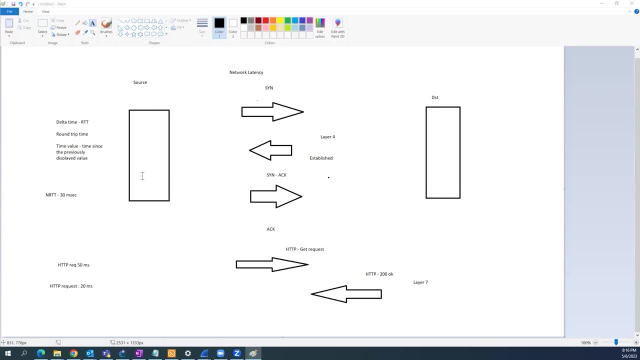 on. is it a client or server? so, but the first thumb rule is whether i have to the takeaways. is it a problem with the network or it is a problem with an application? so for that you have to be familiar with what is delta time, what is round trip time and how round trip time is. 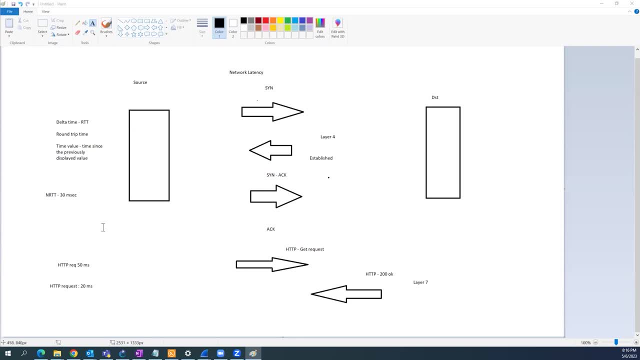 calculated and what is initial round trip time? example: if my communication happened with 30 milliseconds and maybe in the 10th packet in the source, the source again for my tcp connection, if the value jumped from 30 milliseconds to 50 milliseconds, so it means that my network has some problems, so i have some bottleneck. so always my. i have to compare my initial round trip time. my initial round trip time is the when exactly the the tcp connection establishment happened. back then if i had some problem, and my time taken has been increased from 30 milliseconds to 50 milliseconds. so that is something i have to look into. my 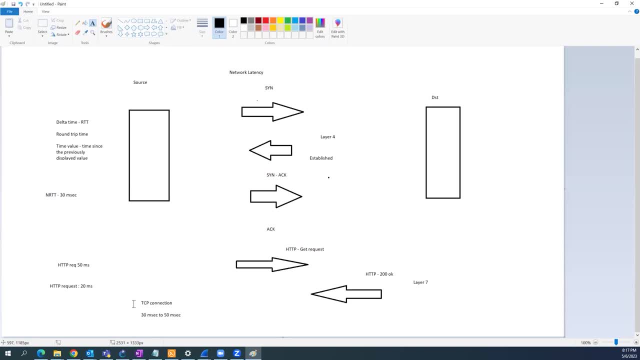 network that there could be some problem. we have to figure out that. but even for all the communication until your tcp fin packet, if you see your network round trip time that stays and sticks to 30 milliseconds, it means that your network connection is stable and there is something problem with your application. 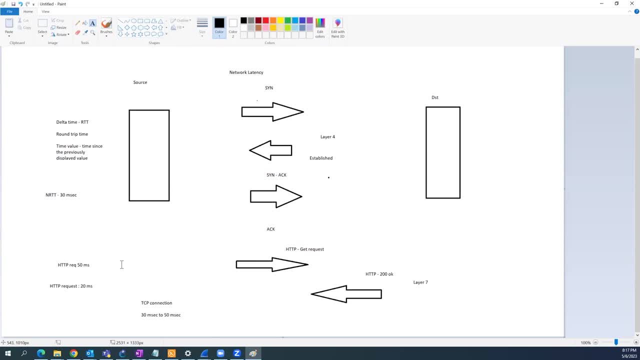 so this is how you can differentiate. is it a problem with the network or it is a problem with that http? it's a layer 7 or layer 4. so this is how you can differentiate and you can spot exactly where the problem is. so now let's see a capture. 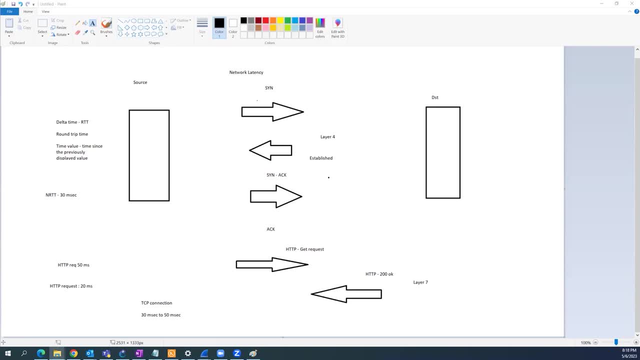 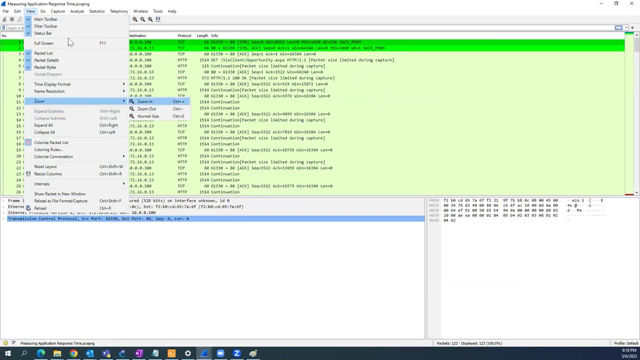 but in dairy, which is a field called concoction, this is a state low light and it saves a lot of time for one cloud because it has three fibers. it is not required for one ihr browse. let me see if this is sort of a sharedprise. so let me open up this. 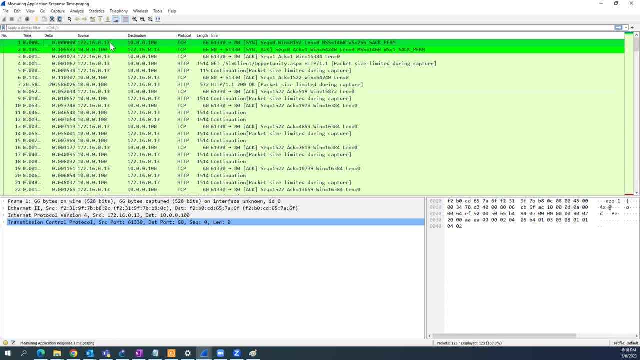 okay, so the video is here. if you can see the chat box, you can see that there are two webpages here. first packet: we know this is a sin i send a sin packet from because this is a client. from the port number: i know this is a client, random port number and 80. this is for http. 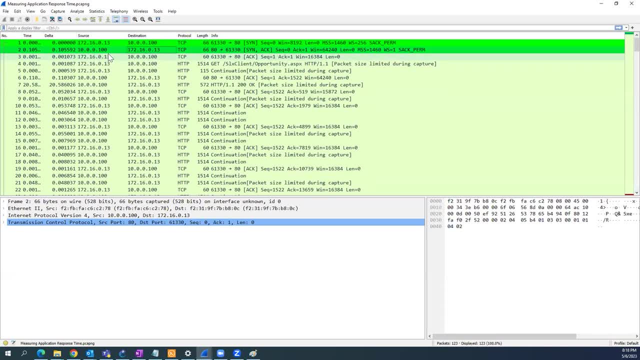 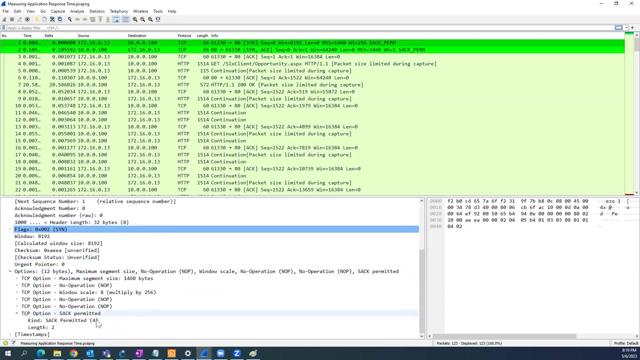 and i get a snack from the server. the server is 10 0 0 100. i get a snack and if you look at this, both allows the sac selective acknowledgement. so here you can see that and even the tcp options. you can see the selective acknowledgement. it should be permitted on both end. 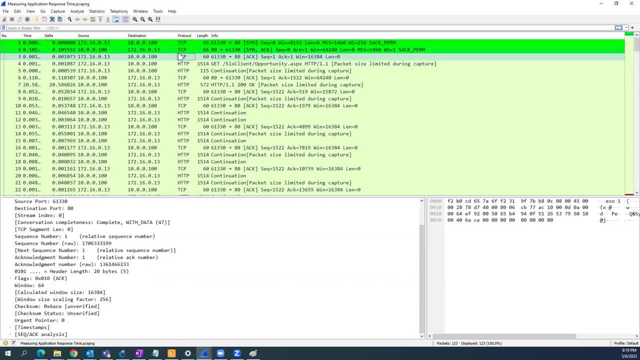 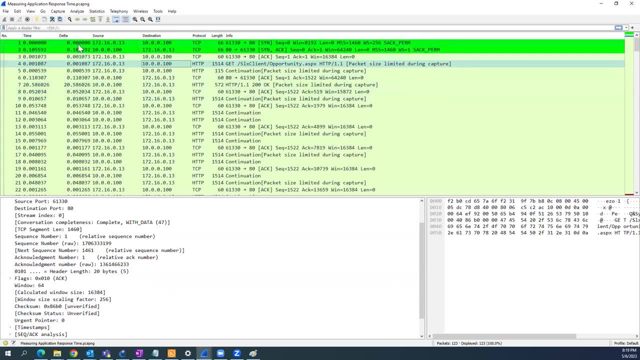 so now my connection establishment happened successfully and the client sends a get request. but before that, when you look at this, this starts with the delta time starts with zero milliseconds and then for my sims snack it takes 105 milliseconds. so this is my initial round trip time. 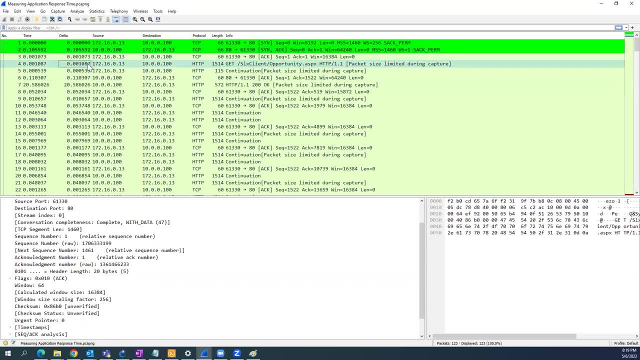 and if you actually see this, i send a get request, http get request, and it continues and the server sends an acknowledgement back, then it continues. and if you exactly spot here for this, http 200. okay, this is from the server. it took about 20 millisecond here. sorry, 20 seconds. 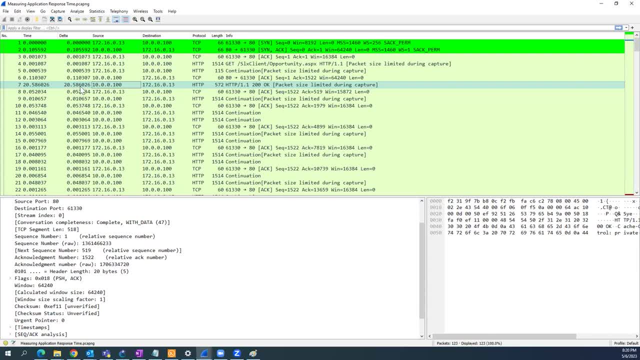 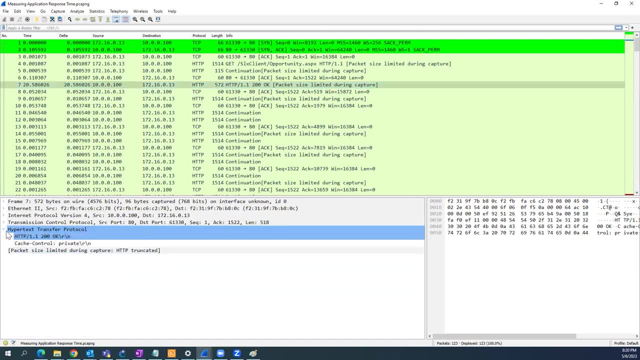 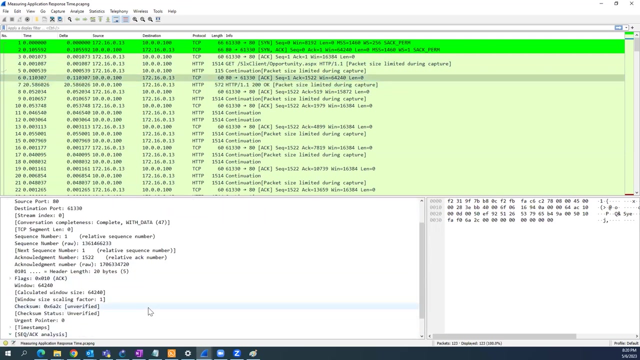 so all the values beyond this period is millisecond. so here it takes 20 milliseconds. but if you look at the initial round trip time, so for example, if i take this tcp and if you have to go to sequence and acknowledgement analysis and if you see the initial round trip time it says is 106 milliseconds- here for my tcp connection- 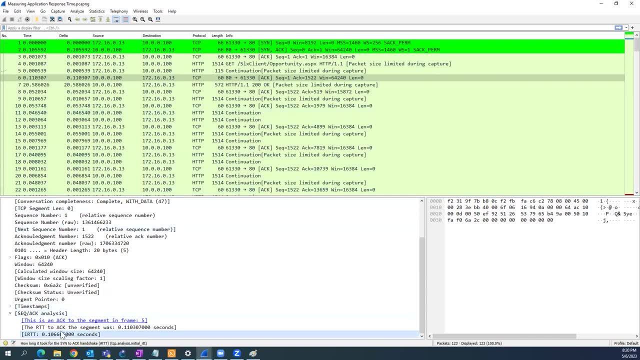 so it means that i i don't see the jump in the tcp. so i'm going to go to my tcp connection, but whereas for the http i see a jump of 20 milliseconds. so who's doing that? so i send the http get request, but after 20 seconds the server is actually sending a replay back. 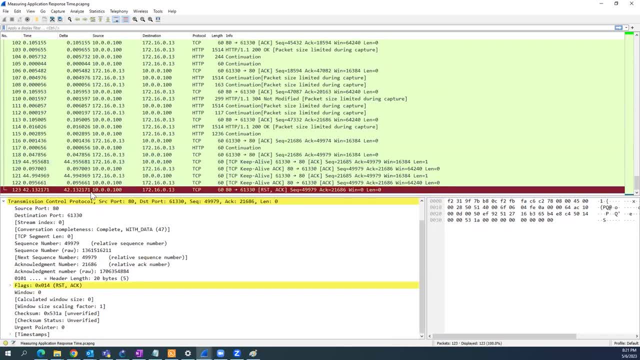 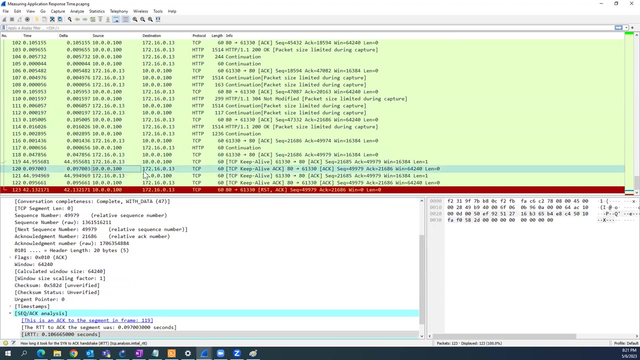 and if you scroll down the server is doing a reset so it might be a busy with some other communication and it is not ready spawn at this point of time. and if you see there is a lot of tcp keep alive. so this is a client and the client keeps sending the tcp. keep alive and for that the server is sending your tcp keep. 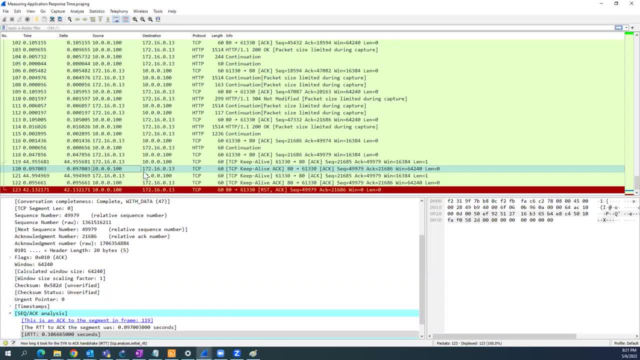 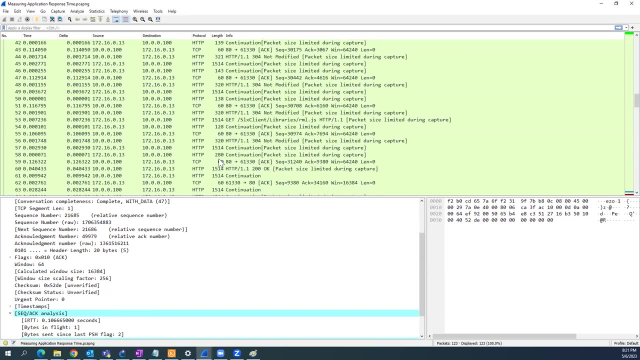 alive back. so it is something like the tcp connection should be opened. it says that my tcp connection is active, but it takes 44 milliseconds for a client to send a reply back again. so here the problem is the server is busy server and the application has a slowness. so what are 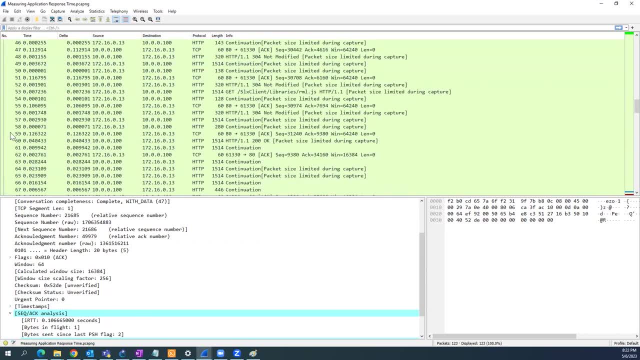 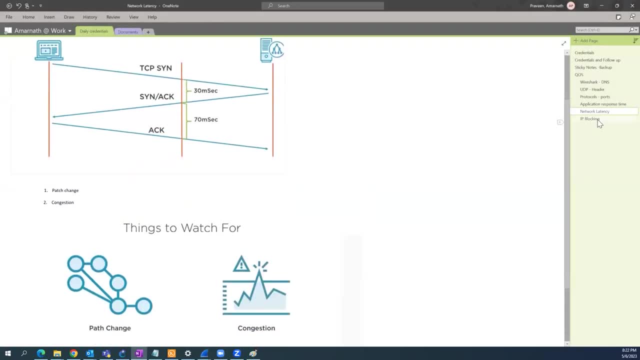 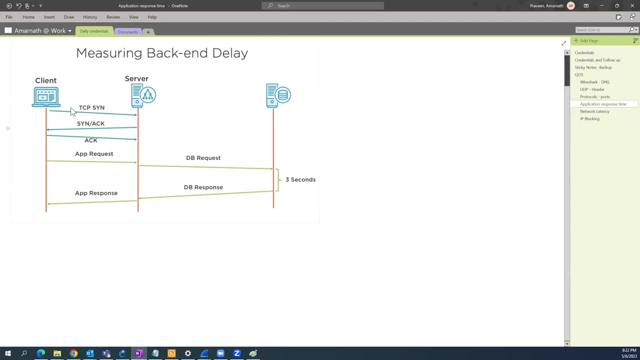 the other key things when you have to consider, for when you reach out to your application team. so what are the key things? you should ask them. so if you look at this, the key parameter is: you should ask them: what is the time taken for my tcp, syn and syn act, but whereas for my application request and 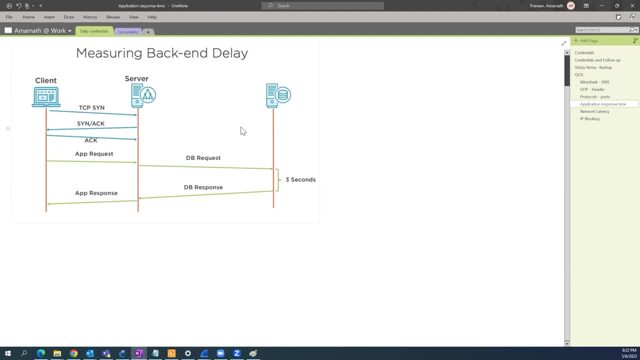 application response. i see a jump of 20 milliseconds and also i have to check: is it the server is connected to the back-end db server or any kind of server, or is it as some kind of a load balancer, you're trying to establish a connection and the back-end services that's running on the back-end? 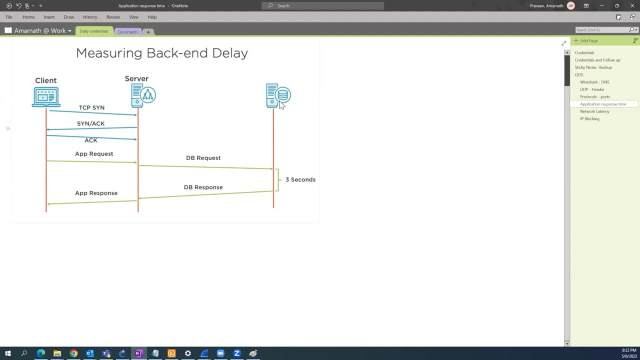 server from the load balancer whip to the back-end servers. so if you have calculated my initial round trip time, what is the time taken for my tcp syn and syn act? it establishes another tcp connection. is it a problem there? so you have to do a capture even in. 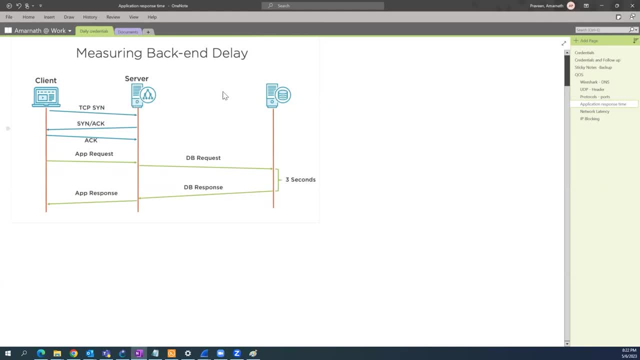 the middle and you have to calculate: is it from my server to the back-end server? what is my round trip time and what is my application response time. so we have to look at all from all the angle, from from every angle. you have to look into it and you have to do a capture. 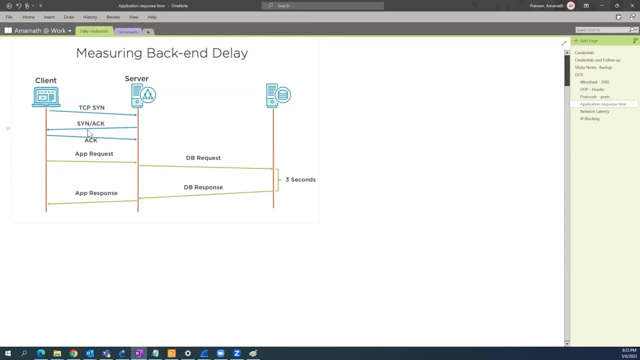 but the key thing is you have to differentiate. what is the difference between the tcp round trip time and the application round trip time? and also you have to look at what is the db connection it has, or it is a load balancer, is something connected in the middle and 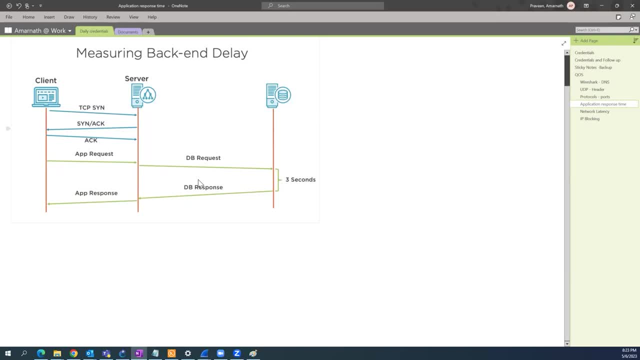 you have to do a bi-directional capture and you have to see where exactly the problem is. but the key thing is you have to the takeaways. you have to know the difference between what is the tcp round trip time and the application round trip time so you can figure out where the problem is. 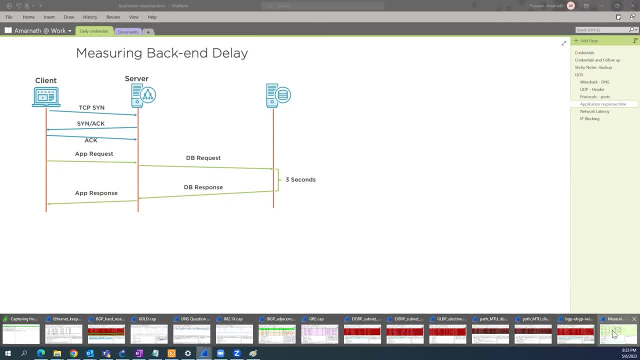 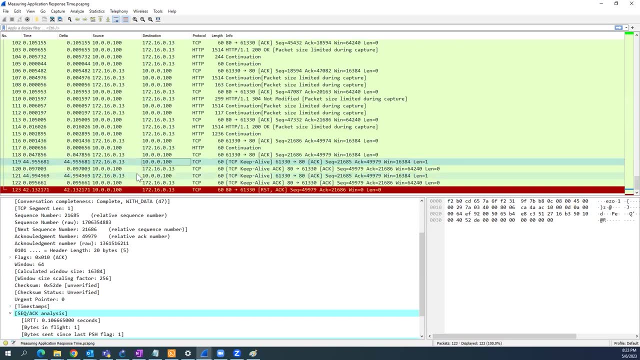 and if you have to go through some other options like, do i see a keep alive, tcp- keep alive. so if you look at this, the client is keep sending a tcp keep alive and i get a replay back after 44 seconds. it sends a keep alive, so it means that. 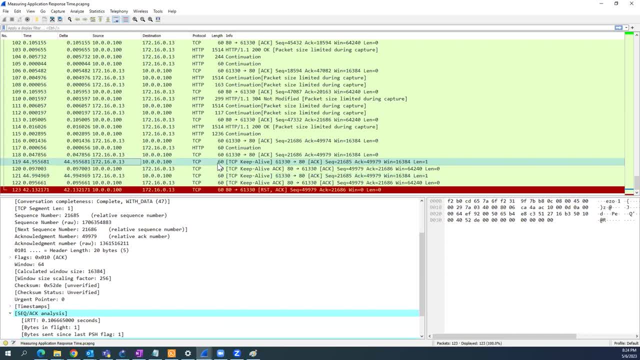 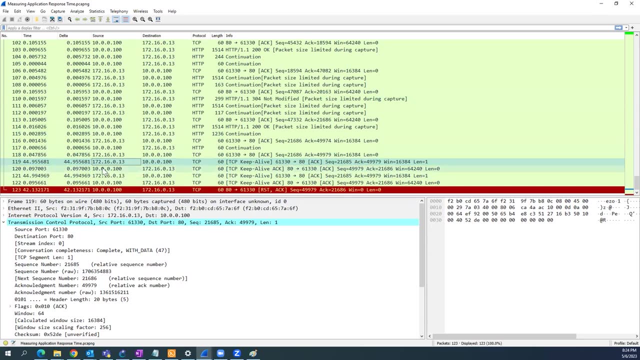 the server is not responding and also you can make use of your other fields, like your ttl, your acknowledgement fields, and you can make a comparison as well. but it's it's pretty evident that i keep sending your tcp- keep alive for the server, because i am not getting a response from the server and later on, at some point of time, the server is. 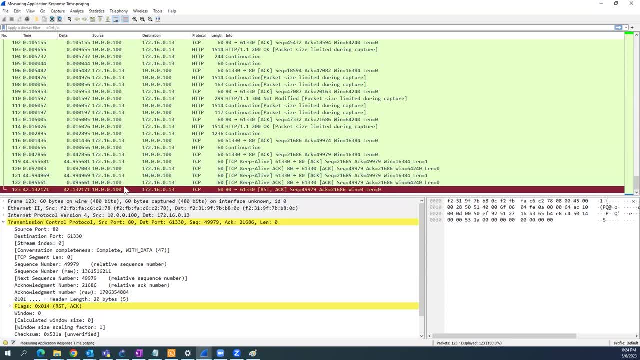 resetting my connection here. so there is something you have to look into this server first. is it a lot of reset happening for other clients or is it the reset happening only for my? my ip address, one seventy two sixteen zero dot one, three, or it is doing a lot of resets there and i i also 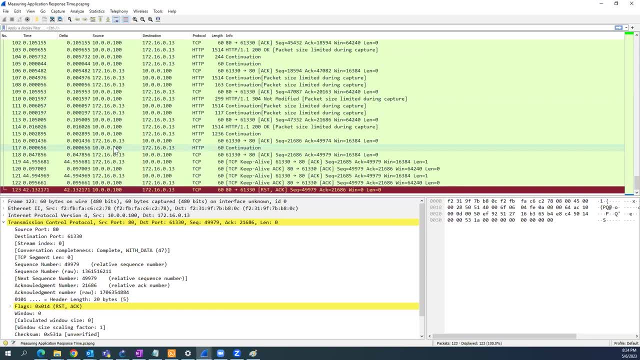 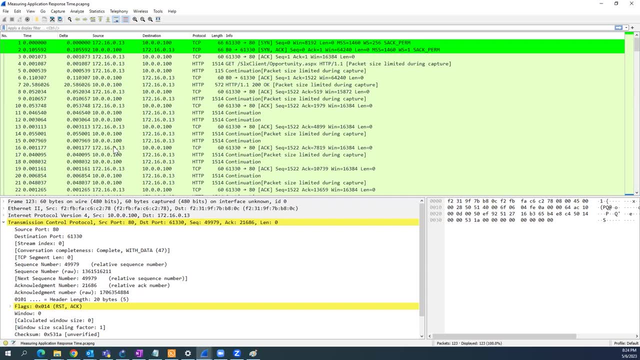 have to check. is it? a lot of keep alive is happening on the server end for other http connections as well, so this is the key thing you have to. you can find your application slowness with this logic. so let's do a normal capture and let's see what is the time taken for it. 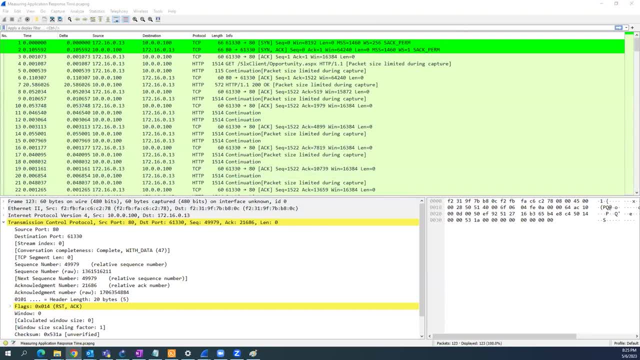 so for that, let me open up the server. just give me a moment. i mean, have some problem connecting to this server, but yeah, it may be a lot, but i'll let it be, because the server is fairly large and all the other data are still on the server, which is great. so let's take a look at the 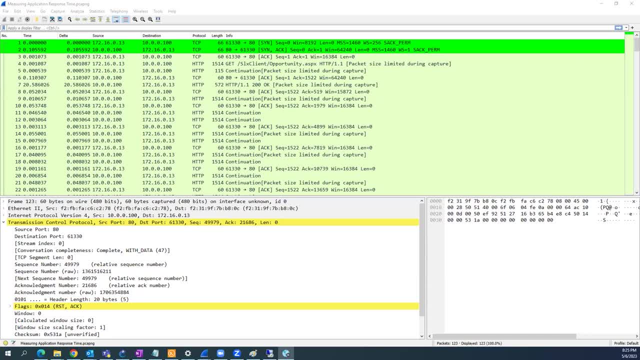 server. now that's. that's pretty great. so first of all let me just do a great power drop and then i will take a look here at my mobile device. can you see where i have my camera camera on my mobile device? it is on there. let me can go ahead and let me do that and 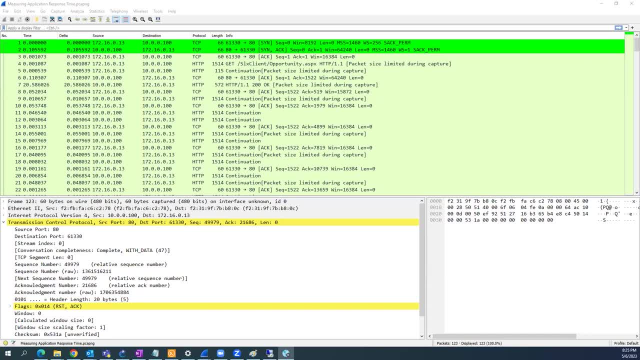 we can also set up the app. so let's go ahead in the app. there we go. i'll go ahead and check out the app and we can see that it is the app that is running on the server and on the server here you can also see, you can see that there is a power drop over there. 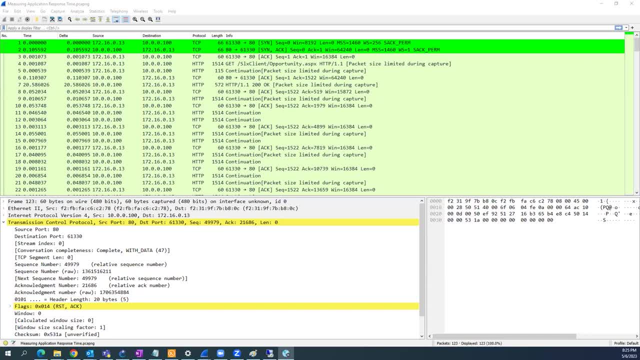 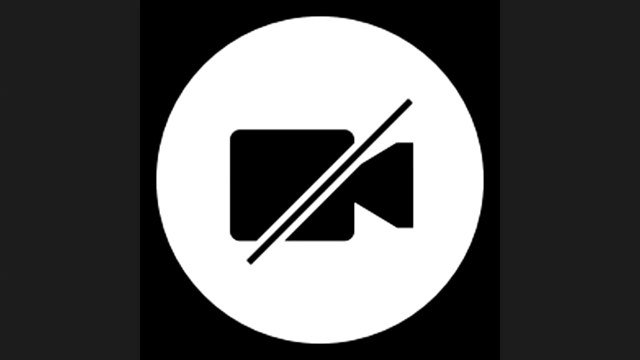 you just need to double click on it. that's all you have to do. that's all you need to do is to check out. as you can see, you, you Just give me a minute, guys- You, You, You, Yep. so if I do a DNS matches Google, so I'm going to see my DNS request here. 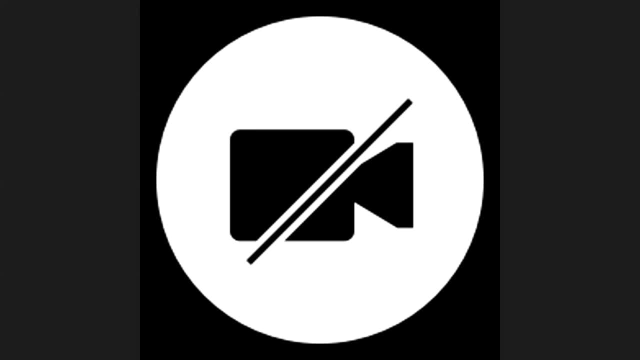 You. So this is my first request here, so I want to find the IP address. Okay, One minute, actually we have some problems. Okay, so I'm going to see my DNS request here. so I'm going to see my DNS request here. so I want to find the IP address. 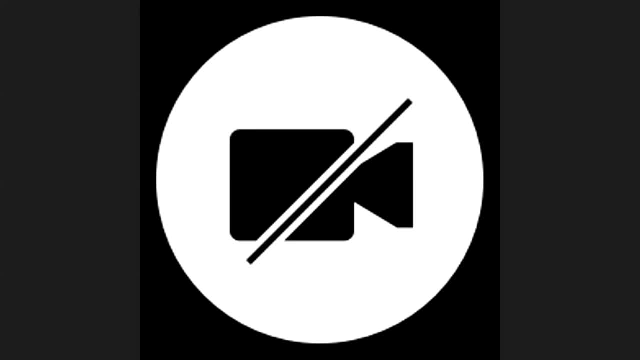 Okay, so I'm going to see my DNS request here. so I'm going to see my DNS request here. so I want to find the IP address. Hello, Hi, Gilbon, can you hear me? Hello, Hello Arjun, yes, I can hear you. 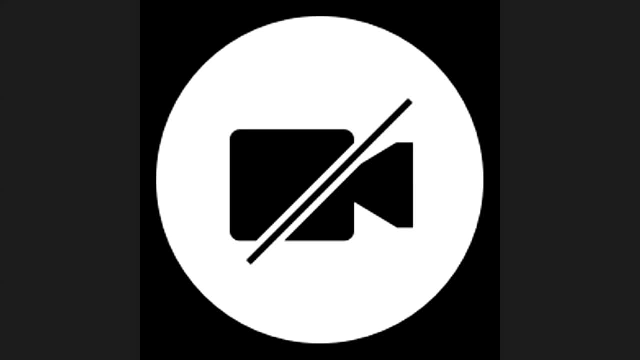 Hello, I don't know, for some reason you became a host. Can you make me a host? Yeah, Oh, I don't know how that happened. Just bear with me. Sorry, No problem. yeah, Okay, I'll tell them. Yeah, thank you, Yeah, Ok順. 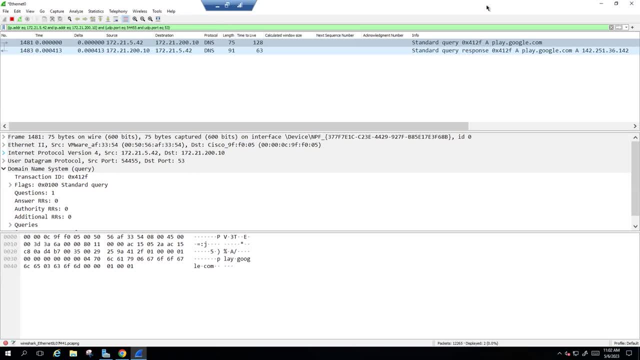 So I think everybody can see my screen right. Yeah, Yeah, Yeah, answer You. I can see you Right, Right, So, Just So. So if you see this DNS queries, I want to find the IP address of googlecom. So, if you see this DNS queries, I want to find the IP address of googlecom. 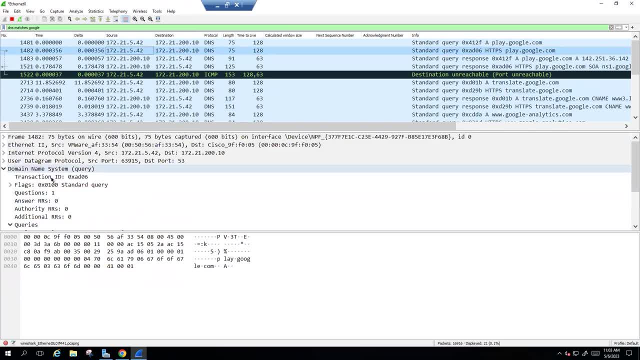 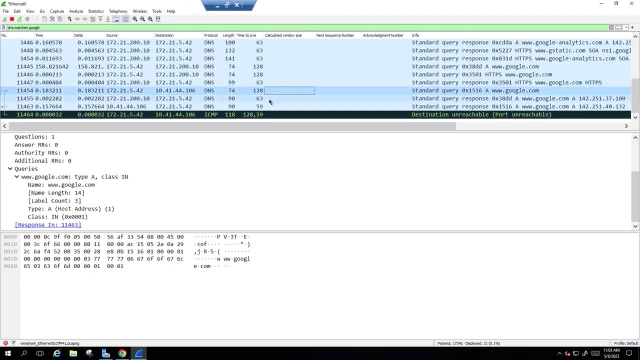 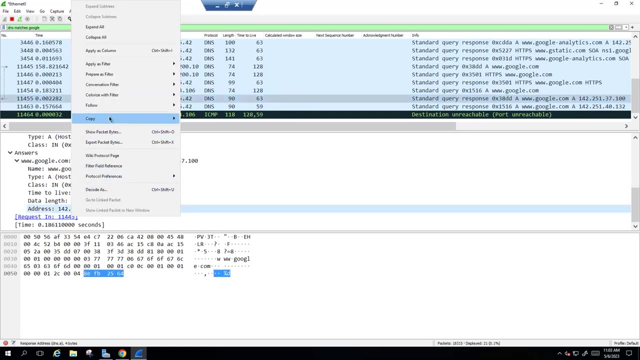 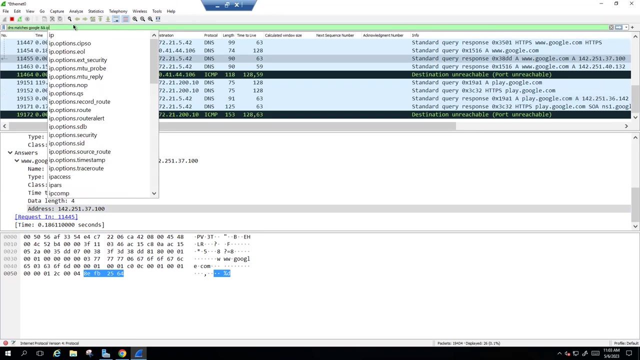 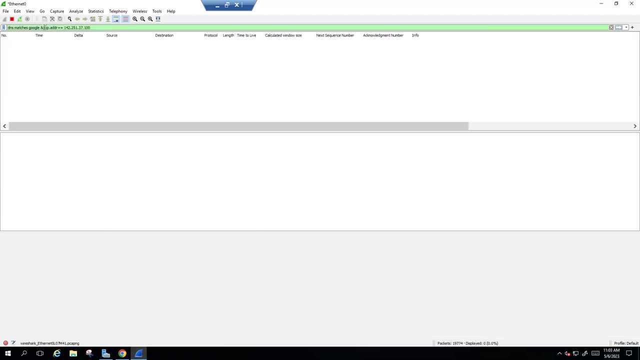 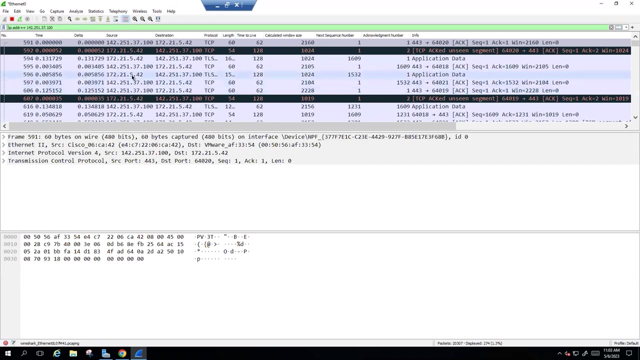 So if you see this DNS queries, I want to find the IP address of googlecom. So for googlecom, I got a way record here, So I got an answer here, So I'll copy this as a value IP dot address. So I'm going to filter only the IP address of googlecom. 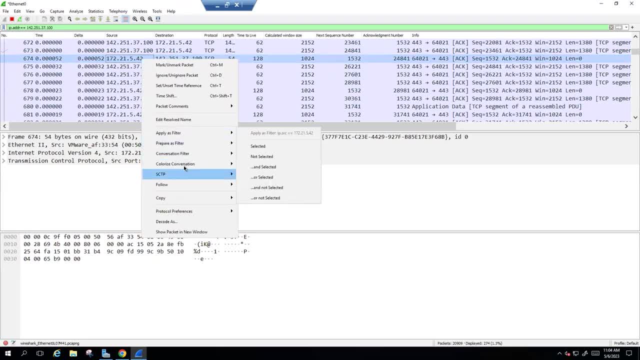 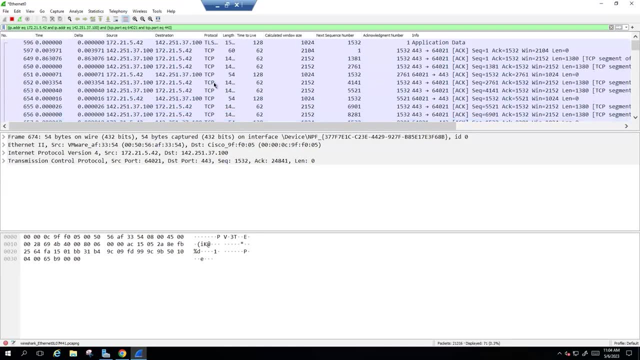 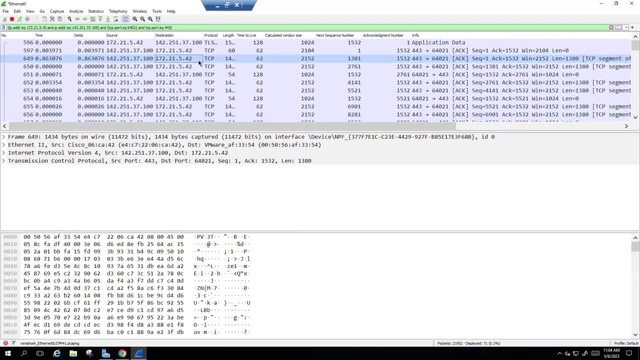 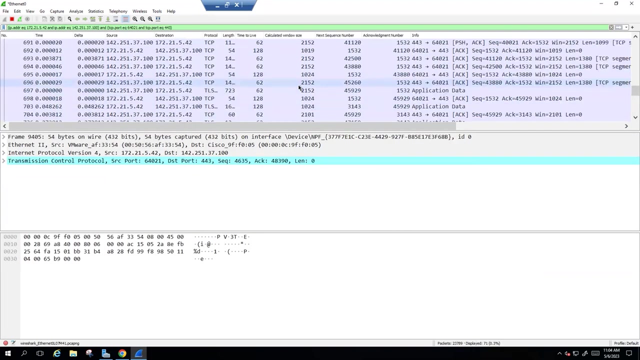 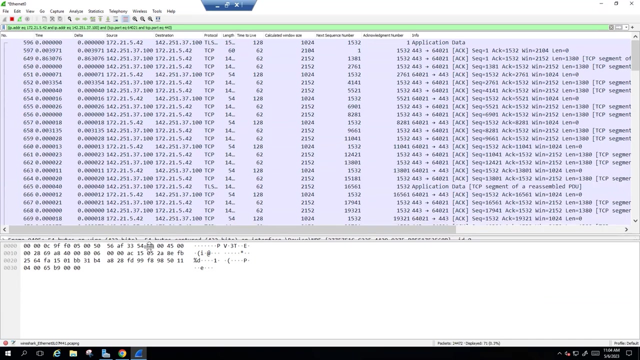 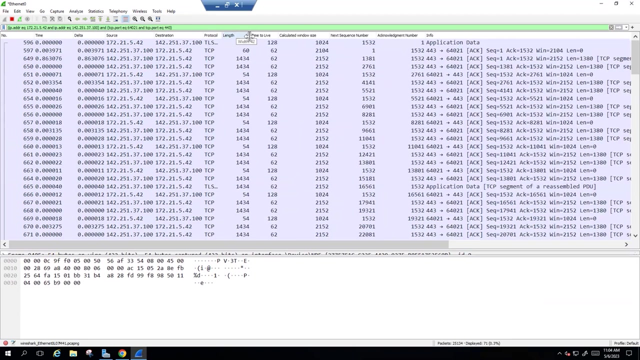 If I go to any conversation, So if I go to conversation filter and TCP. So if I go to any conversation filter and TCP, Go to your conversation filter, TCP. Check this. So it is broken somewhere in the middle. So it is broken somewhere in the middle. 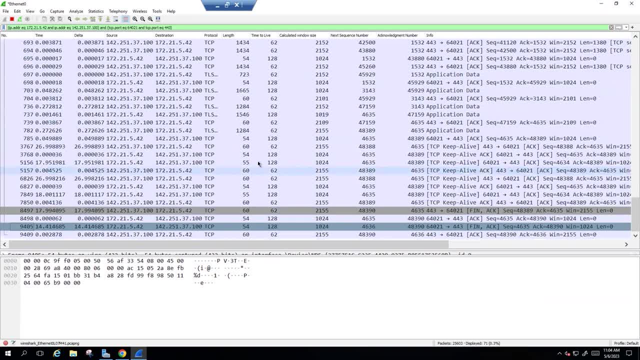 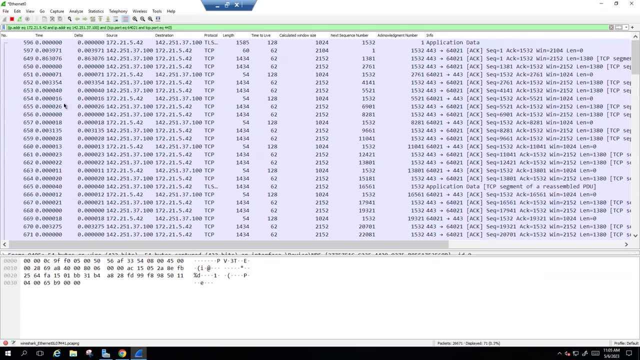 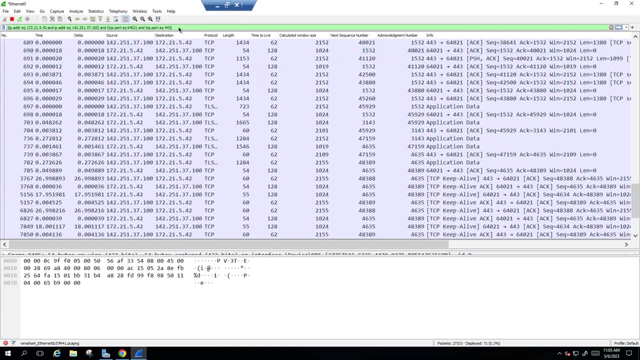 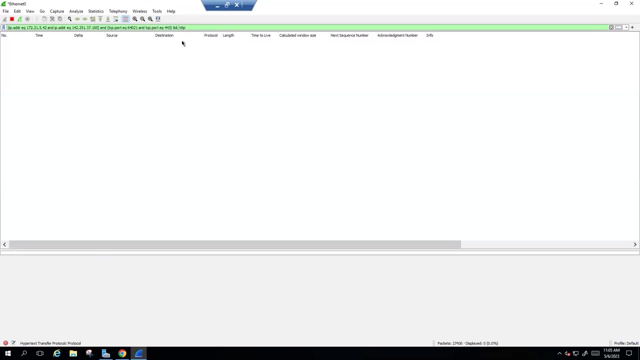 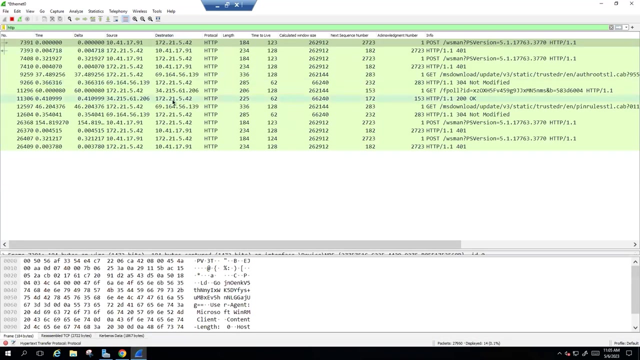 I calculated my-knowledgement, My calculated window size, my-knowledgement. Ok, from here, if you look at this for your HTTP, Let's take and write a new. So no HTTP connection happened for the source and destination, So this is my device. 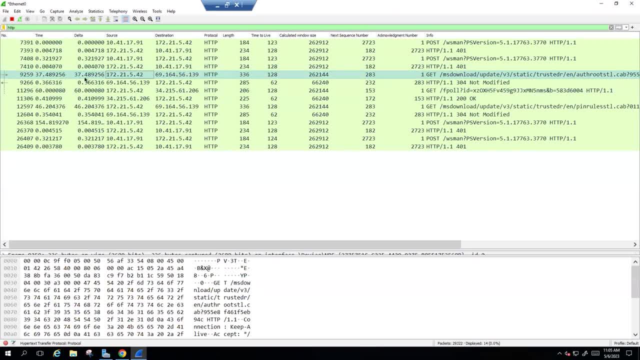 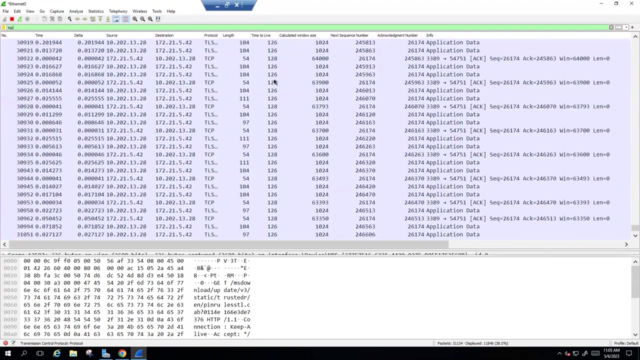 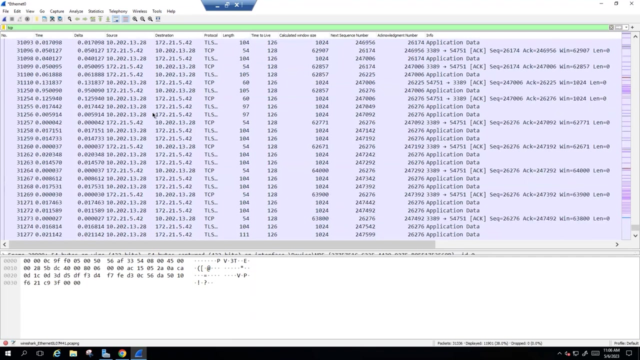 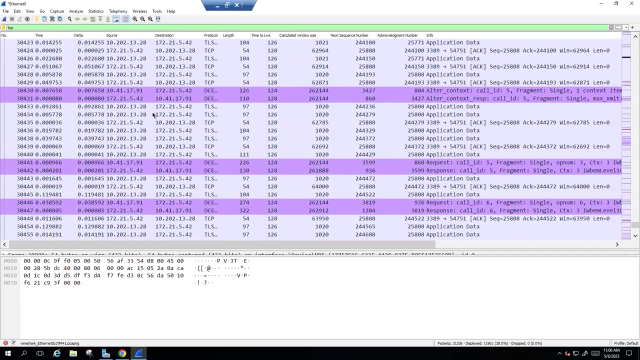 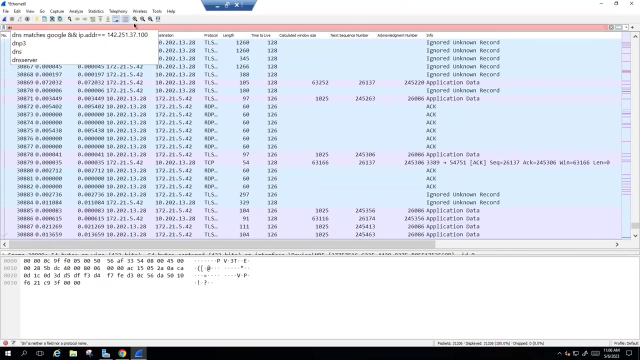 So it has taken 37 seconds for a get request And if you look at this, all my device, it's taking 46 milliseconds, And if you compare the value with TCP and if I stop the capture, So this is the IP address. 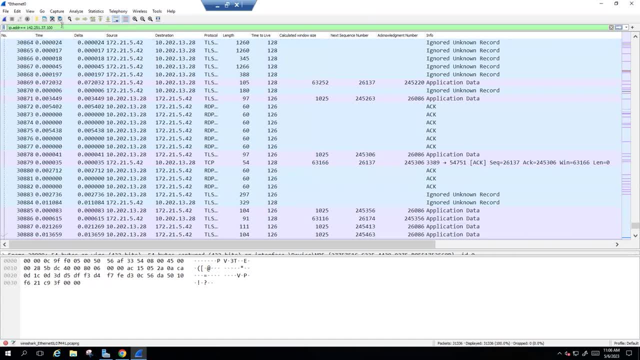 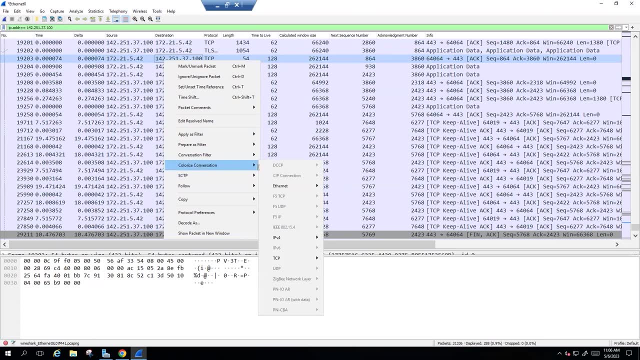 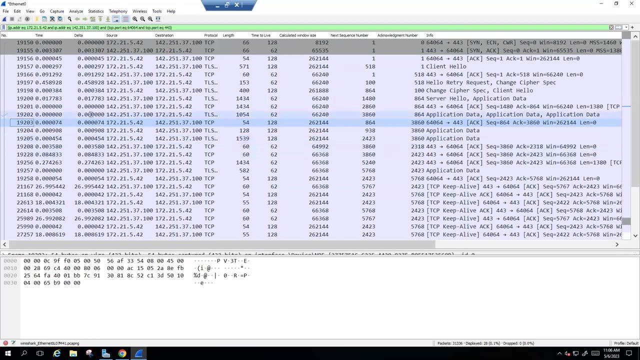 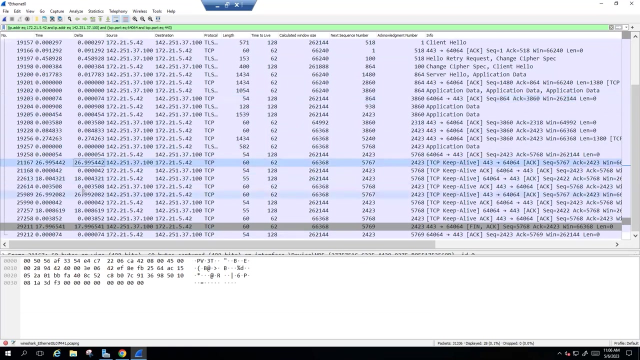 So let's check for only TCP. So if I go to conversation filter- TCP, if you scroll down here I can see for the TCP it goes from 20, 26 millisecond, 18 milliseconds, 17 milliseconds and 18 milliseconds. 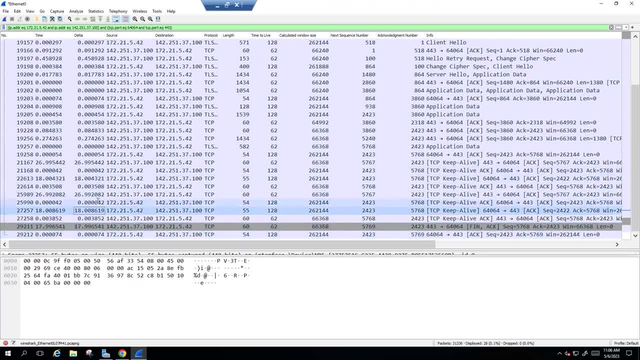 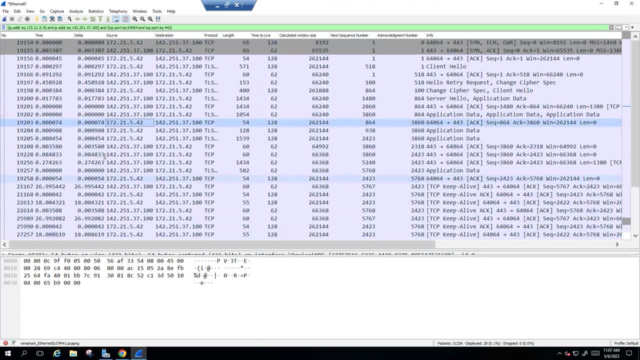 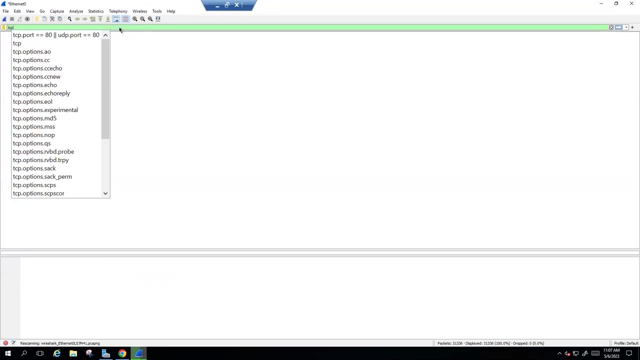 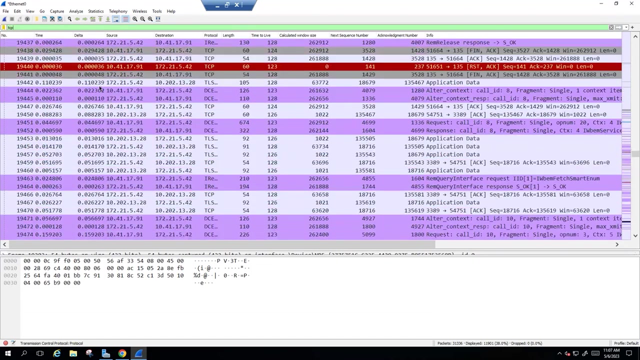 So it means that definitely I have some slow connection here. So how to find who is doing the slowness? If you look at the other TCP conversation, if you give common as a TCP, if you look at all my TCP connections, I don't see a biggest jump here. 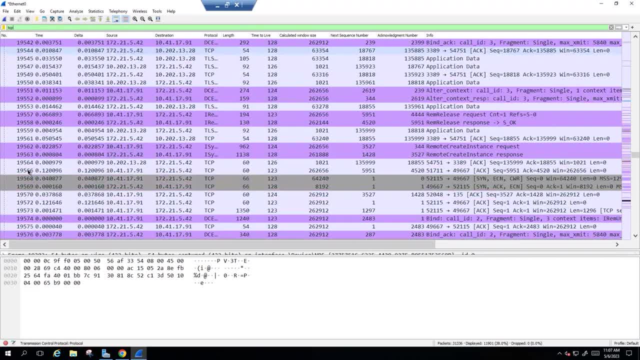 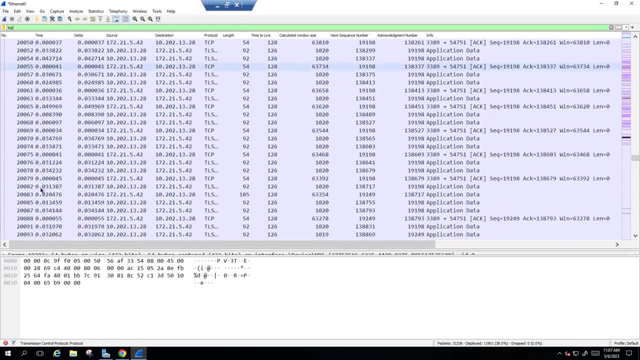 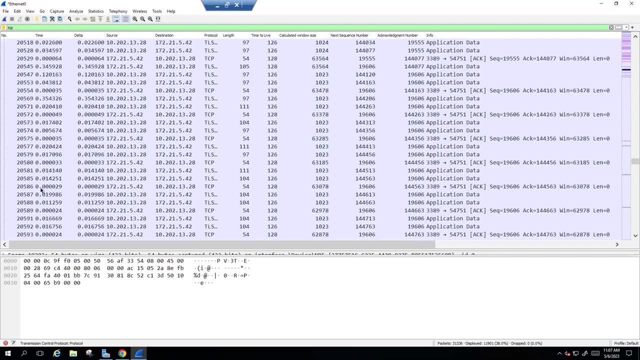 If you look at your Delta time value and my time value, it's not showing anything abnormal, or it's not the I mean the time taken is not jumping even for a second here. but for that specific conversation, my Delta time has been increased to 17,. 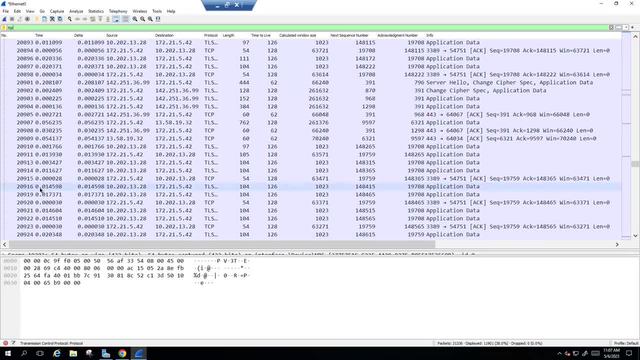 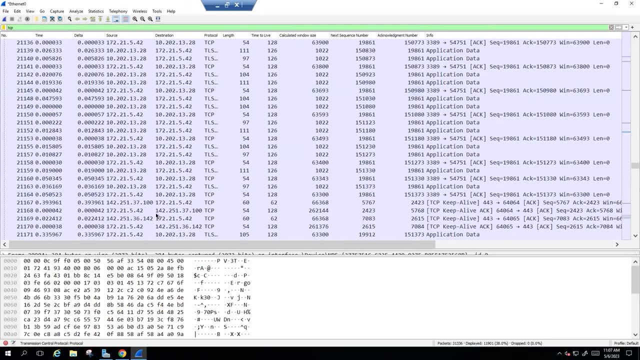 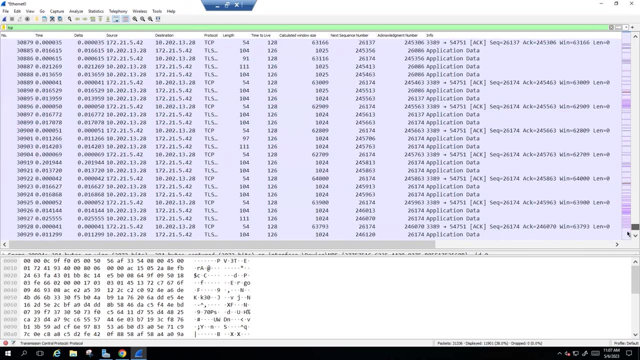 40 milliseconds. Okay, So it means that. so when I establish a connection, HTTP is HTTP collection. I see a slowness. but whereas for other TCP connection, if you look for other IP details here- one leaf TCP- I don't see anything here. 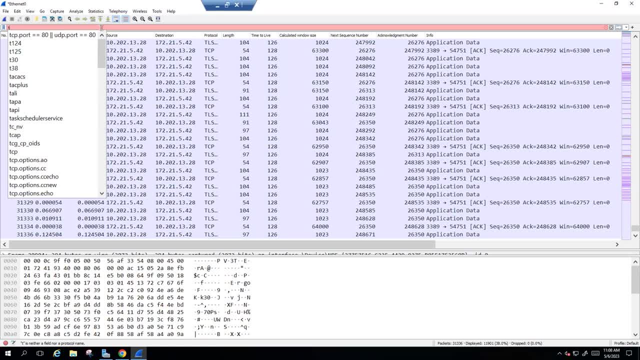 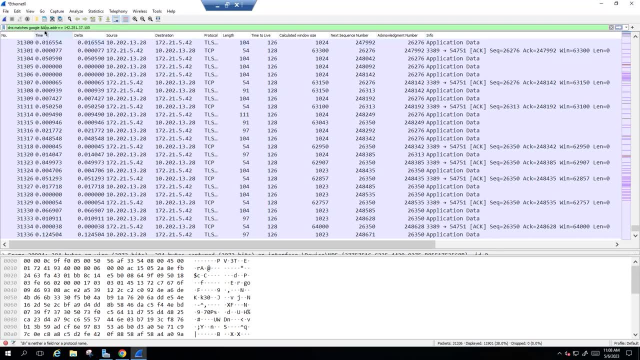 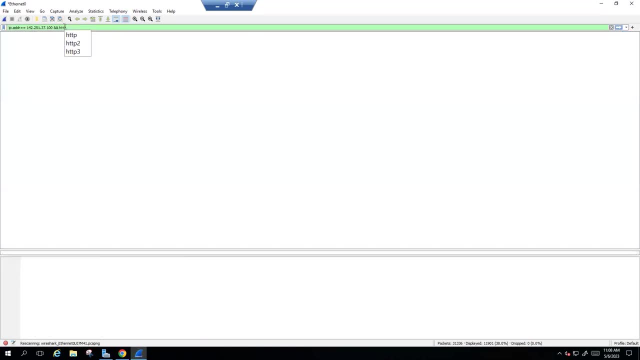 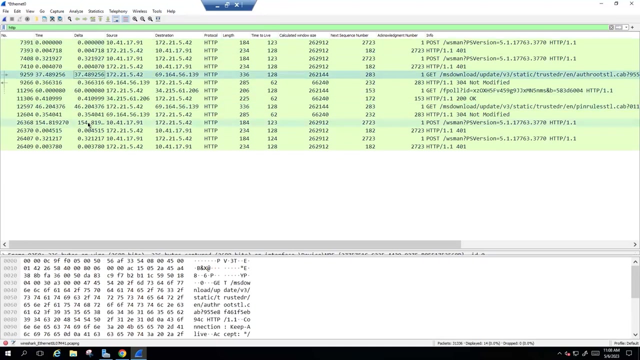 but if you look at the this particular, this particular IP address and HTTP, if you look at the HTTP request, I see a lot of latency for my HTTP requests If we go over here to the relevant IP address. and if you look at this common public IP address, 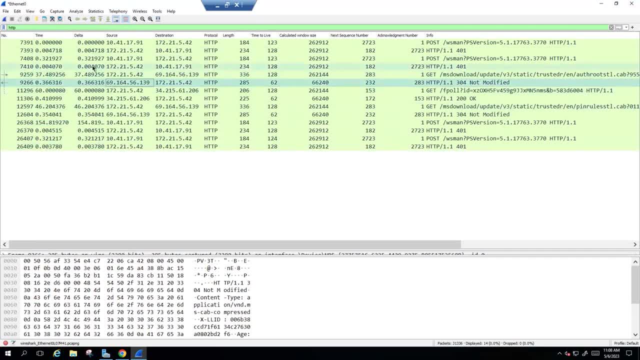 I don't see a big jump in the public IP address, but for the internal IP address. So for my PC it takes 46 milliseconds for me to do something. So it is something that I am doing, something. I am making a connection here. 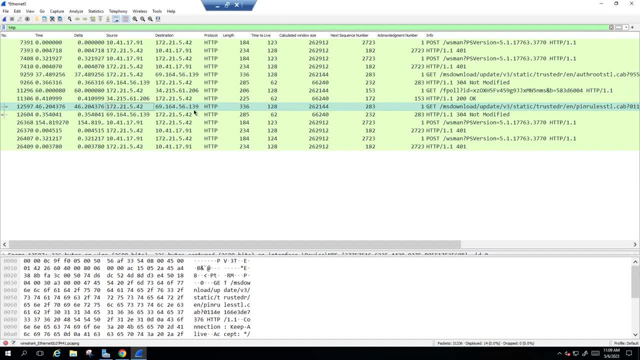 here i'm searching for the options here. i'm not doing a proper. you know i'm not very active with my http connection. that could be one problem and other problem would be really if it is a server and if you clicked on something and if the user is not doing anything and if user is active. but 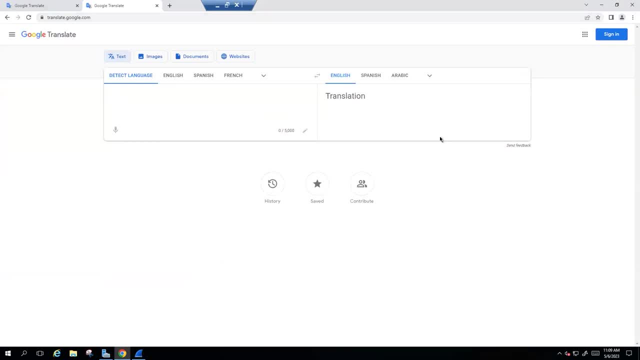 the server is not responsive and if the server is busy then you will definitely see the slowness. so this is just to find how we can compare the- you know the round trip time for http as well as for the http. so from here you have to figure out, like the same way you have to figure. 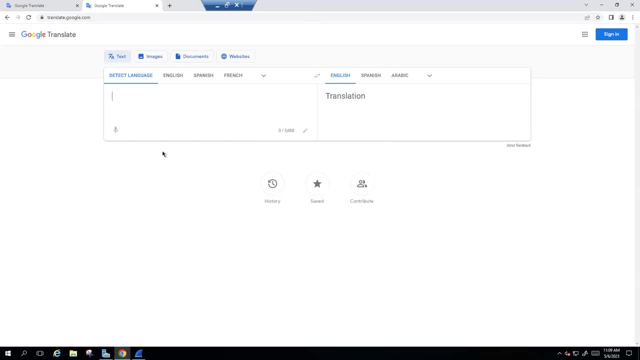 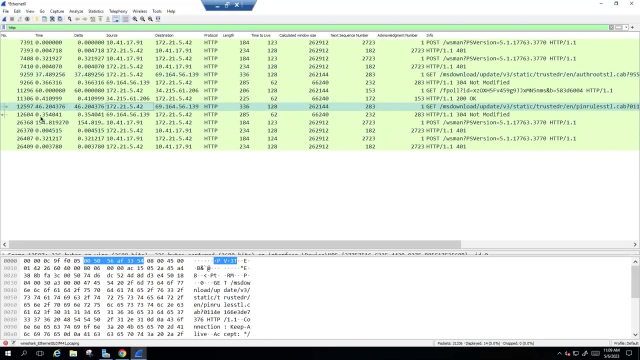 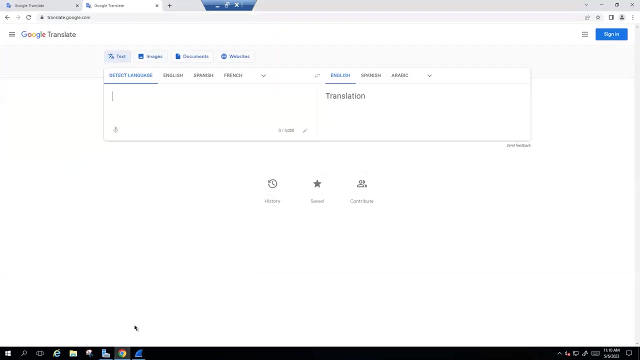 out for other issues. so you have to replicate and you have to go through step by step and you will get to know about that. so the main key thing is how we are going to differentiate the round trip time for http and tcp. so now let's see uh use case for bgp. so i'll give a little bit background about bgp for the same. 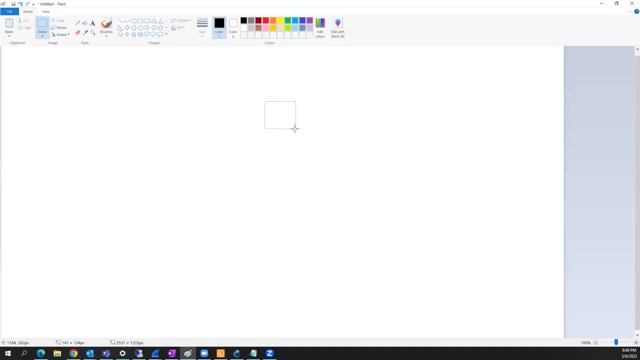 thing here. so this is a sort of a Thank you. So there are two different protocols. we all know about this. This we know. I mean, the routing protocols is used to exchange the routing information And there are two classification: one is IGP, one is EGP. 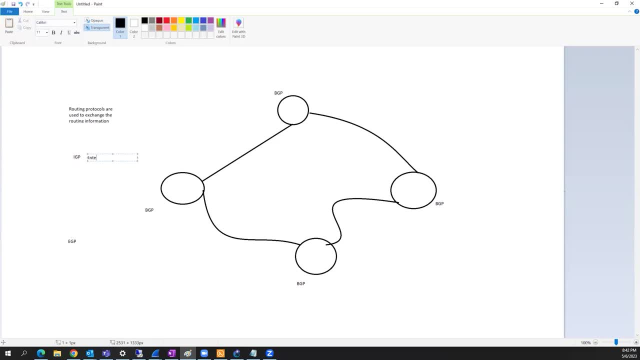 IGP stands for for interior gateway protocol. EGP stands for exterior gateway protocol, So why we are talking about all this? So I just want to give a background about that. So IGP, that's further classified into all your EIGRP. 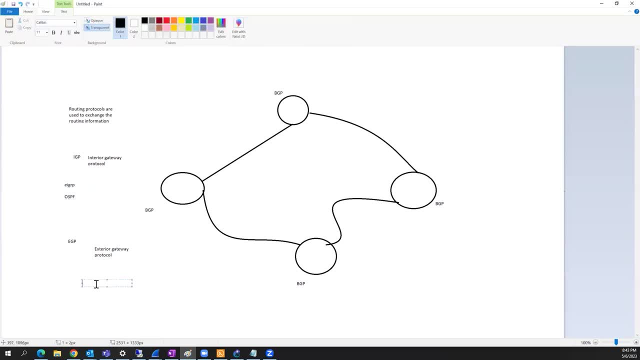 The most commonly used, and OSPF. And for EGP there's only one protocol, BGP, and that is most commonly used. So I think the ISI falls in the category of BGP, but here we are just talking about BGP. 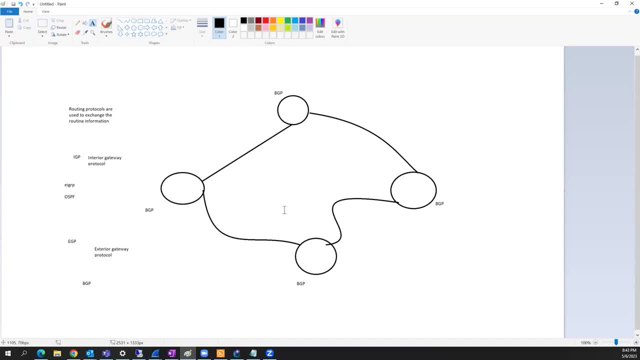 So what is the interior gateway protocol? Okay, so this is my network, This is my autonomous system. I mean, this is your company and you have your own, you know- WAN connections. So you are managing this WAN and this is IGP. 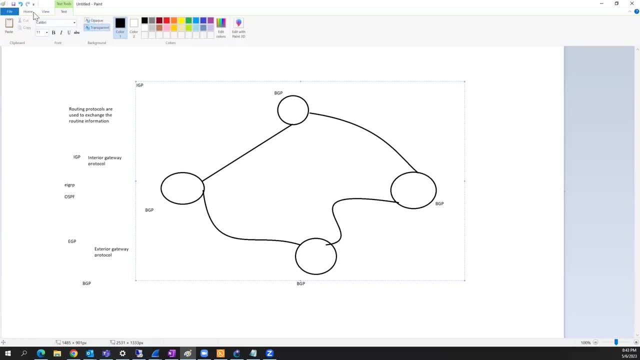 And BGP is further classified into two categories: IBGP and EBGP. So by design, so if you are using, if you are using an IBGP, it should be mostly the use for the core switch and the hidden router peering. 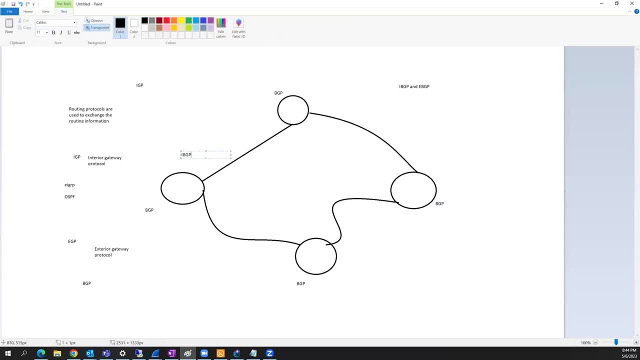 For that we use IBGP, So this IBGP routes cannot be routed externally, So that all stays within your network. It's currently being mastered for a different goal And now you can cut this out vanillaishly. Thank you. 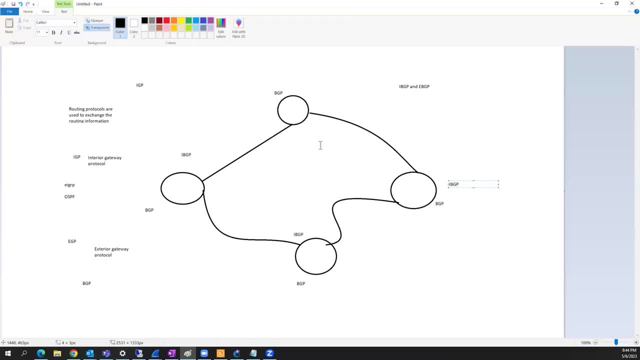 Don't worry, that was English, that was thoroughly radishized. So only your hidden router and your ISP. they both will be talking and exchanging routes on EBGP. So remember that when your ISP runs directly into your IP, you can control the usage of that, not just throughusiovware. 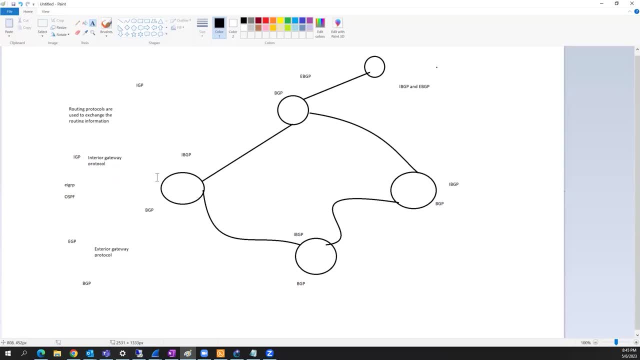 Yes, now I use IBGP as well, ibgp's interior gateway protocol. so most of them they use eagrp or ospf. this is the most familiar and most commonly used routing protocols and the bgp why we are talking about bgp, bgp, that. 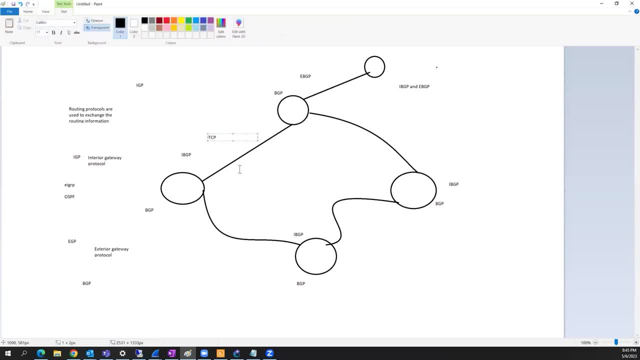 pure sleep. it purely work on tcp if this particular router, if this both router, has to establish a connection, so it has to send a sin. for the sin i have to get a synapt back and then again the source will send a acknowledgement back for the tcp synapt. 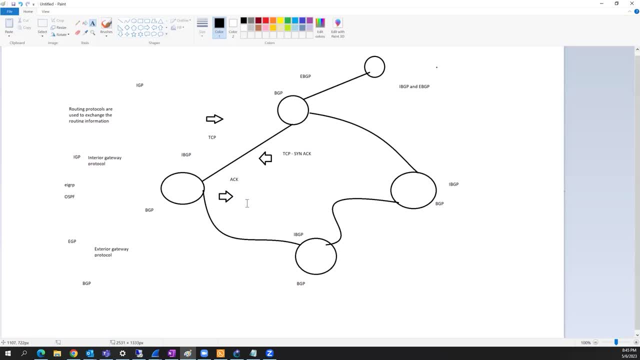 so once this tcp connection establishment happens in the bgp updates it will share the nlri information, that is, network layer reachability information. so for this device, the network example i, i own a network 10 000 and i own a 20 000. so in a bgp update 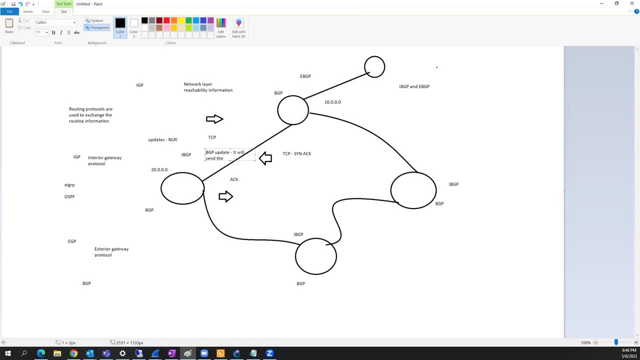 it will send the network layer reachability information the same way. here it will see share its network layer reachability information. it is that so it shares the network information. along with that inside the network layer reachability information you will see the subnet mask, the ace number. 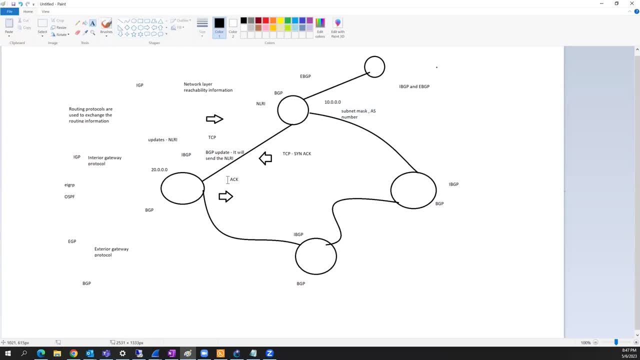 so i'll be in exchange. so why we are talking about all this? so if you know about all this and if you, if you peel out the you know capture and wire shark, and if you see, is there anything- the subnet mismatch- that is stopping your connection, or is it something? 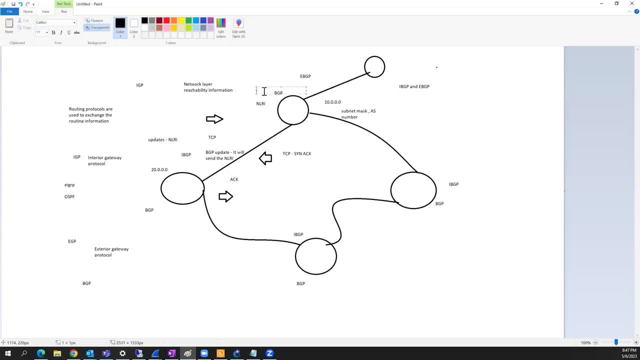 there are some here, particular acl. they have applied to tcp sin if they are blocking the tcp sin, so you cannot establish a connection. so both side the tcps, both three, three flags has to be open, since you can act only then, the if the connection establishment happens, after which your bgp updates with all your nlra information. 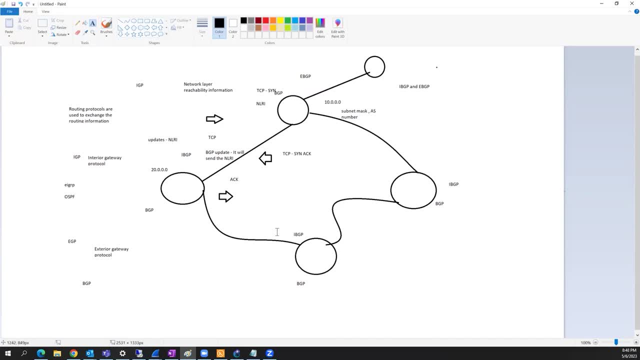 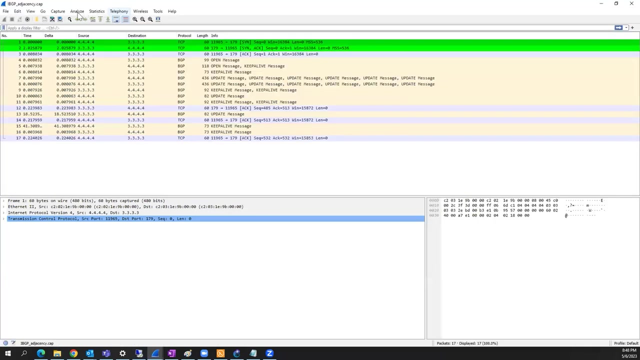 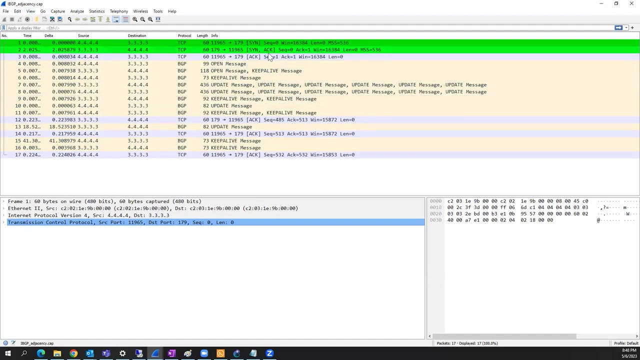 everything will be exchanged and now let's see how wireshark is going to interpret all those values in our active capture. i'll show that first and we'll do a lab followed by that obi's DType. so if you look at this very first packet, the source is ending is a sin. for that sin i have to. get a cynac and then for the synapses you will need to come to the problem pool, so this will go there. only the link check. this link will take you to the link to the synapses. if this normally either into a boring transaction, the link pitch is good: has easily 이거는 ayorsun rather than. add another link, coin trading, moneteering between all of threeren and then also seriously bring four pairs of exchanges or so. if you look at this, it's the same in tab. it should be trapped this uh block area. so if you have access to the value源 or the cultural organization, takes aos or 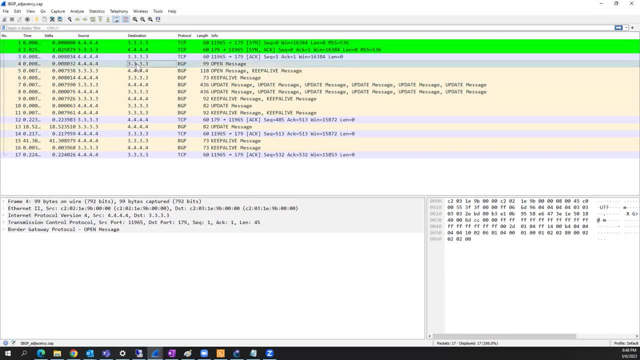 synag, it acknowledges it back. then it sends a bgp open message and if you drill down the open message, if you can see the bgp open message type and you can see the autonomous system number and you can see the bgp identifier, the ip address of the source. 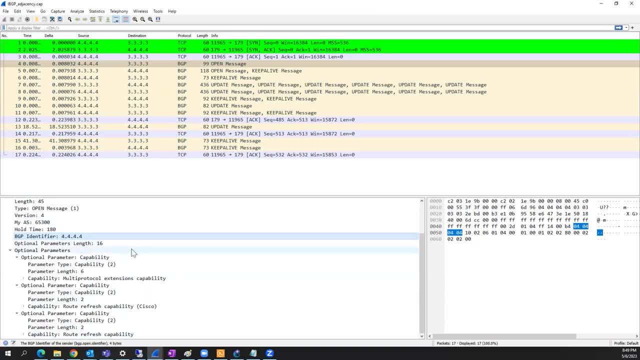 and it also talks about the capability of route refresh. we'll talk about that later, but it it shares all this information and along with that inside the bgp it has all the. it has the capability to share all these parameter details here. so i get a reply. message from 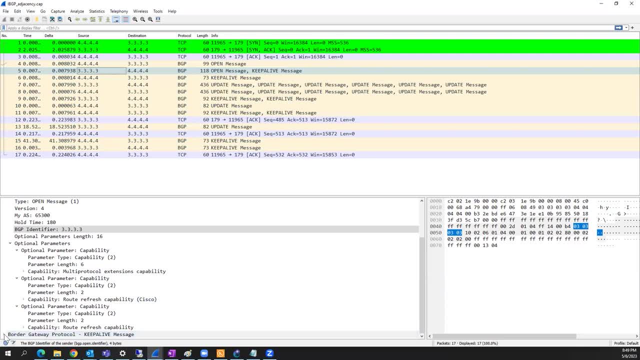 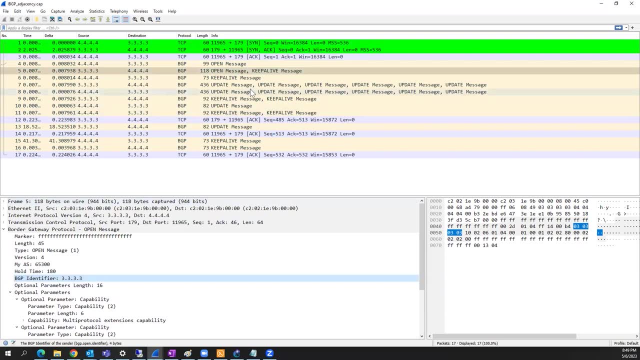 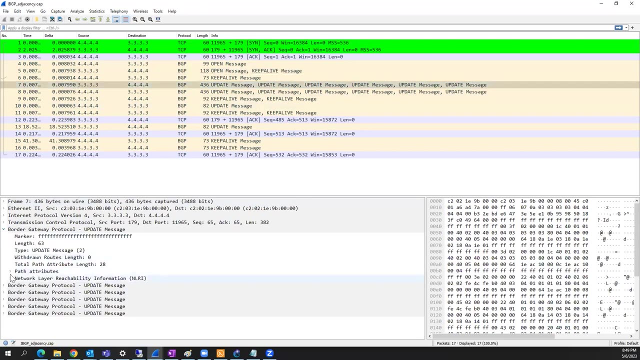 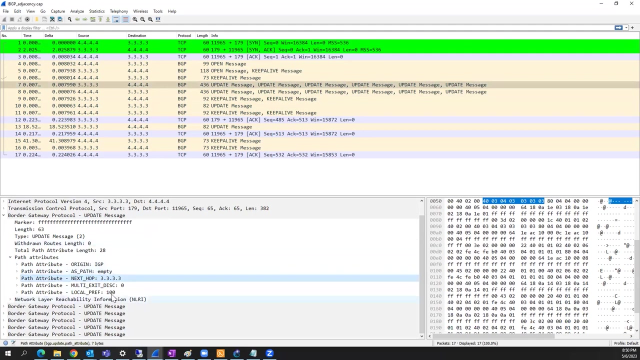 an open message: keep alive. so it means that my tcp connection is still active and this is the actual update message from the remote destination. and if you look at the path attributes, it says igp. and if you look at this, this says it's a next hop. this is my next, next hop and along with that, the local preference value. it. 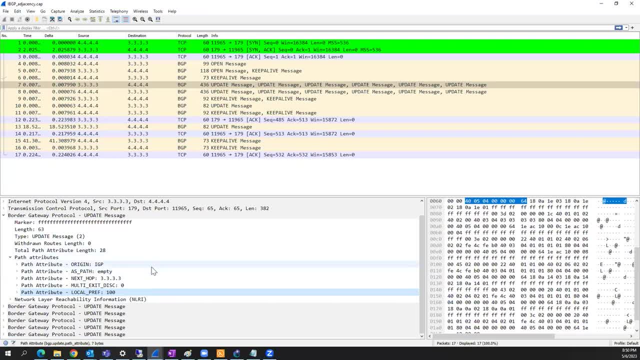 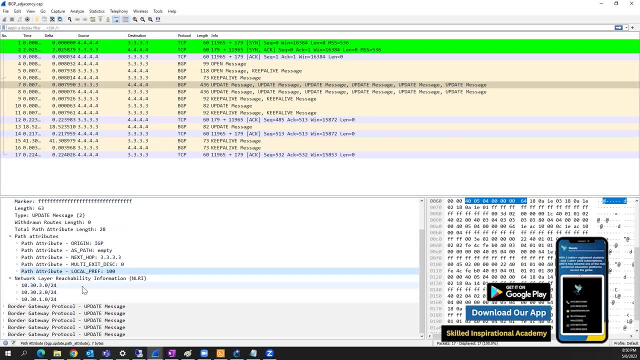 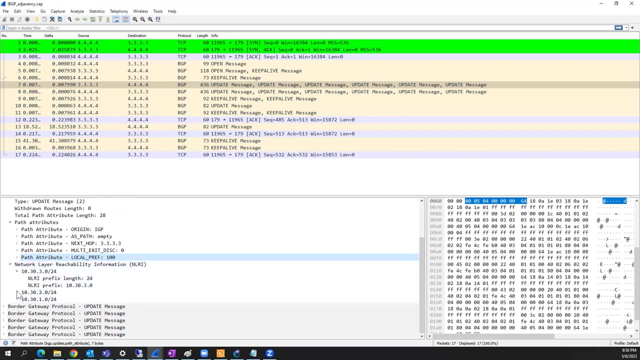 says the local preference will talk about what is local preference. but if you see, you can see all this attributes inside and along with that it we can see the network layer reachability information inside. so if you open it you can see what is the network address and what is the prefix length. 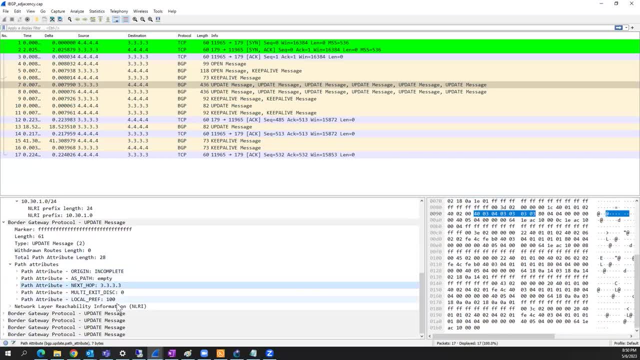 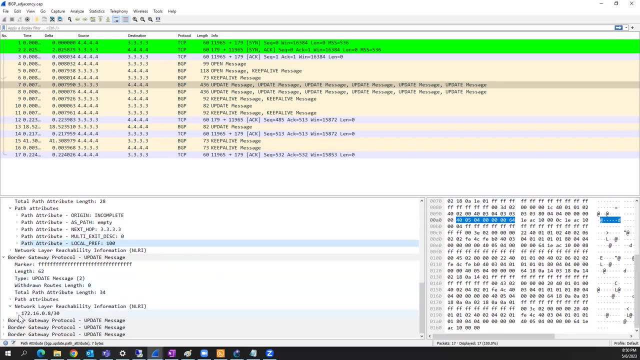 so you can see your next hop, your local preference value. you can differentiate both the nlra information. you can check: is it something your subnet mask is incorrect? you can go and verify it and then you can see the next hop. the next step is to verify the same. it will give you a bird's eye view of everything about. 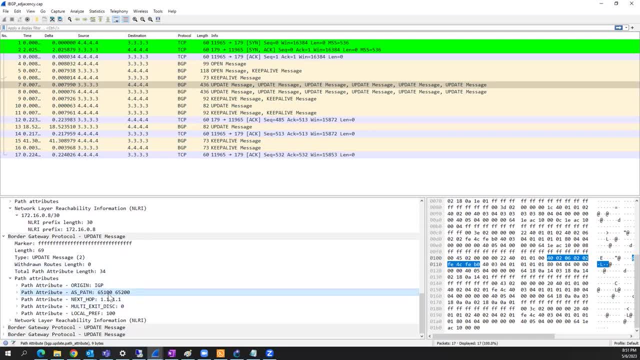 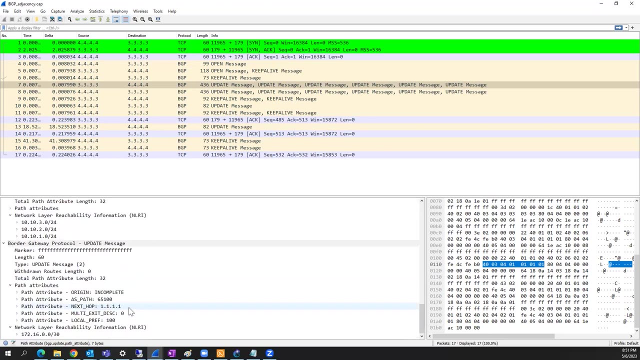 your bgp and you can see the as path. it says it takes six five one zero zero and six five two zero zero. so it says my next stop is one dot one, dot, one. and again i see bgp network reachability information path attributes. all this value is very useful to troubleshoot the issue. 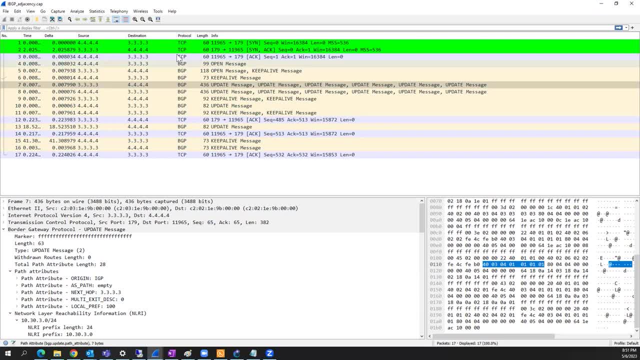 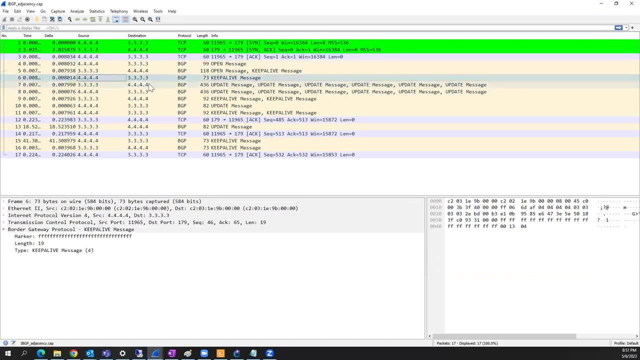 so, if you look at this, this is a successful tcp connection establishment happened and both formed and both established a bgp connection. then it's exchanging the updates and inside the updates it's sharing its nlra information and it is sharing its autonomous symbol system and it's sharing its as path. all this value, so you can check end to end. 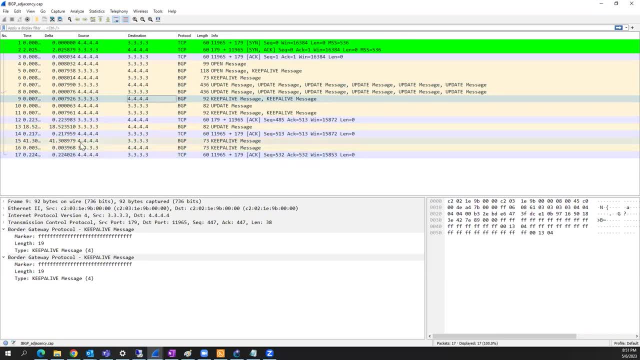 is it something problem with my parameters? is it something wrong with my updates? it's not something i should look at. you can see the keep alive packets, a lot of keep alive packets. why there is a latency here? because 41 millisecond and for 18 milliseconds and 41 seconds it's giving and keep alive if it. 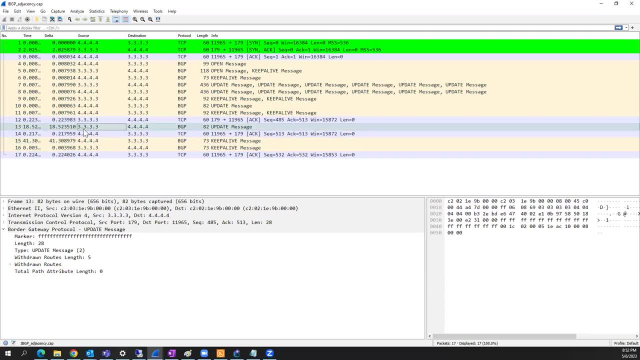 is sending an update. that can be considered because after 18 seconds you made some changes in your domain and you- you made some changes in the router for specific to the bgp. so after the 18 seconds you- i mean you- made some changes and after 18 seconds it sends an update back. 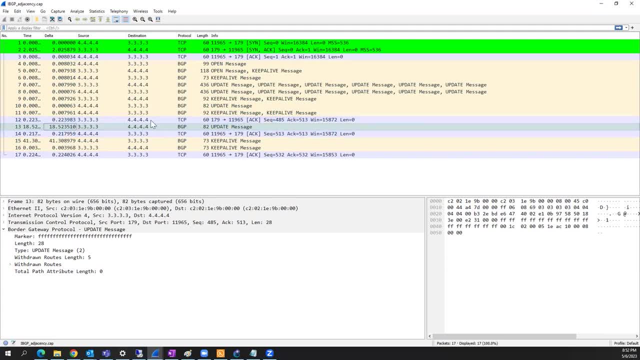 so the update is coming on. so you're doing some configuration. but if you look at this keep alive, it's taking 41 million 41 seconds. so that is a bit higher. so you have to look at why. i get you know. after 41 minutes 41 seconds, i got a reply from 4.4.4. you have to look at the router. 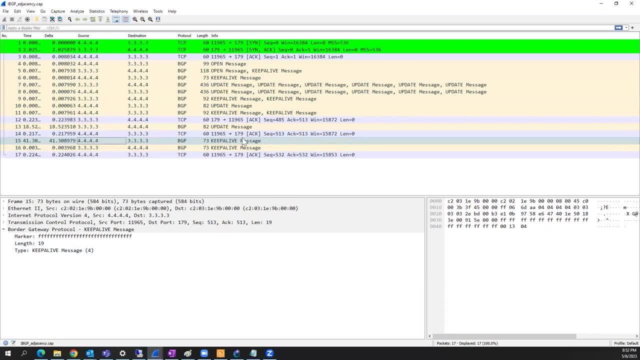 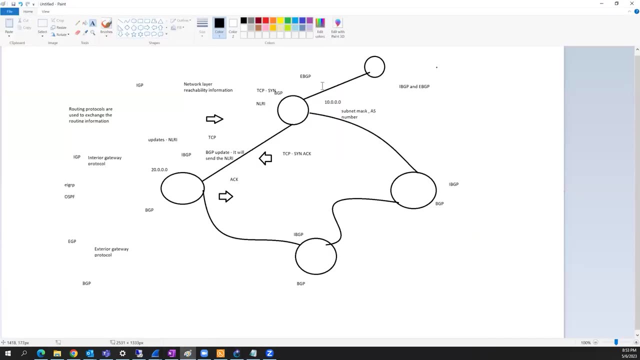 so this is how bgp looks into and how wireshark can interpret those values and we can use it for troubleshooting. so the key thing is the bgp. it will. the bgp is the first thing is only if your tcp connection establishment happens, your bgp update happens. so if your tcp connection establishment fails, 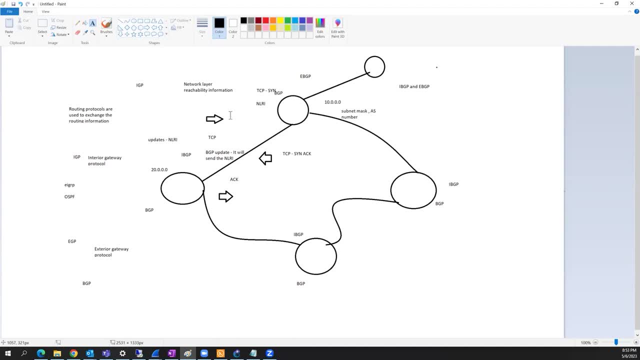 and your bgp will not work here, and we talked about igp, so the ibgp that comes under igp. this all works within your autonomous system and the only protocol which talks to your isp and the head-end router is ebgp. it has to be a ebgp neighbors and it should share its nlri information network player reachability. 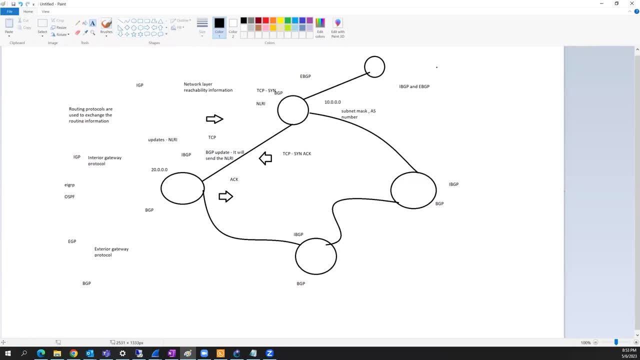 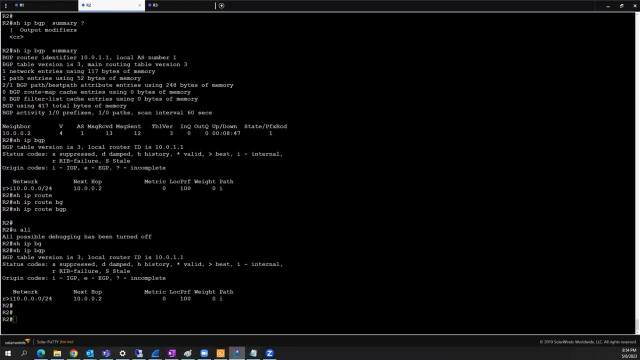 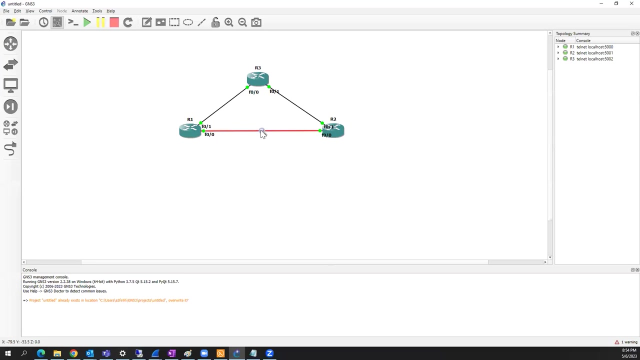 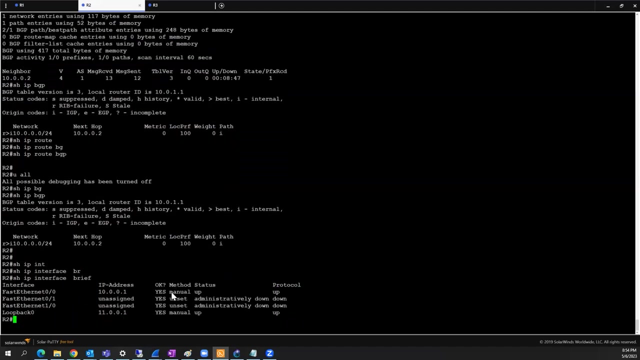 information between both. so this is how a successful adjacency looks like in bgp, and let's see the action, see what we can do with the lab, and we'll do a capture there. let me stop this capture. if you look at this, i made a very simple config. 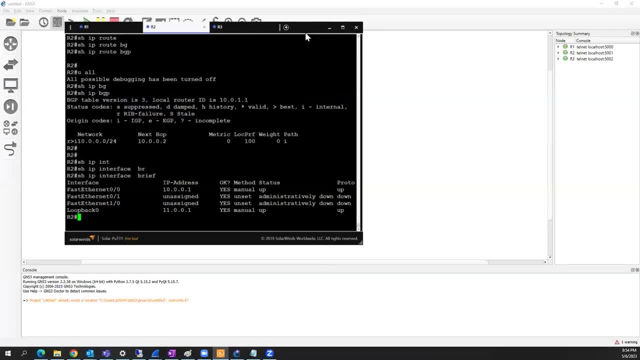 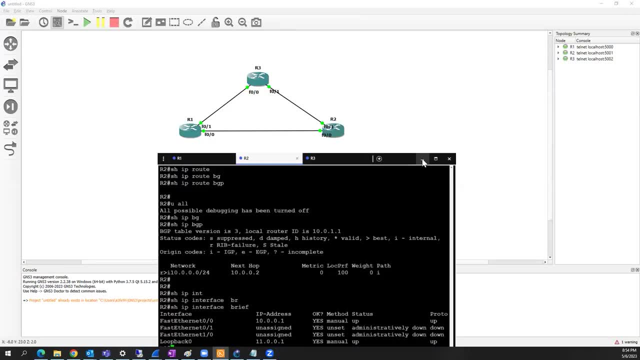 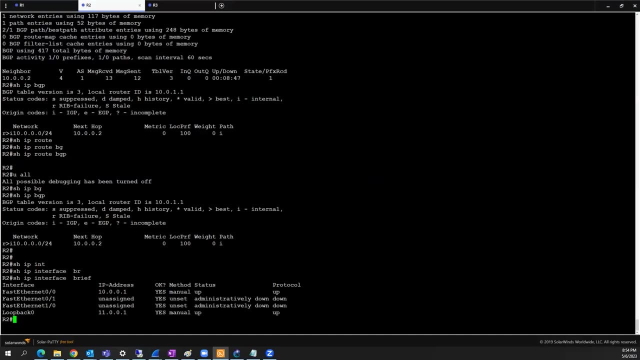 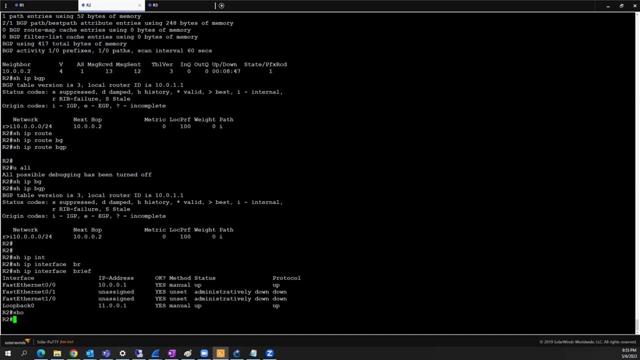 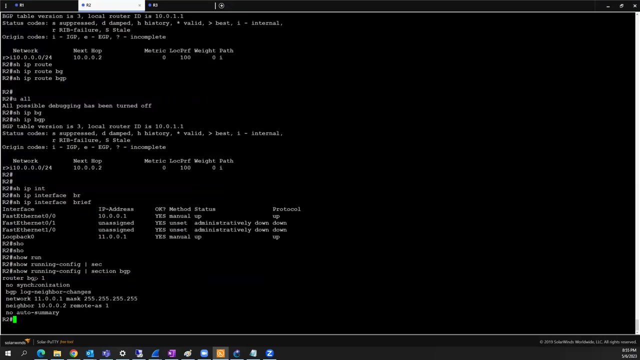 i have two interfaces on router 2: fast ethernet 0- slash 1 and fast ethernet 0 slash 0. so the very first thing is i have to check my interface status and protocol is help, and then if i give show, run section bgp, pretty simple config. so very first thing is we will define the ace number. 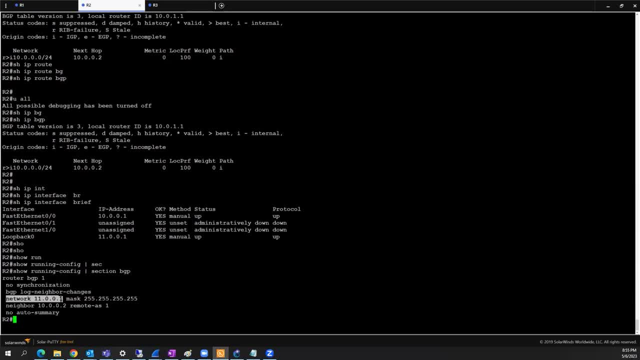 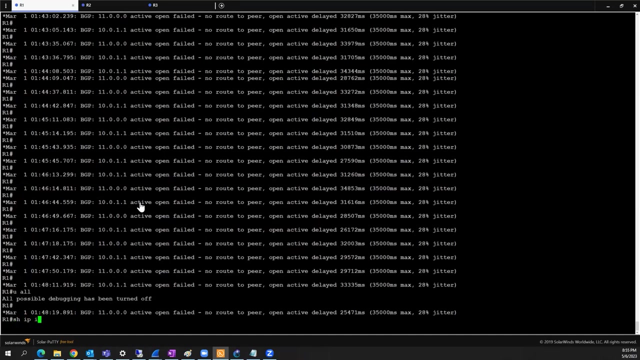 and then the network. what i have i i got two network here, so 11 network and 10 network. i didn't advertise the 10 network, but i have advertised my loop loopback ip address here. see me if you look at this config. i have only one ip. 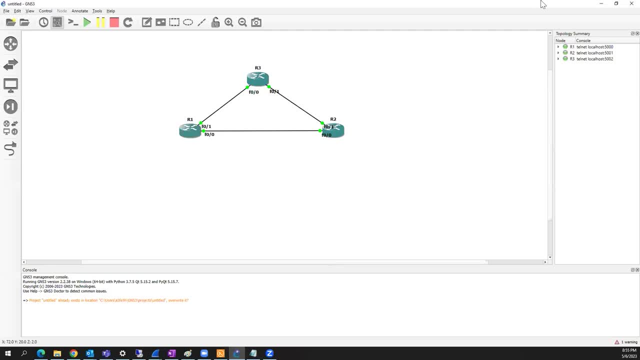 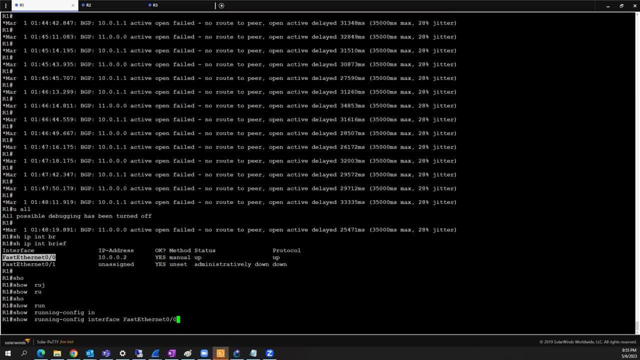 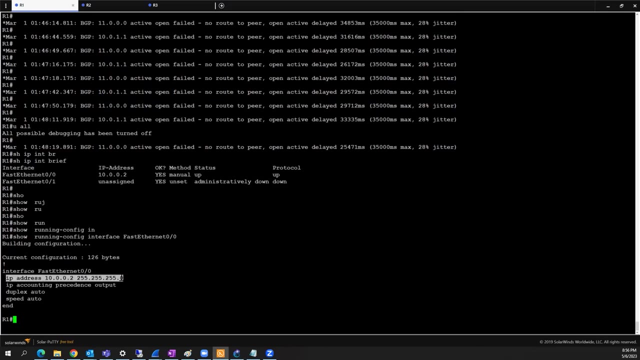 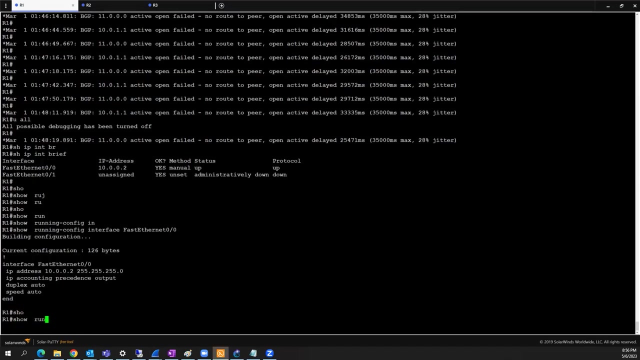 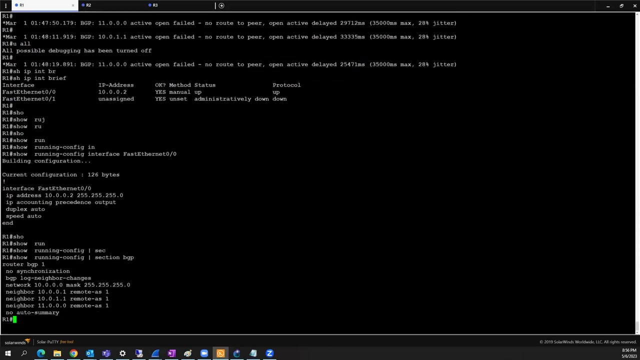 configured on router, one on fast ethernet, zero, slash zero. so this is just something i can. i have given the same point-to-point connection, so it is just 10 network. i have given ip address of it and, if you look at the bgp, so i have advertised my network. 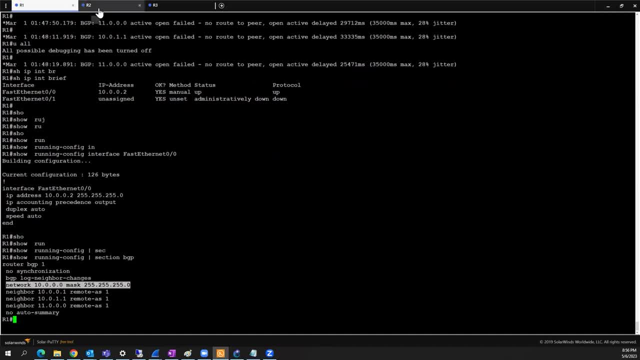 and i said my neighbor, it's ten zero, zero, zero network. so it's in. my neighbor. i said it's ten zero zero one, and remote as is one. and i have to. you know, this is something i'll advertise, so. so i have to make a neighborship and i have to advertise a network, only then. 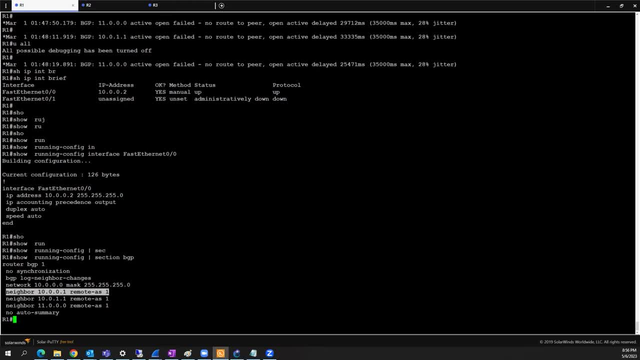 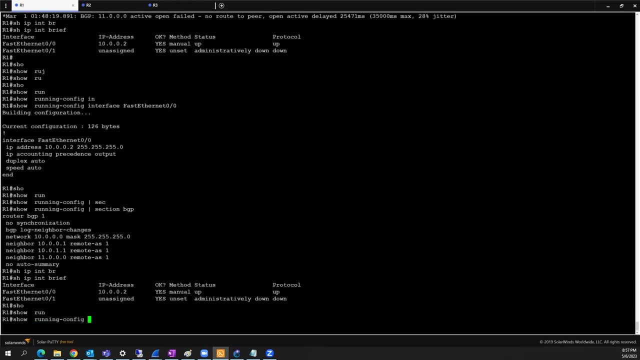 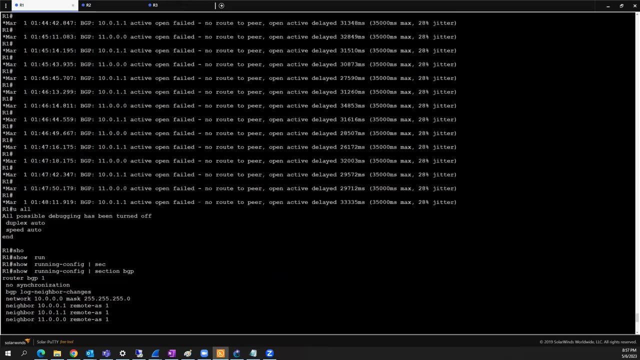 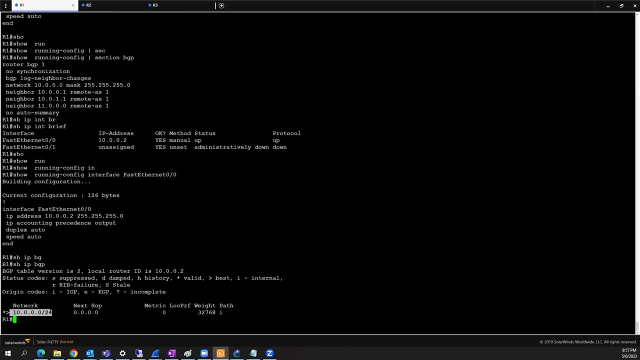 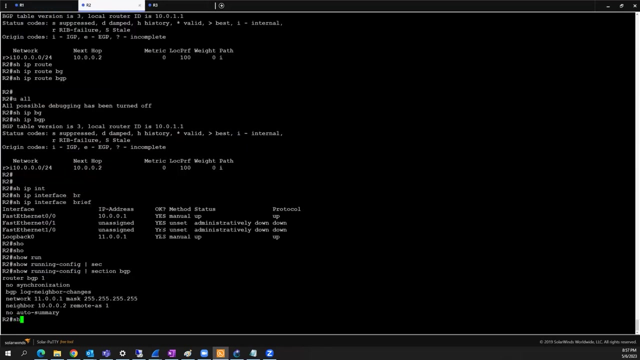 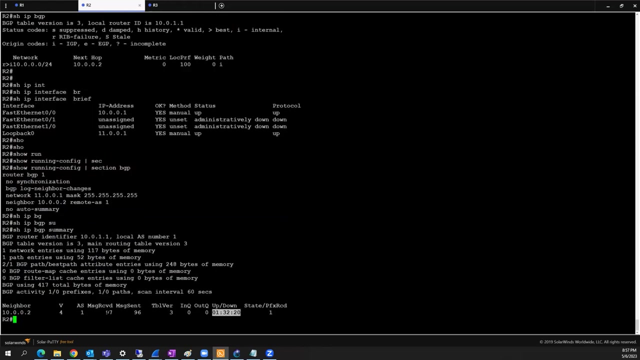 your connection establishment happens here. and if i give show ip bgp it says this 10 network, the default weight value and i stands for igp. if i go back here show ip bgp summary, it shows my uptime, it shows the number of messages i send and receive all these details here. 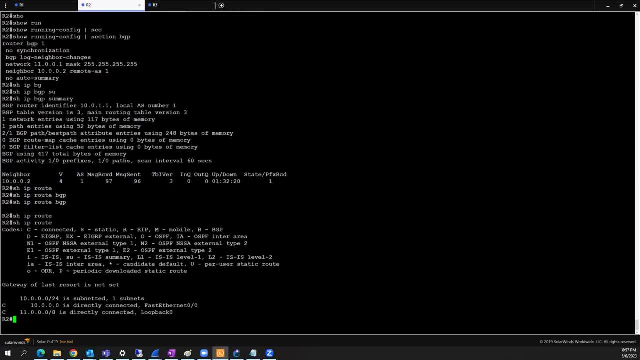 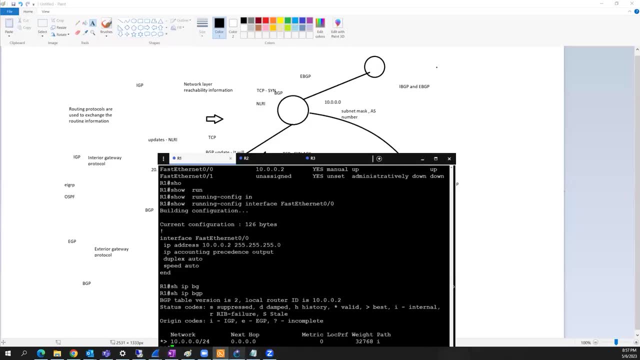 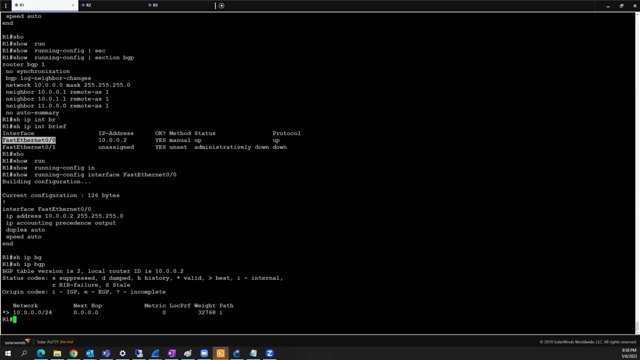 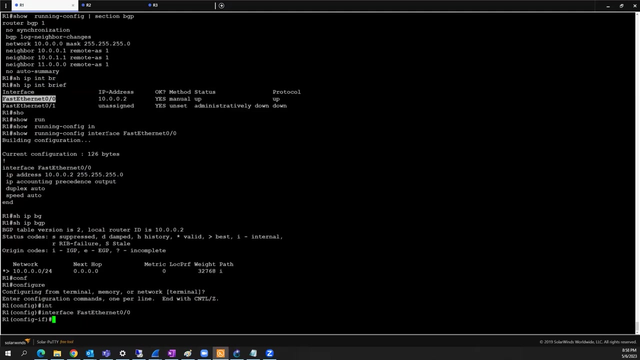 so i have to say it's 10 on 10, so it offers the directly connected route. so now i have to specify my network. so let me go ahead and say it's 10 on 10, so it prefers the directly connected route. so now let's go and shut down the port and let's see what is the message we see there. 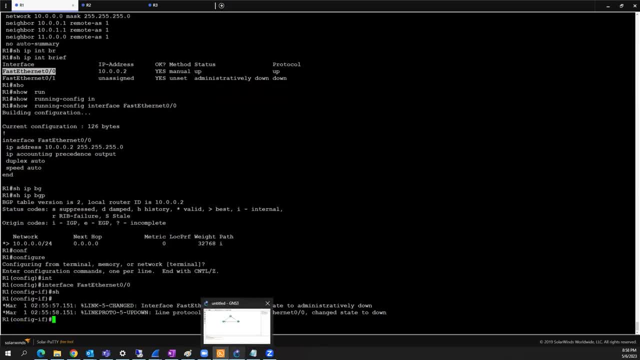 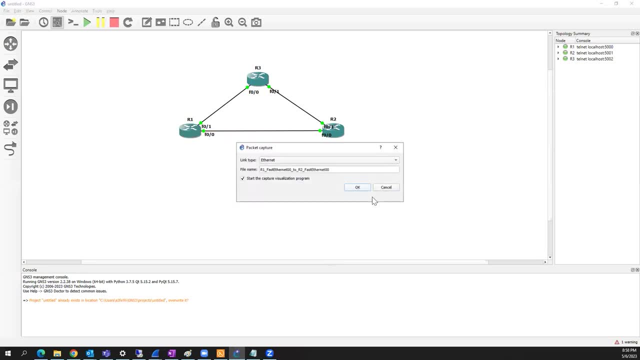 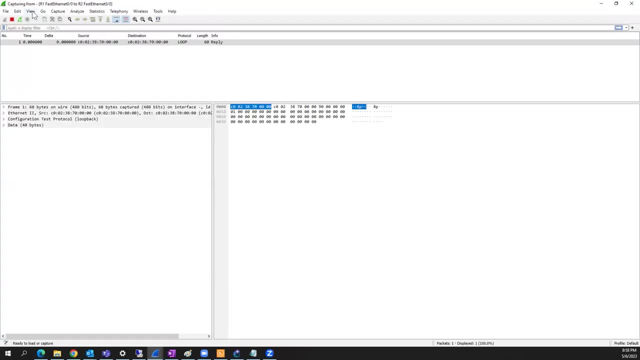 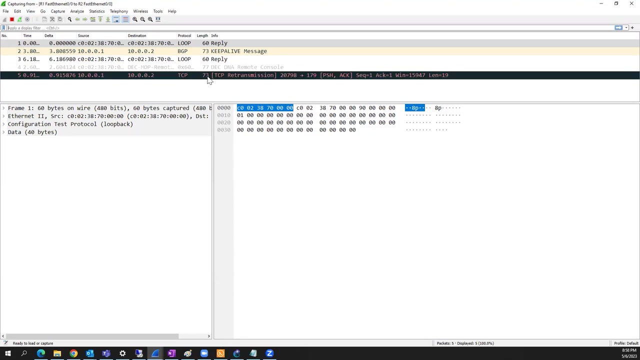 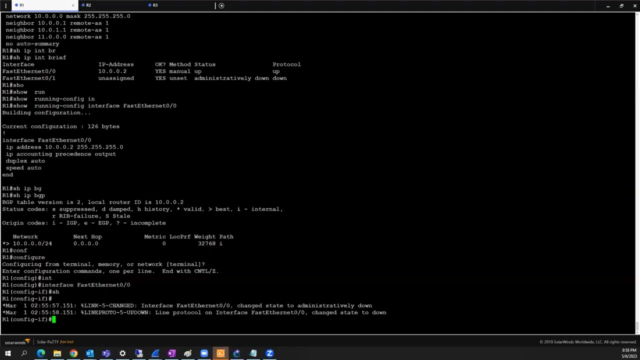 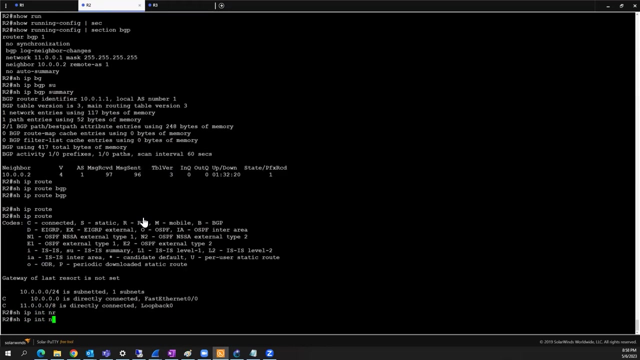 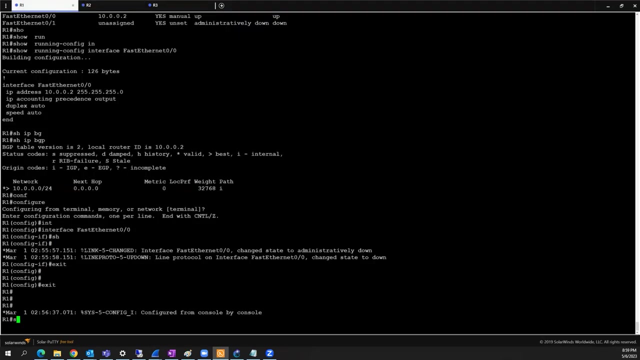 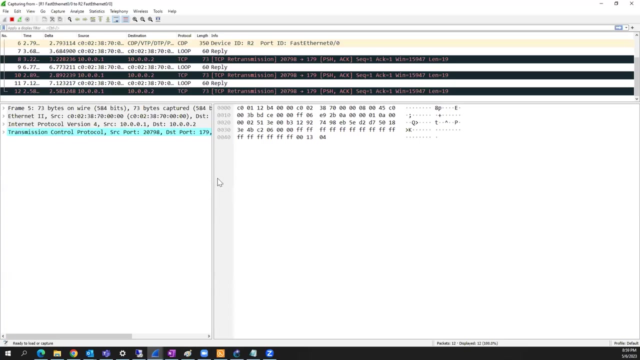 so. So you can see 1001 is doing a retransmission because the port is down on router one and it is 1002. it is continually sending a retransmission, so it is hot down. so i established a bgp connection and it is down. 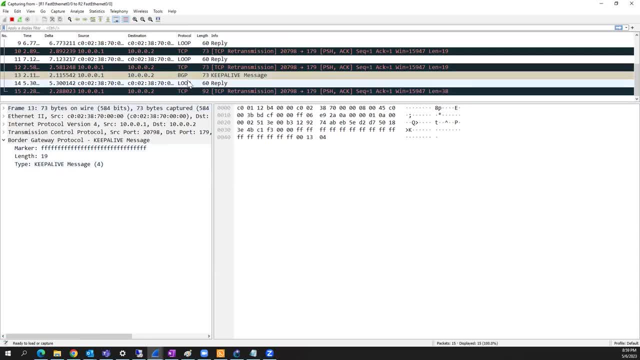 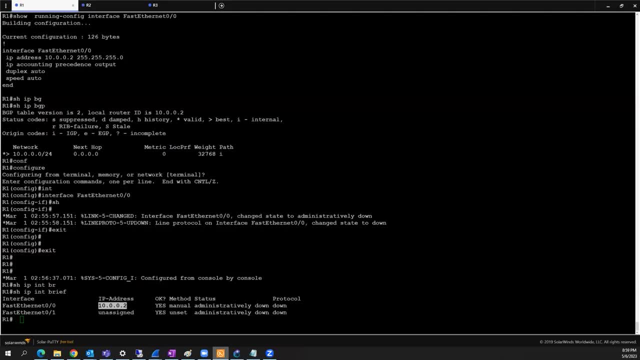 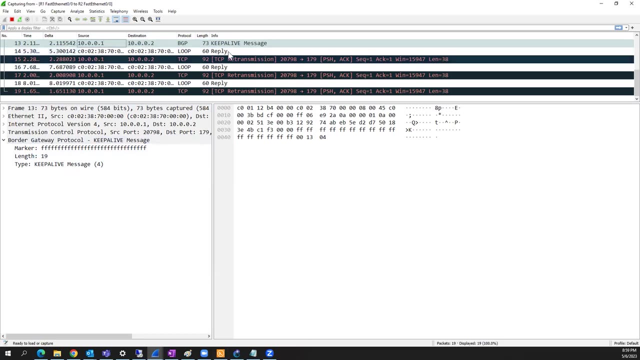 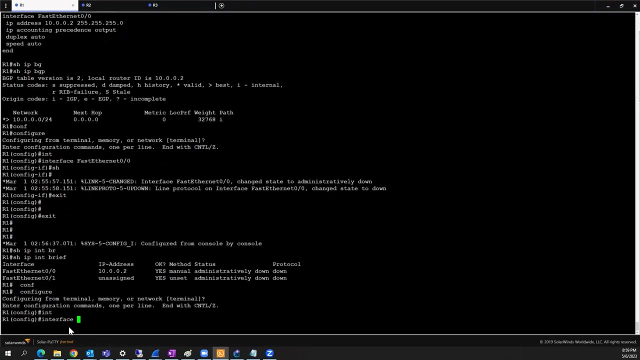 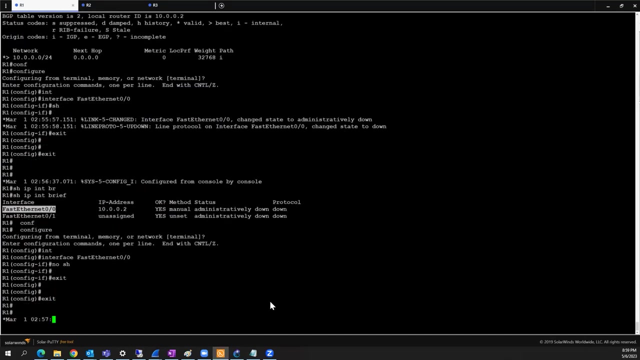 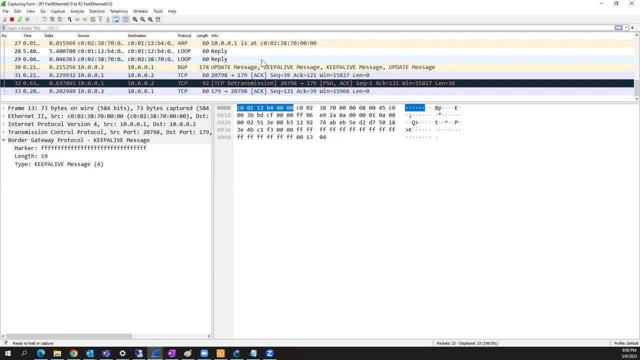 so it is sending a keep alive to make the session open. 1001 is on the remote end. it is sending a keep alive and you can see i'm not sending a keep alive back. but if i go back, i gave you no shutdown and now let's see the bgp update. 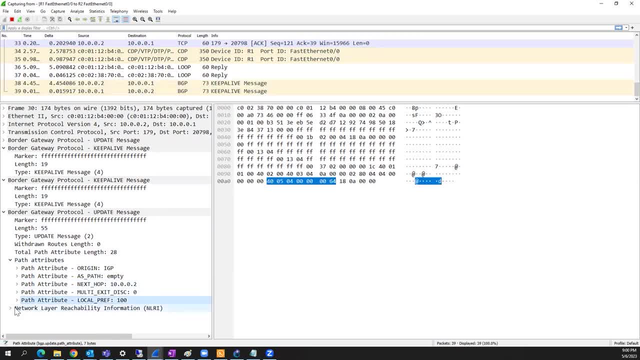 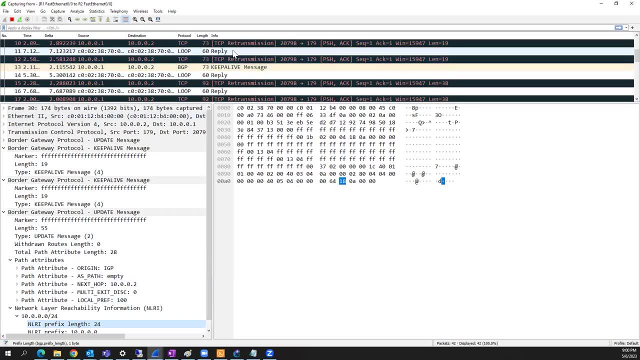 it says the next stop is 1002. it's a default local preference and then nlri information i can see here. so when it was down, so it is sending a retransmission and it's sending a keep alive 1001, but i am not getting a keep alive back. 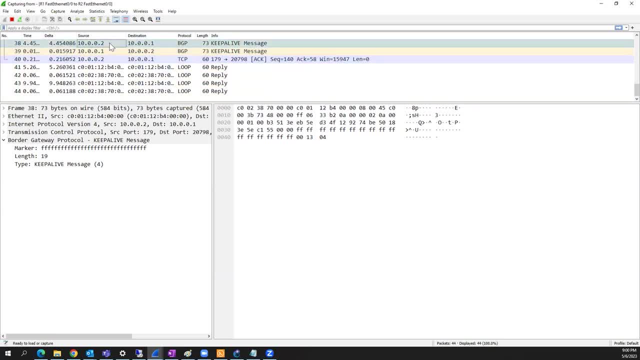 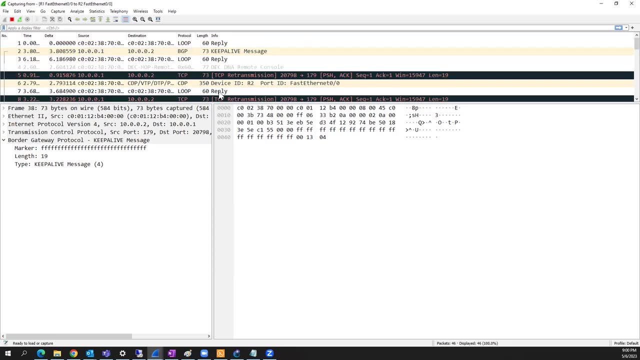 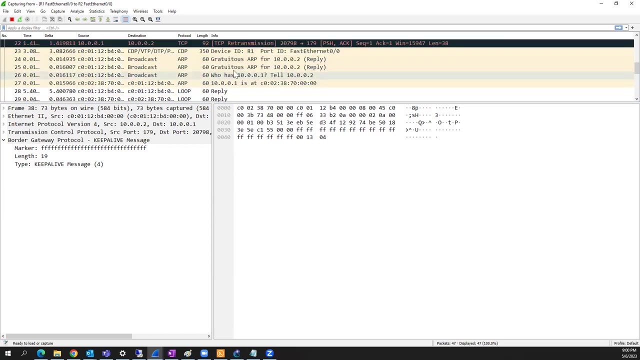 but if you look at here again, the 1002 is replaying back for the keep alive sent by 1001 here and this is the port that is down. it is coming up, so it sends an arc and this is evidence that the port is down. it is coming up, so it sends an arc. 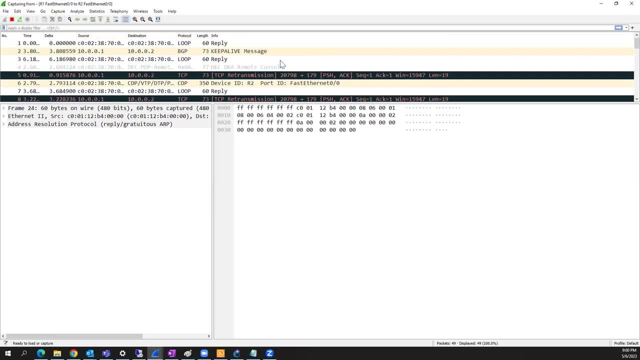 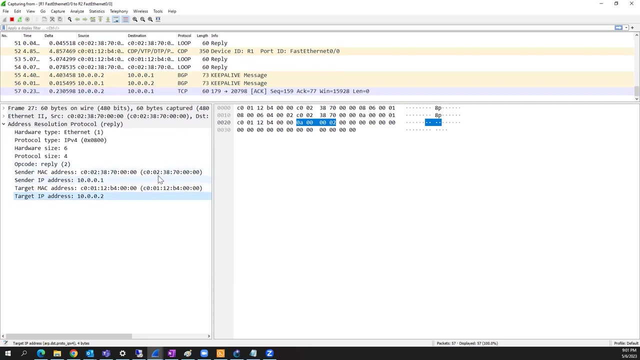 for the off request, i get an arc replay back and the gracious startup it says i go, i, this is my address, i am back. and for the art request, it sends a replay back so you can also compare the mac address for the same. so this is how you can. you know, this is just an overview of it, so you can. 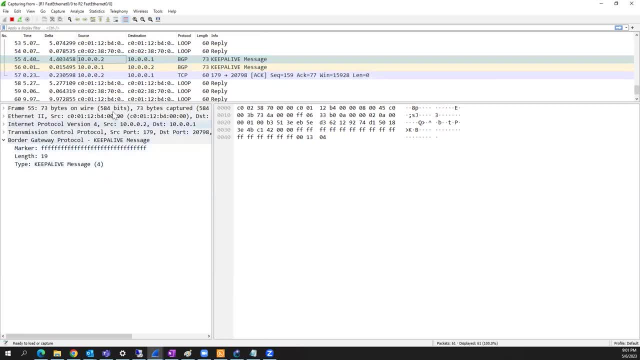 dig deeper to find other stuff. but, as we discussed this in the successful adjacency, the bgp updates, if you look at this you will get- you'll get all this information here. so if i suddenly i see there is a keep alive package that's coming in, so it means that i i made a tcp connection establishment successfully. 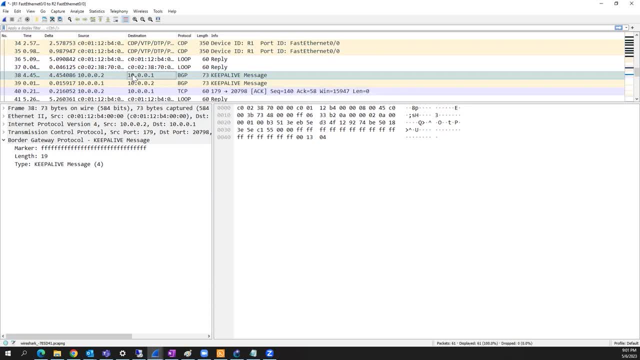 but i didn't get a reply back after some time. there is something problem. it's a device physically hot down. that's why i send the keep alive right, so there is. there is something in the middle in the network path. i lost connection to it. so for that keep alive, i get to keep alive. 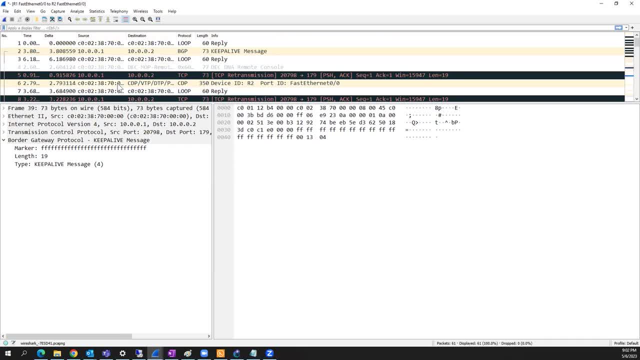 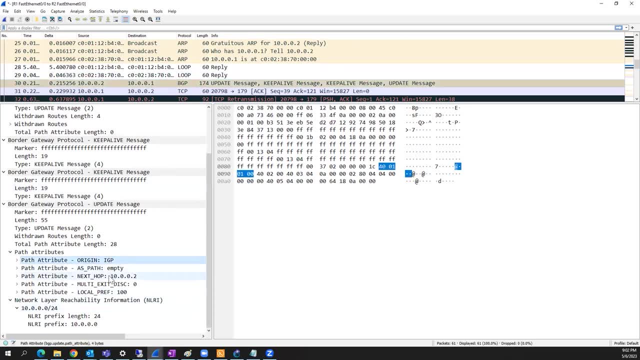 back and after in the bgp update i see the nlra information. so for that, keep alive, i get to keep alive. back and after in the bgp update i see the nlra information, the absolutely, and i'm running igp. it differentiate with the as number. so in 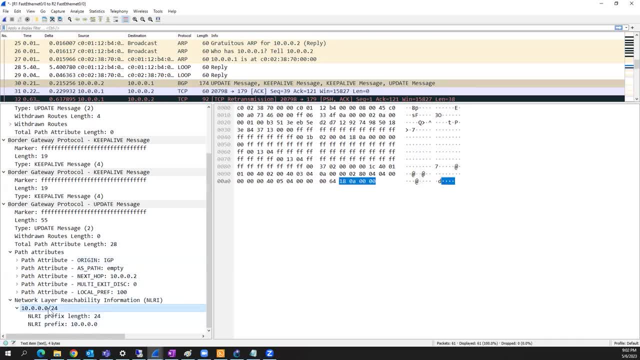 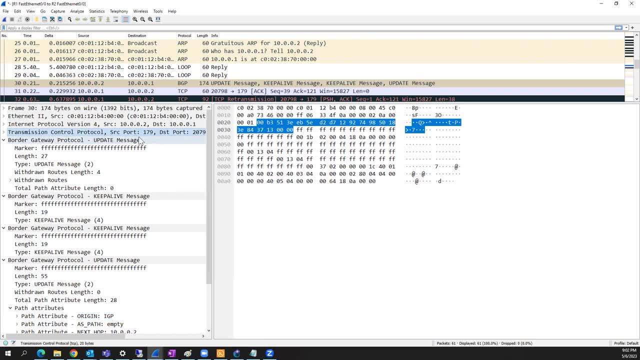 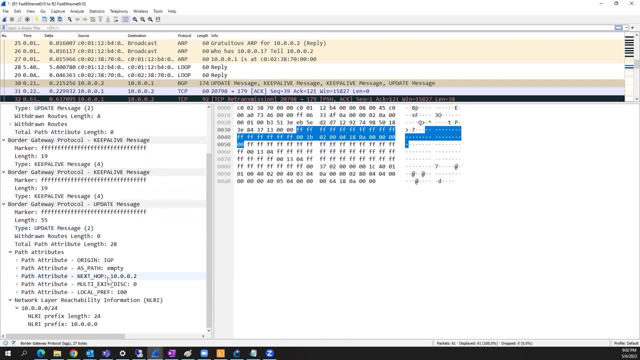 the nlra information. i see the attributes. what is the information? what is a network update? and, if you see, always it uses a port number 179, tcp port number 179, and it says it's a bgp update. and since i don't have an aspath attribute configured, i don't see anything. 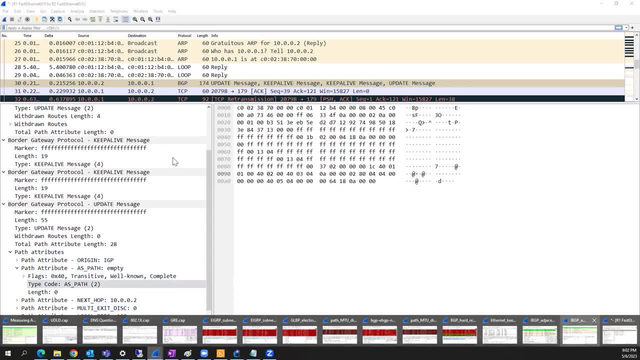 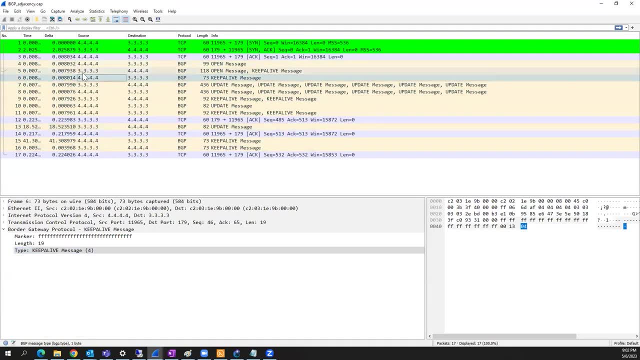 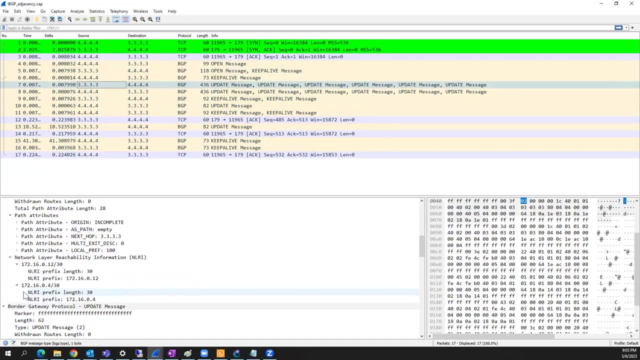 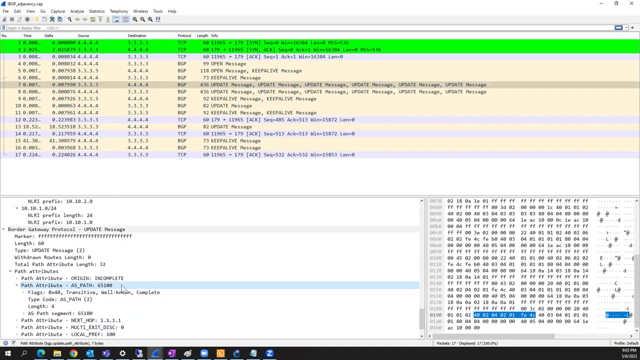 But if you compare the BGP connection adjacency- what we discussed earlier- You can see your AS path value here: 65100. this is the AS path because it's been configured with path address. So all your path attribute. you can see here your local preference, your origin, your AS path, all your path attribute. BGP has different path attribute, right, so you can look into all the attributes. since this is not BGP deep dive, I'm just showing how Vireshark can interpret those values. 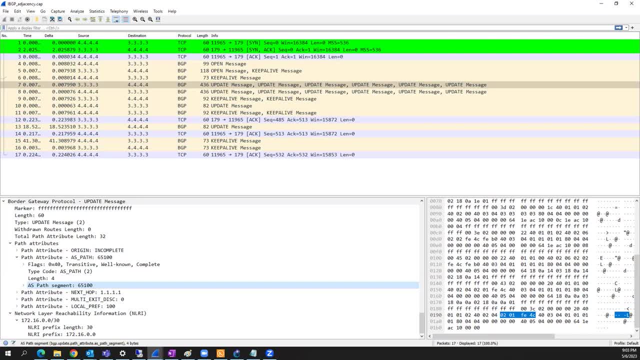 So you will get to know about your weight, your local preference, your AS path, your MED, your matrices. All this, all this information. you can see this is pretty helpful when you do do a troubleshooting and you'll come to know this is something very simple. I know simple false book we did and we try to figure out and who's doing a retransmission and who is sending and keep alive. so it is something that who is sending and keep alive and who's not sending a keep alive back. so it means that I know who's the destination, who is not sending a keep alive back, so I can jump into that particular outer and I can see my BGP can fail. 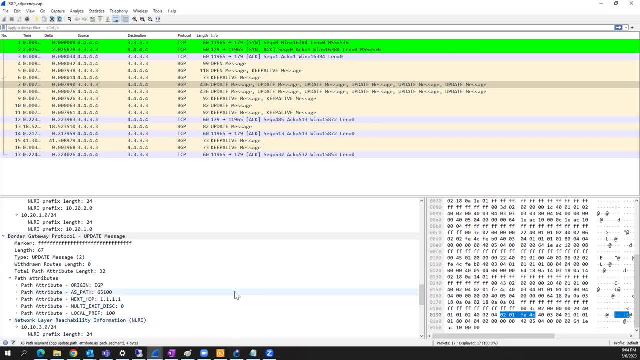 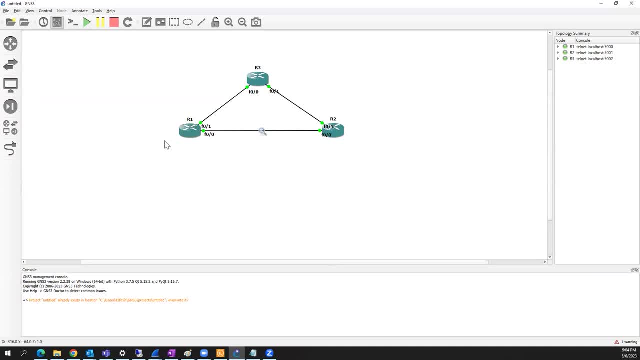 But you can sense enable your BGP keep alive in the router. but that is a router intense task so it will keep sending your BGP. so it's always better to use a Vireshark to capture that, because when you have problem early then you're going to look into your. all your TCP keep alive. so it is always suggested to do a capture with Vireshark. 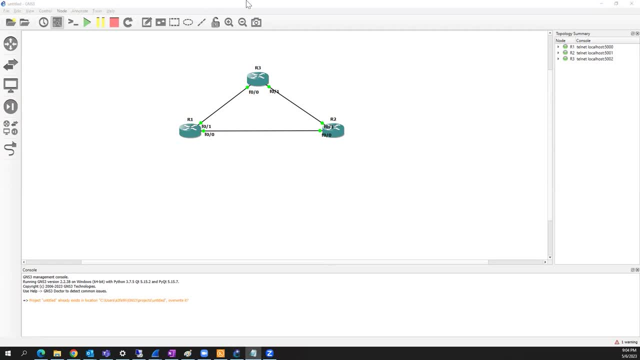 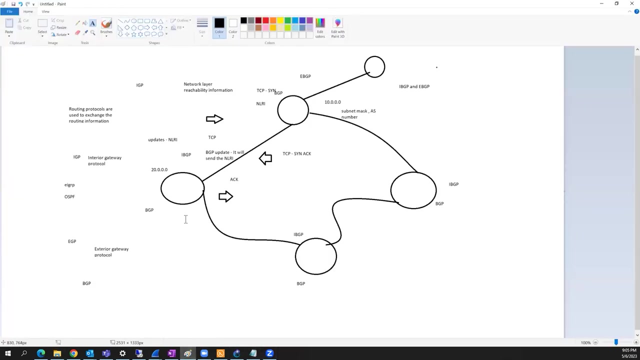 so it is always suggested to do a capture with Vireshark. yeah, now let's see what is EIGRP and what by design, and how vireshark interpret those values. So now let me give you a little bit background about EIGRP. 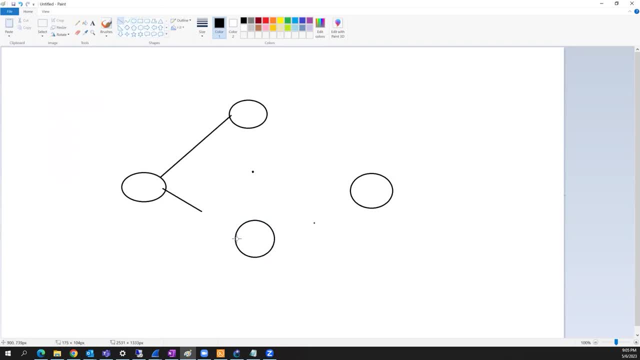 EIGRP. So here I mean EIGRP is not using PCP, anything like that. so EIGRP is routing protocol. all it does, you know, to make the connection active itself some hello packets. but I will give you a background about EIGRP. so this is complete. 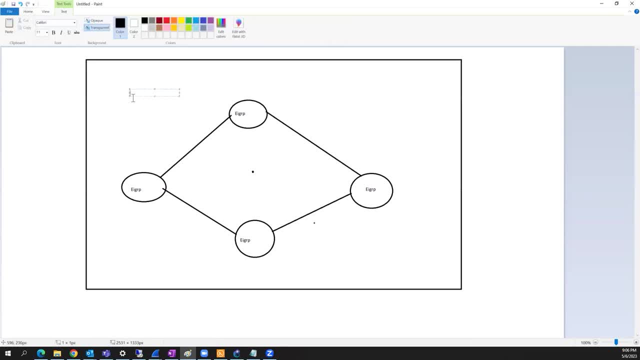 in IGP protocol so that is used within your autonomous system, your offers that cannot be routed in the public. so, example: this is your EIGRP hub and this is poke, so this is your DMVPN hub, example, example. so I make a neighborship with all the CHRP. 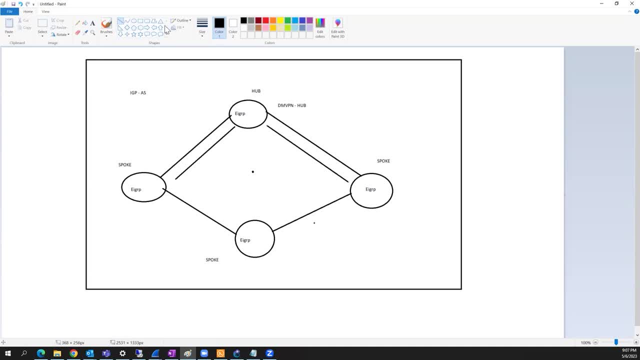 the DMVPN stands for the DHRP and this is the DHRP hub: dynamic multipoint vpn. so why this is widely used? um example, if i want to make a tunnel with a spoke, it's a dynamic tunnel. so it's a dynamic tunnel between the spokes. so from the hub it makes a tunnel back and 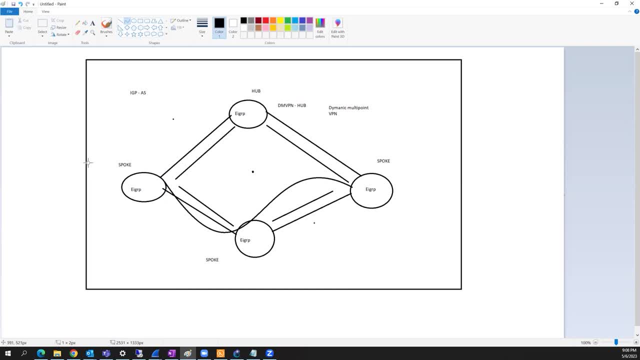 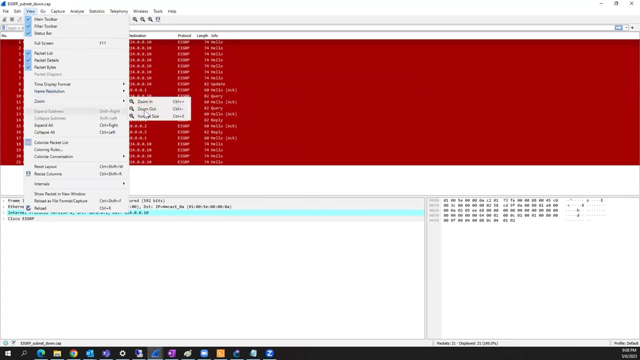 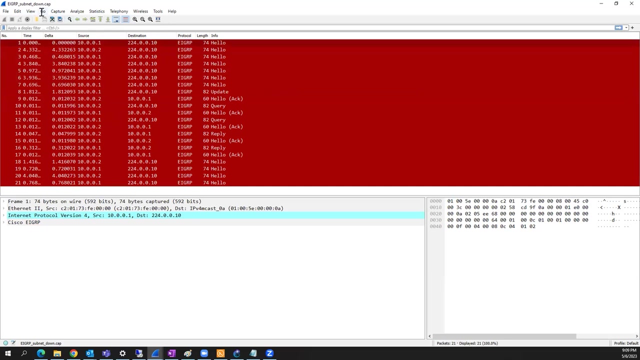 with the wireshark how i'm going to figure. i'm going to troubleshoot the ehrp, so for that i'll open a active capture. so the very first thing is: first we should have a routing, then it will send all its updates to its multicast address until it forms. 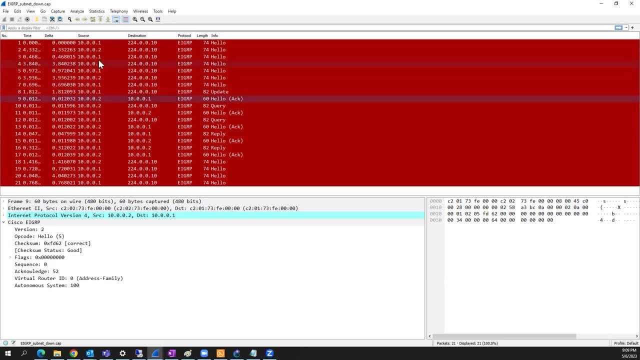 the neighborship and if you look at this, what are the values it shares? so it says: i'm running cisco ehrp and the version and it is an hello packet and my checksums are all good and if you see the soft version of ehrp, it's version 12.4. 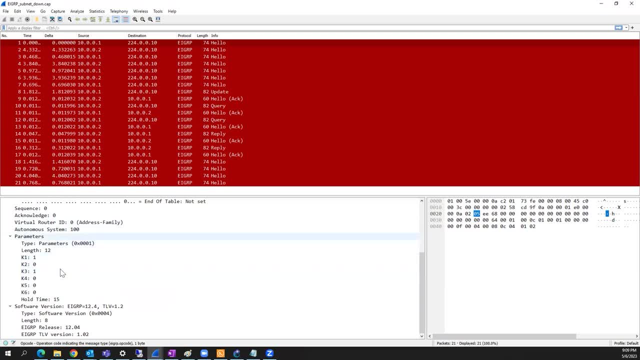 and if you look at this parameters ehrp, it make use of this k values. so we are not doing a deep dive about ehrp, but i'm telling so here you can see your hold down time. so it wait for 15 seconds. if i'm not getting a hello, it will wait for 15 seconds and it's talking. 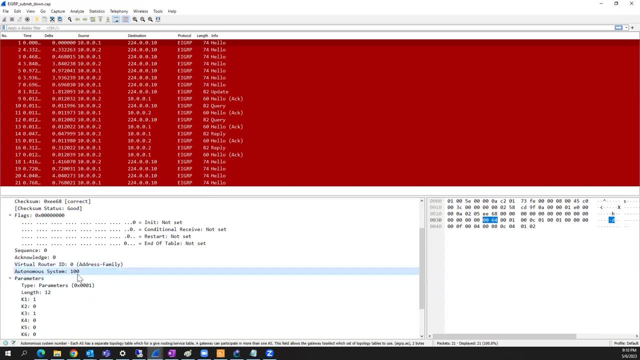 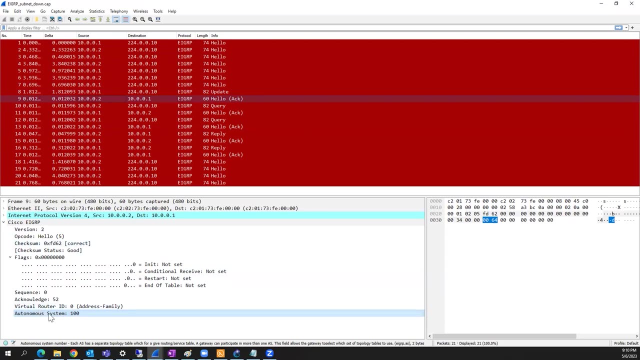 about its autonomous number system. so my autonomous number system is 100 and it has to be same on both end, otherwise your neighborship will not form, and from 1002 to 1001 it will. if i look the update and it says my autonomous number system is 100 and it says my version. 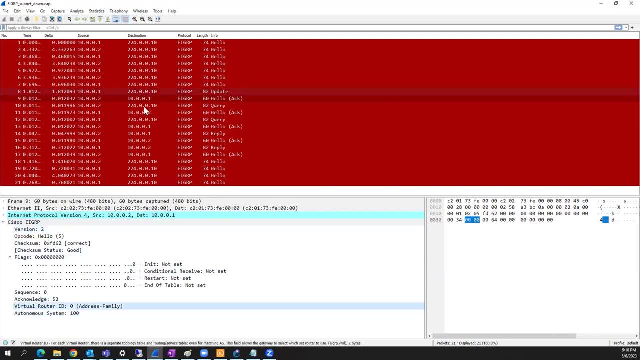 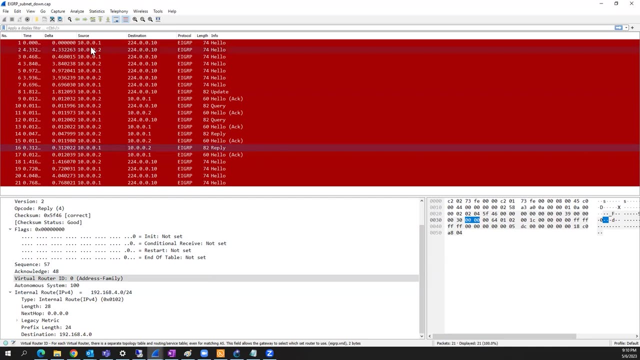 is two and if you look at here, the ehrp update. so once it sends an, you know updates to the multicast address, once the neighborship is formed, it's going to show me the internal route information. so nlri information. the prefix length is 24. 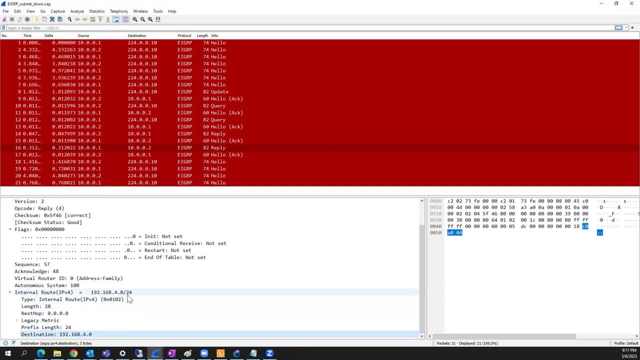 and the destination is 192.168.4.0. network and this is my prefix length and it shows about my delay. and it shows about my delay, my mtu, and if you see mtu mismatch you can figure out that your reliability load. all these are ehrp matrices, so ehrp it uses the delay and bandwidth mtu. 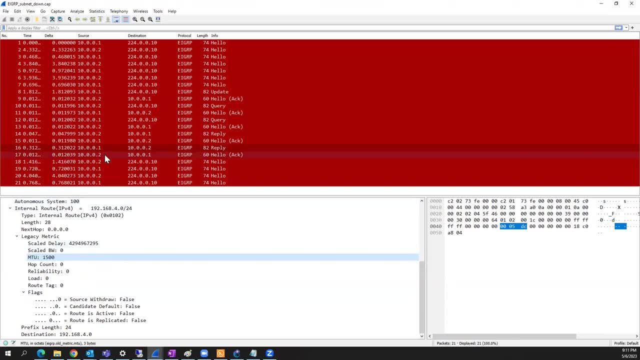 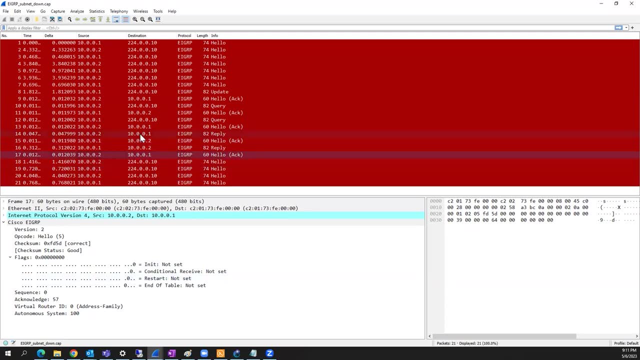 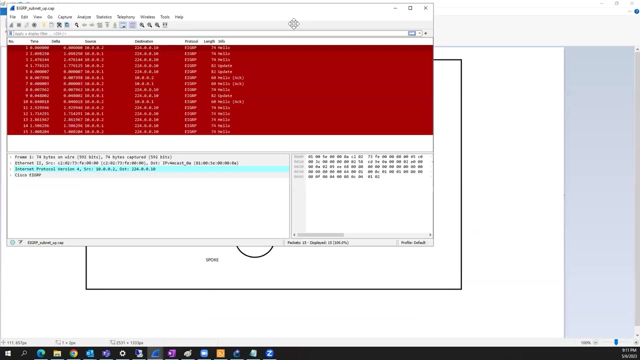 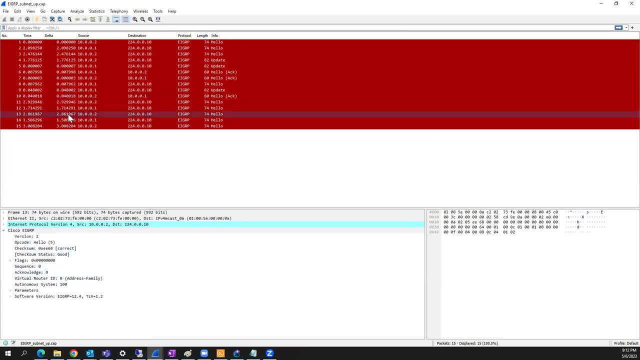 so you can see all these values here. so this is an hello acknowledgement. so there is definitely a connection between these two. so you can compare the parameters, what all the parameters i have, and is it matching the whole path? what the value is, get the use. you also have the. 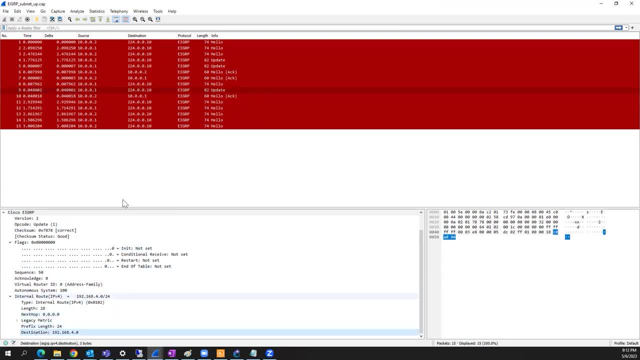 so you can even see the intel route information, your, your next stop details, your prefix length. what is the network that's been advertised? you can see everything in ehrp, but it is not using tcp. but it is not using tcp. so this is something once in both the source and destination, it Halo adventure. 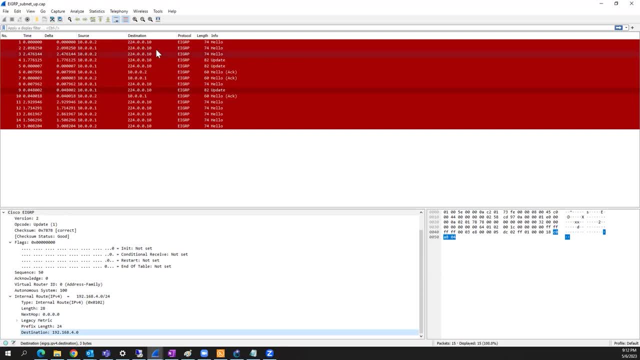 source and destination. it sends all this update in the hello updates. it sends to the multicast address. so once the neighborship is formed within source and destination it's going to exchange all its information between the source and destination, not with the multicast. so if there is an update, 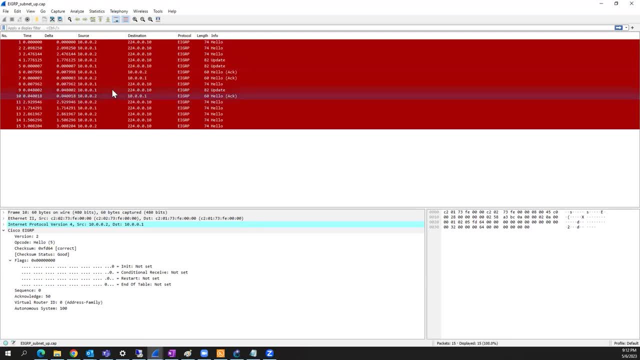 it sends, as i know, hello and it sends an update. so inside the update information, if you look at this, it sends to the multicast address is something in my topology. i have changed something and this is an update. so what is the update and the route information? whatever it's been changed. 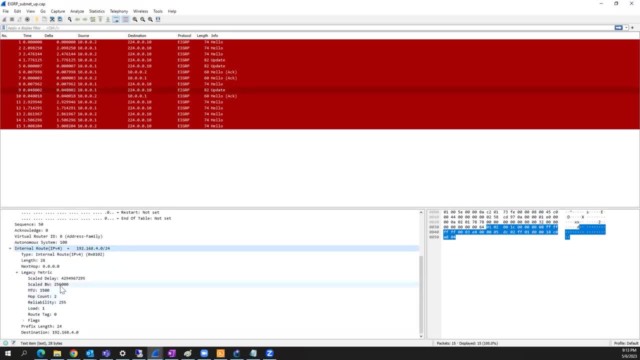 it's going to advertise the same. so you can also see the bandwidth here. it's pretty useful when you do a troubleshooting you can compare. so all the values, whatever you you have given, is it successfully happening on both end? let's again give you a, you know. 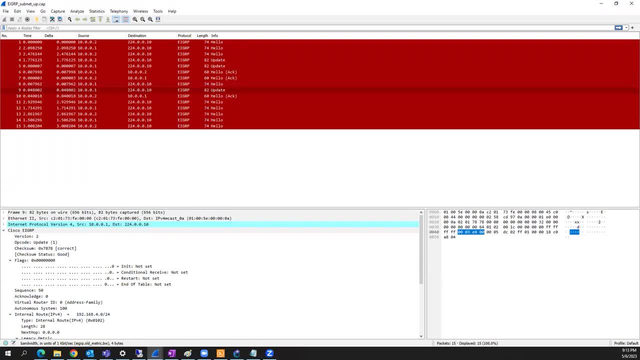 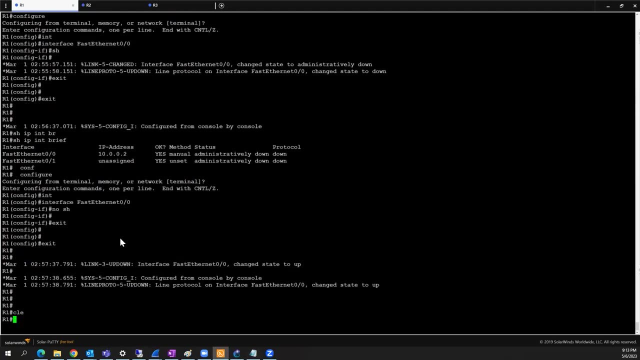 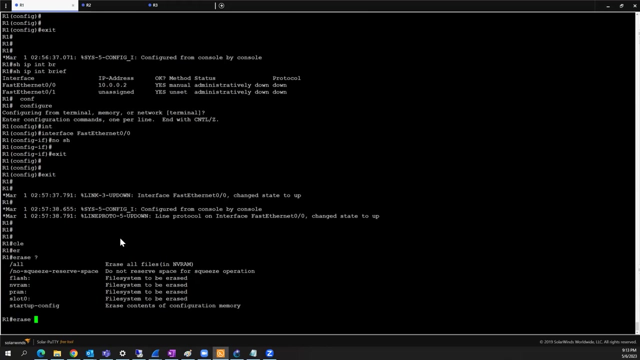 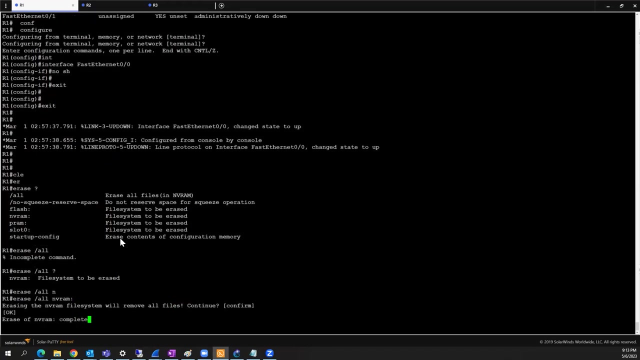 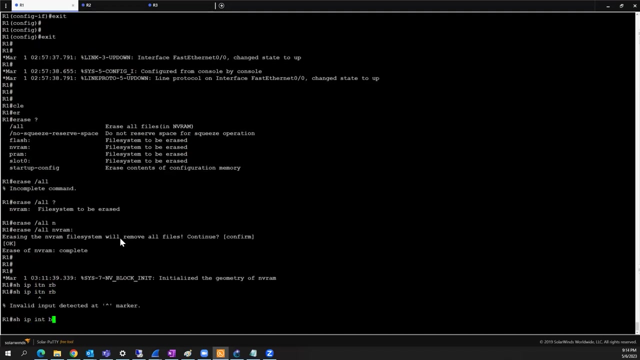 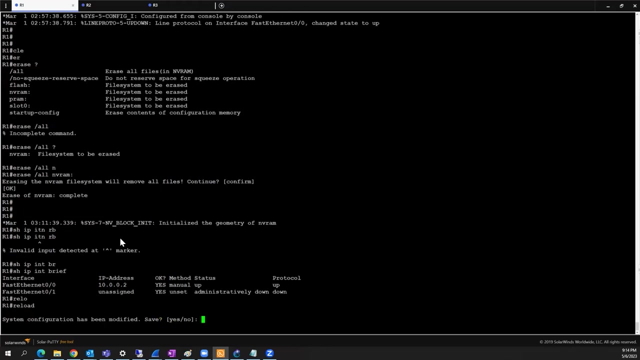 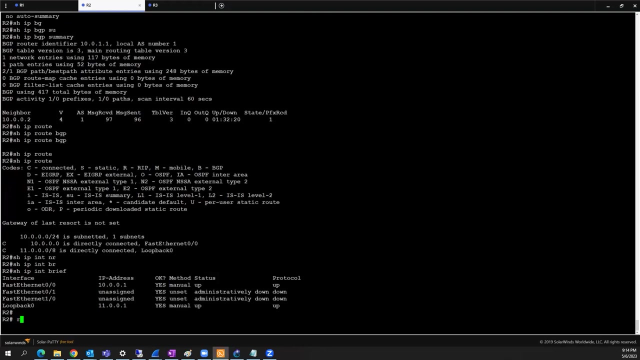 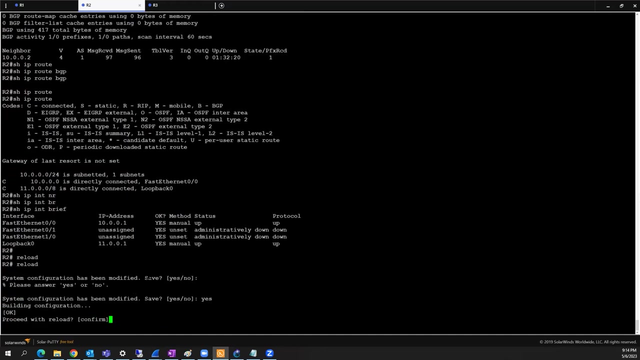 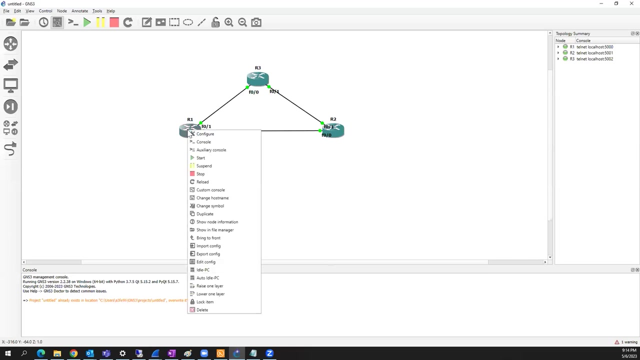 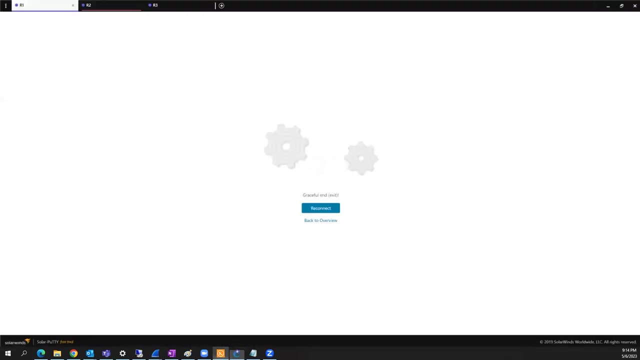 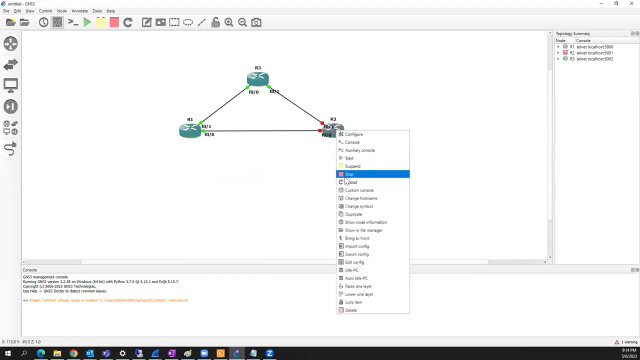 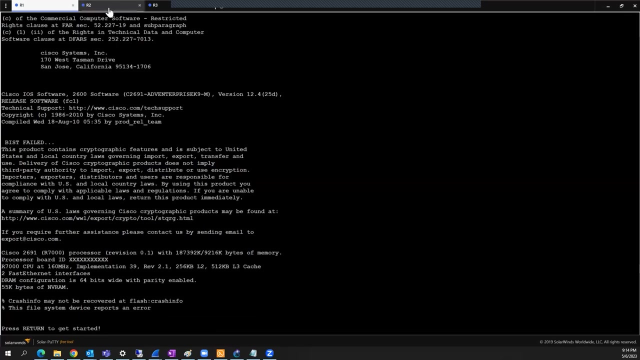 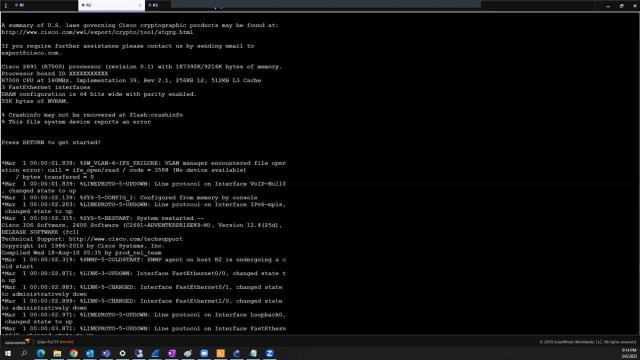 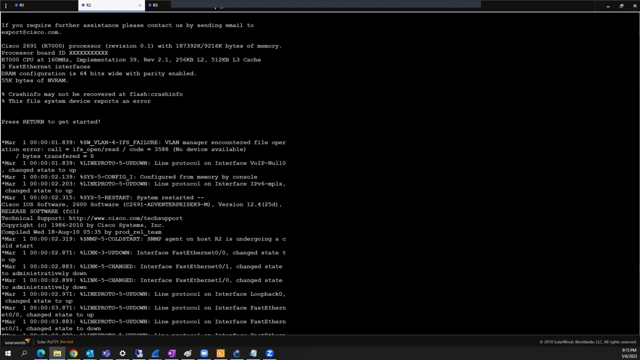 what's a view about the complete eagrp process here. so now let's do a lab for eagrp and let's take a capture and let's see how, exactly what exactly we see there, you. So I'm going to reload this. I'm going to reload this. 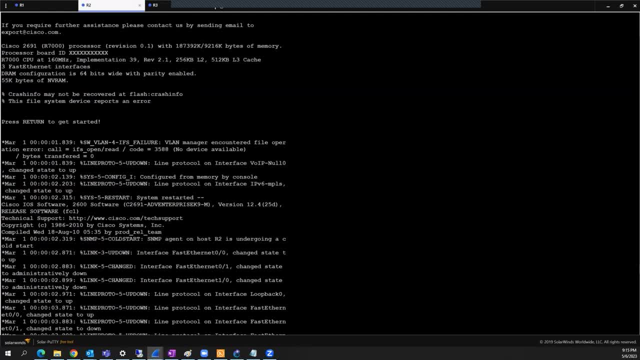 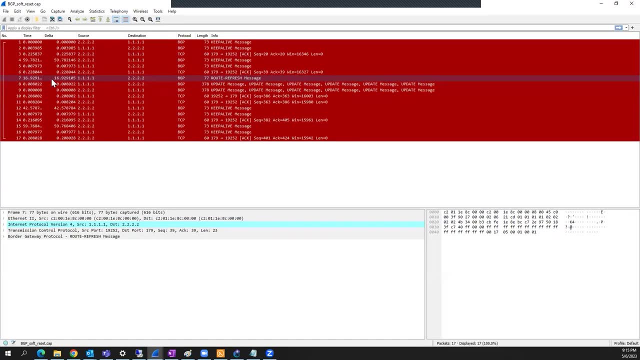 So in the meantime, even the Wireshark. in the Wireshark we see if there is a, you know, soft reset. If we are doing a soft reset, it's going to acknowledge that some soft reset happened. Is it something in the software level? you give clear IPBGP logs. 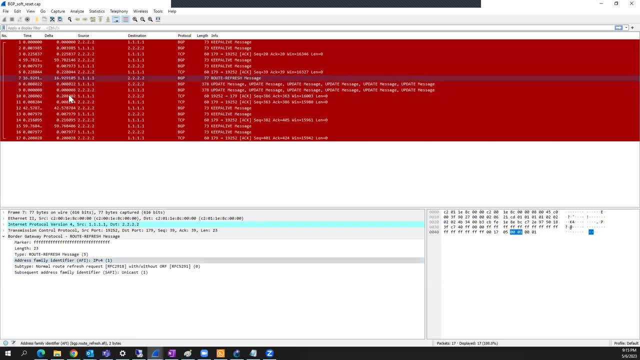 So once you do that, you even get that information. Somebody the remote tends to 1.1.1.. It's, I mean, the router that the route originated from. 1.1.1, that's been, they have been, BGP. 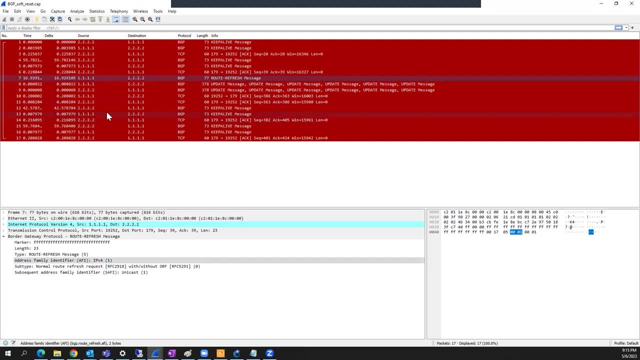 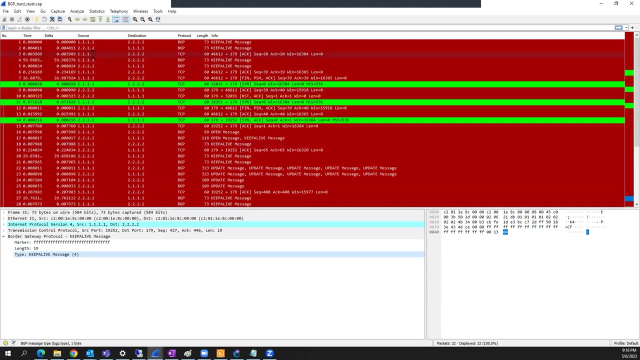 soft reset there. So this is a comparison for hard reset and soft reset. If you see this, because it is a hard down, then again it's in SYN. For the SYN. I got a SYNACK back and I got an in. I'm acknowledging it back and I see. 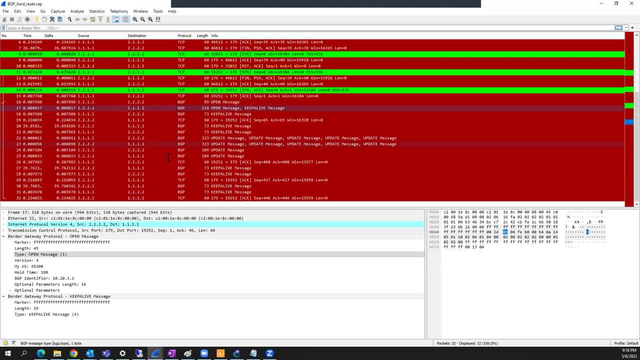 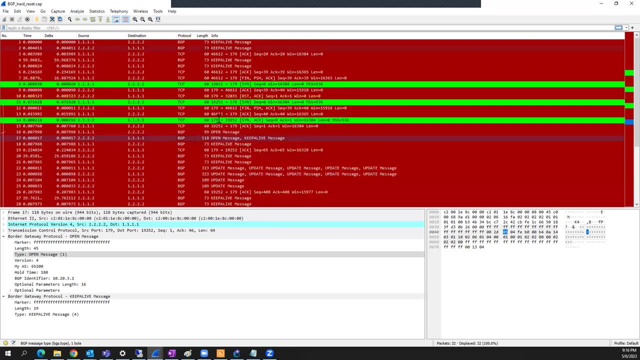 the open message and everything. So this is hard reset. That's something somebody they need to admin up and down on the interface. So that's the difference between DrunkRefresh and this hard reset. Even you can see those information in the wire shot. 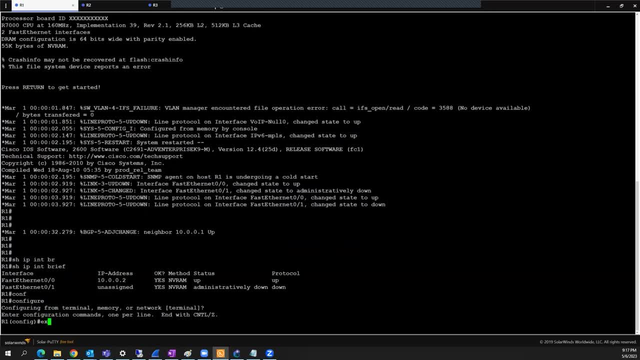 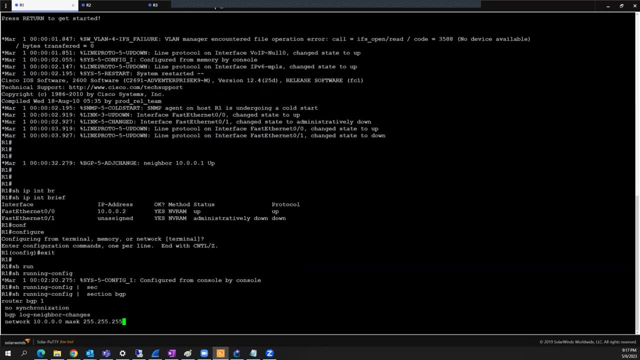 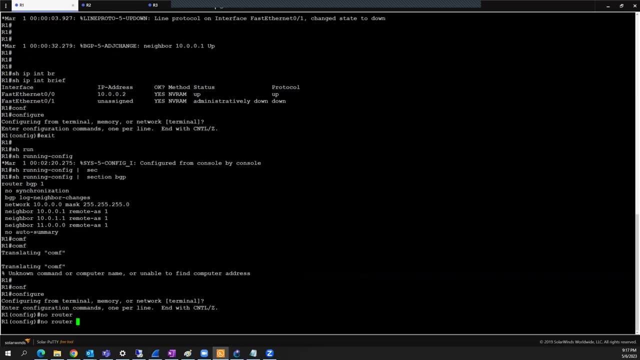 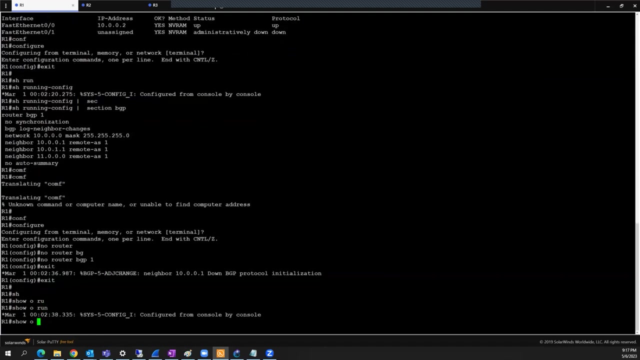 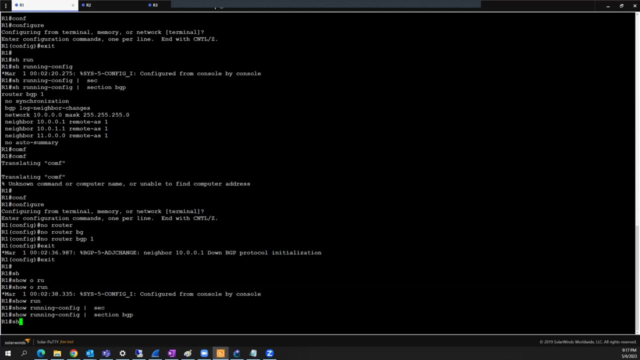 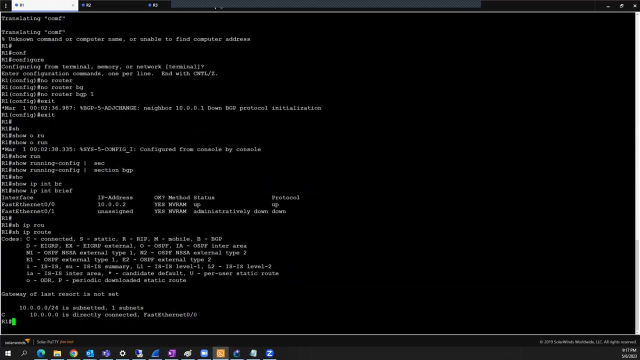 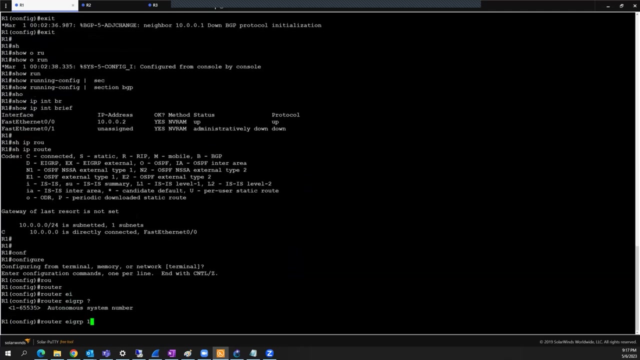 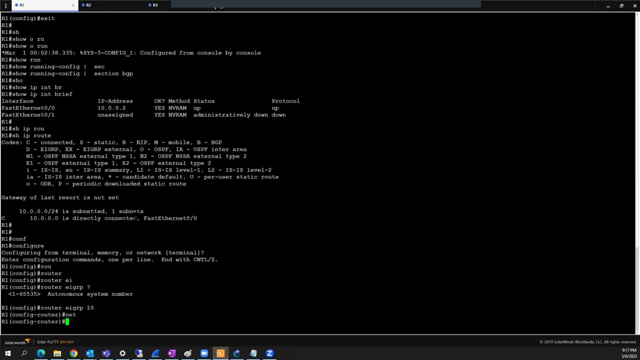 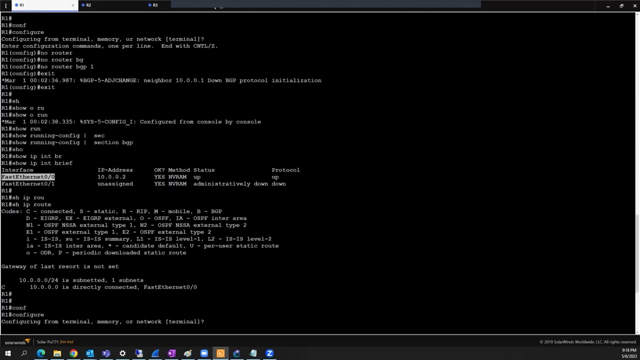 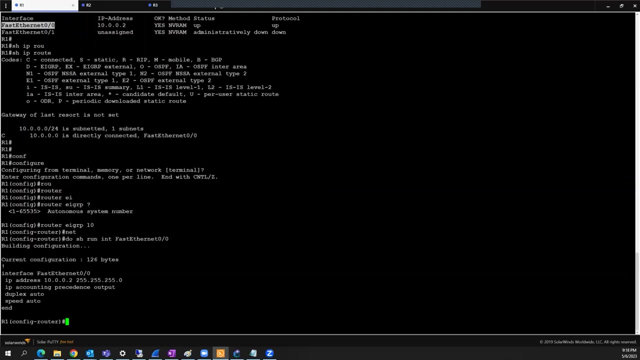 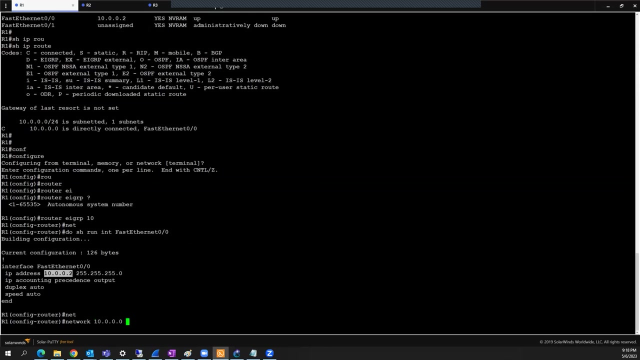 Okay, So still, it's there. So run, section BGP. Okay, So I'm going to give an autonomous number, system 10, and the network to show run. What did I give here? Autonomous number, system 10, and I'm going to advertise my network. 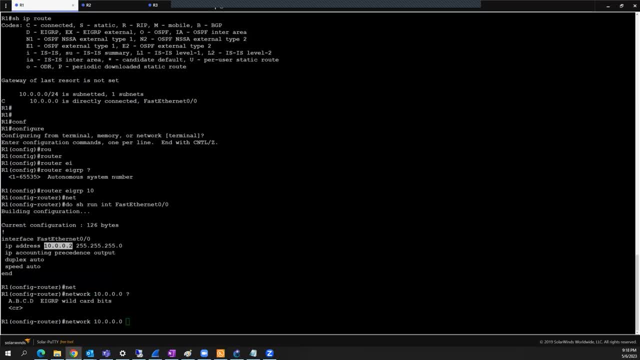 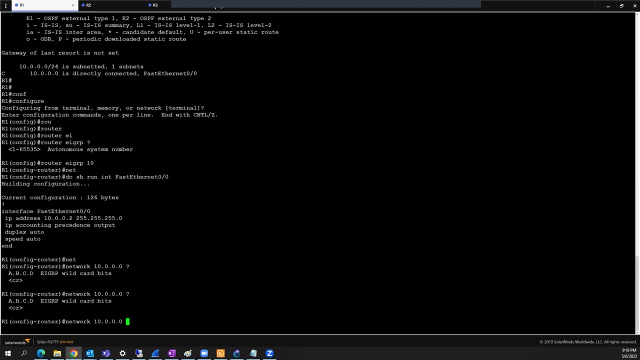 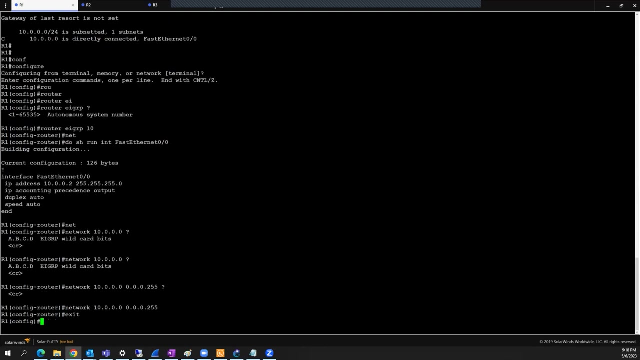 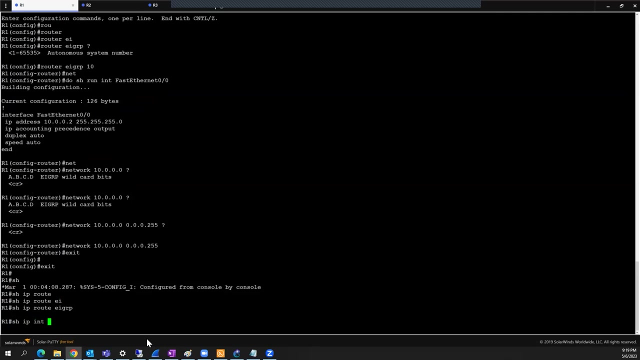 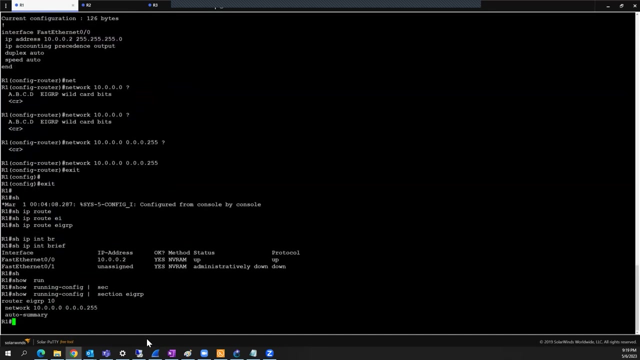 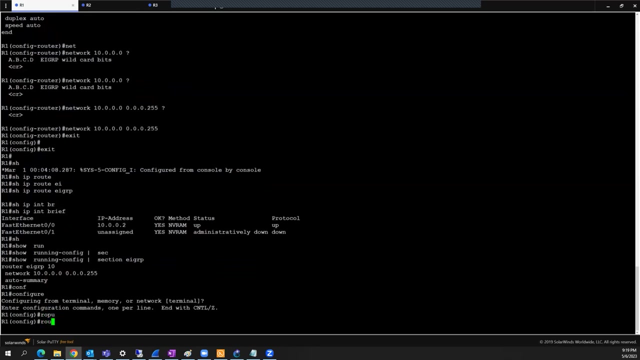 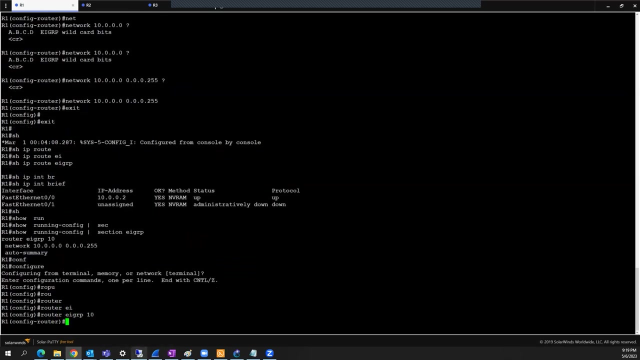 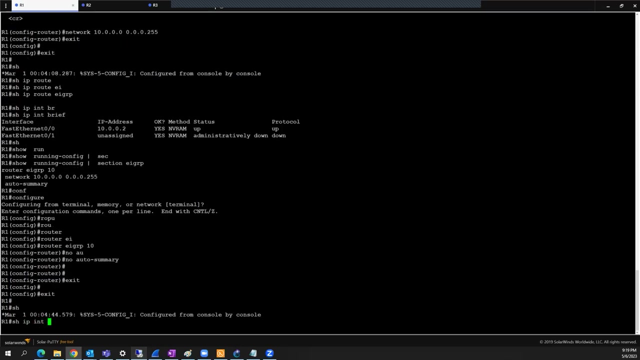 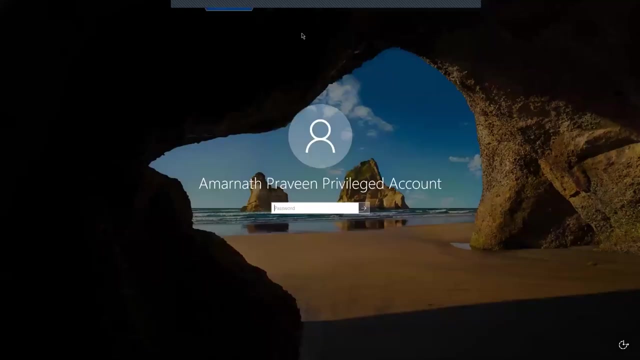 I'm to calculate the wildcard mask for the same. So it's for slash 24.. So, router EHR-P10, no autosummary. If we run it it's going to say one, two, three, four, five, six, seven, eight, nine. 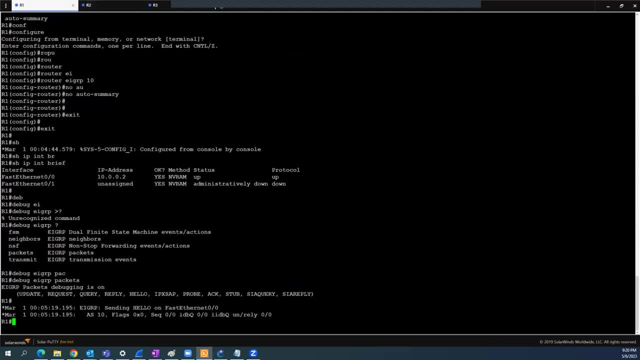 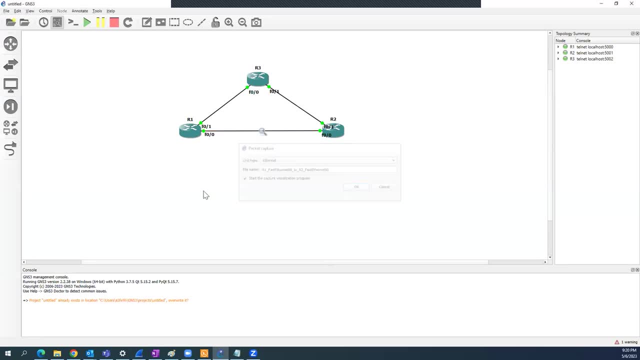 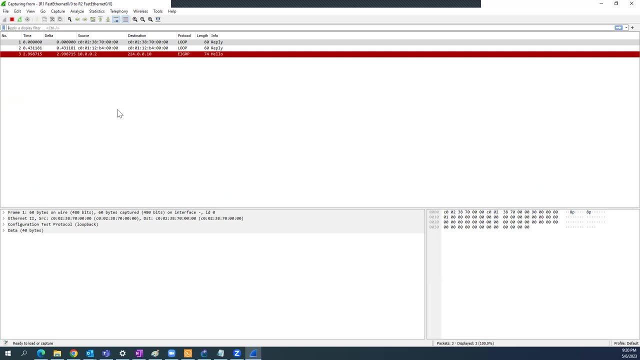 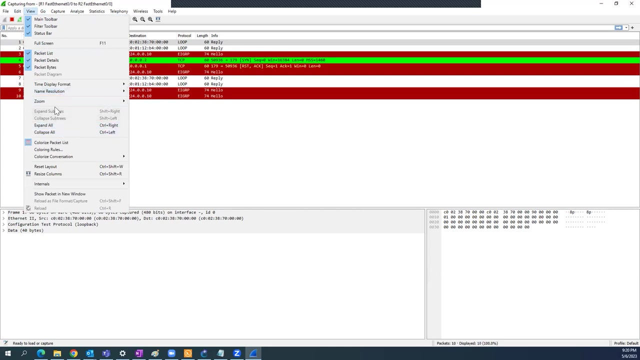 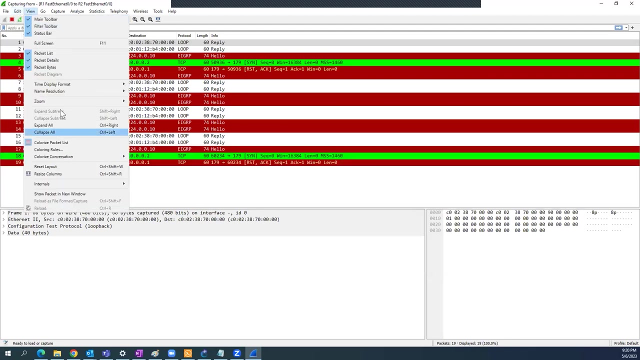 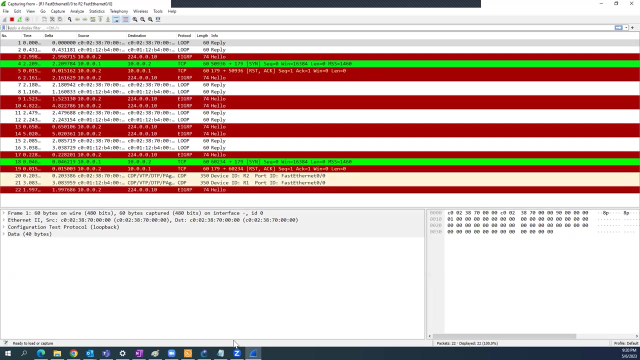 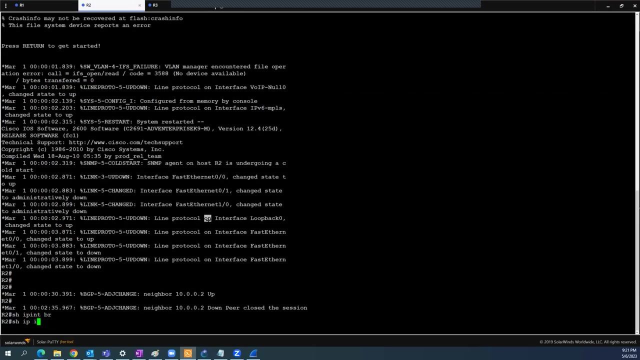 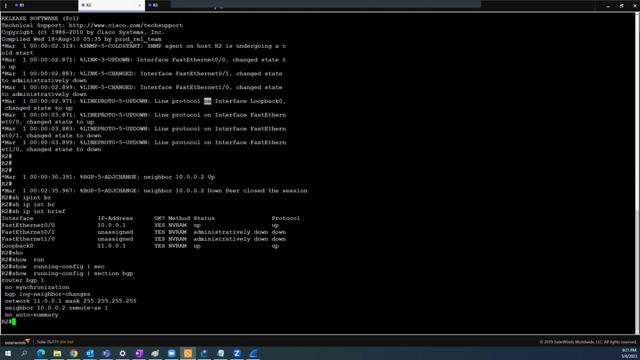 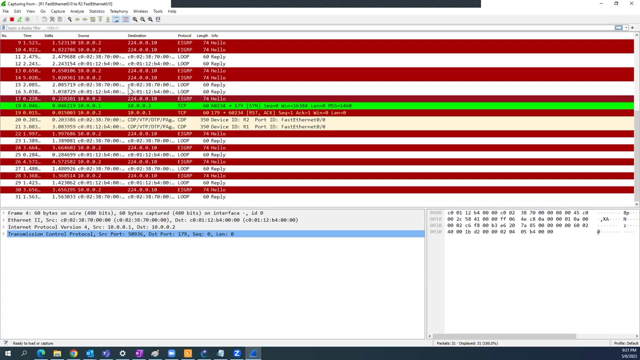 so i have turned on my debug and at the same time i'm going to do a capture. so who is sending a send? so 1001. so let's see where is 1001. i'm still running bgp, so it's a good clue, sir. i keep sending sin. 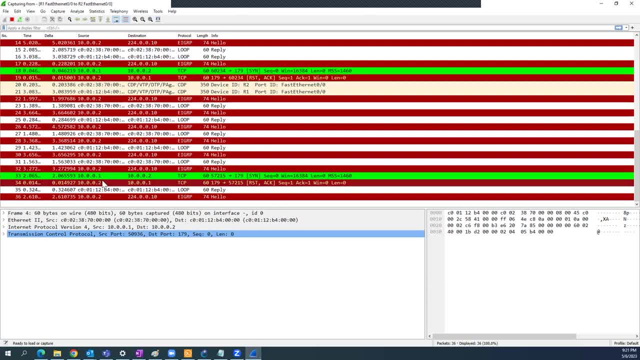 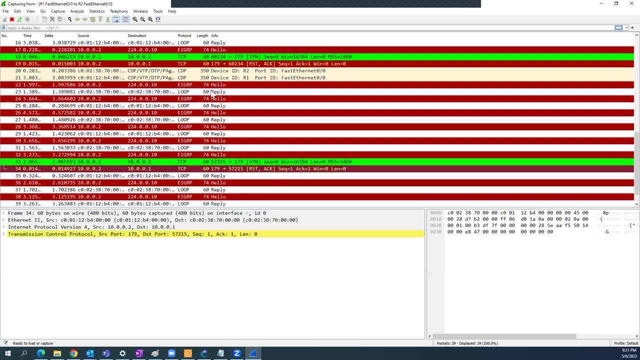 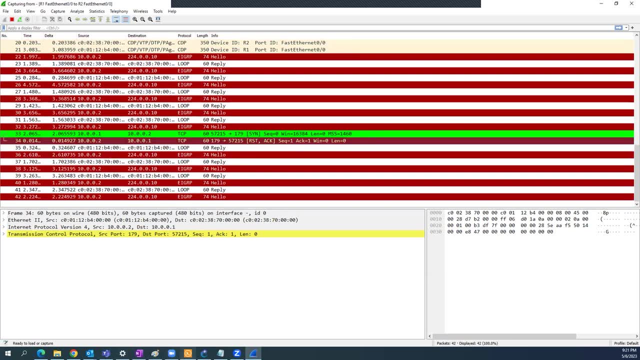 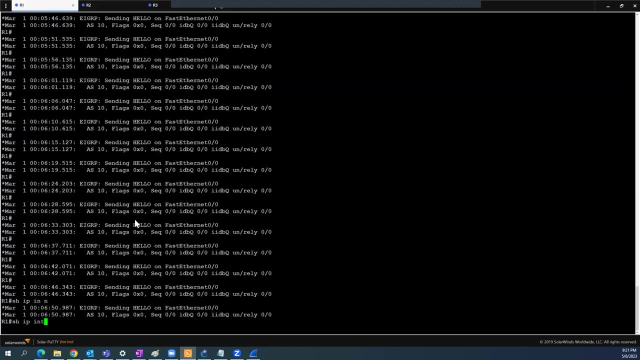 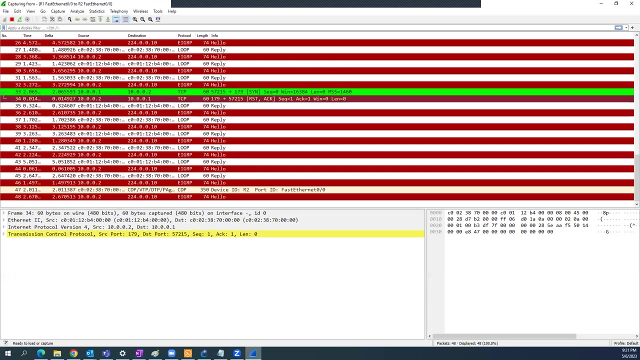 but i'm not getting a senac back and 1002 it resets the connection back because i'm not running bgp. there you can see the reset flags. so it's an indication that, okay, the remote end is not running bgp. so 1002 is resetting and it sends an hello. 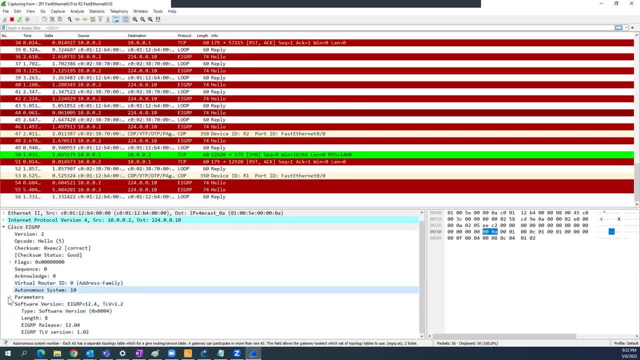 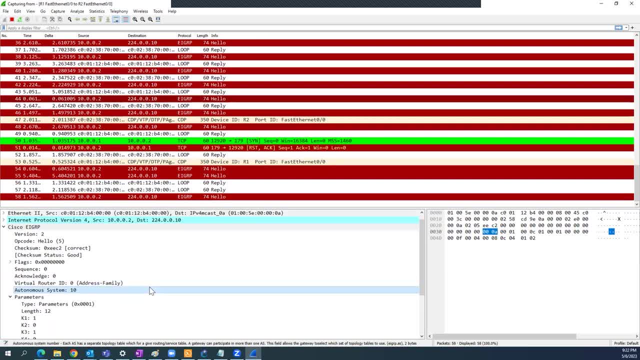 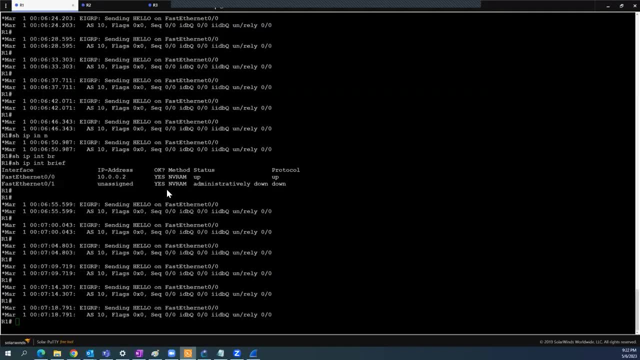 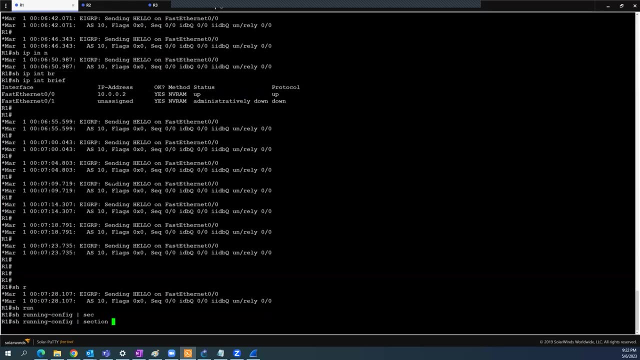 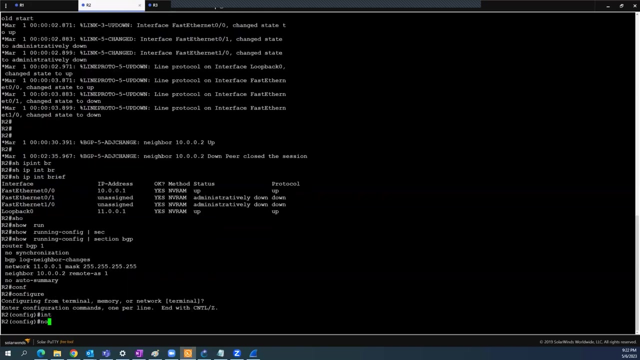 so it says the asjrp version, the autonomous number system, what i'm running, since i didn't establish a connection, so i am not sharing any my i'm not sharing my nlri information here. so i'm going to this doctor and i'm going to give. 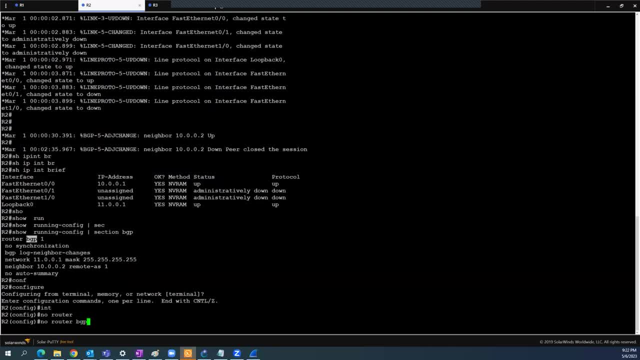 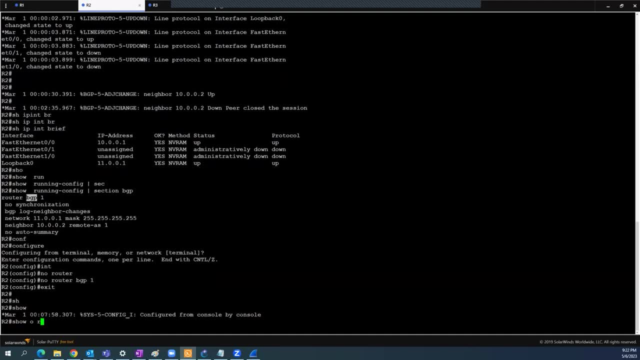 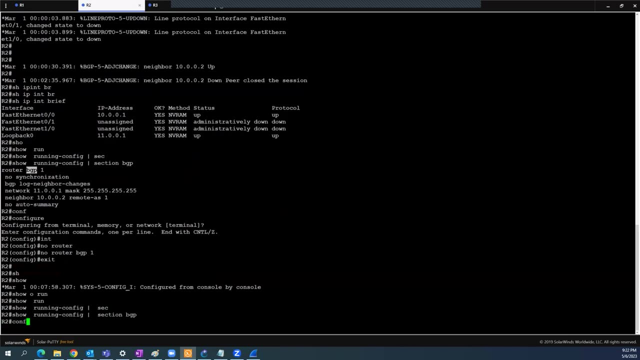 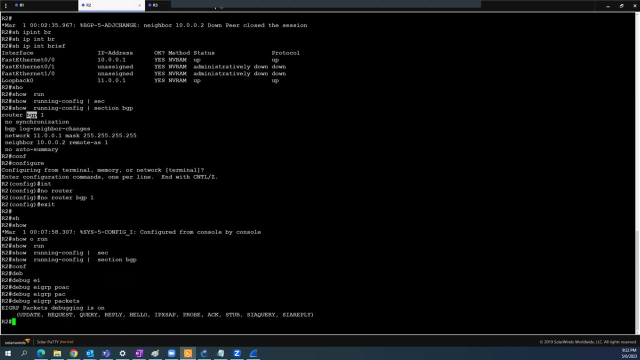 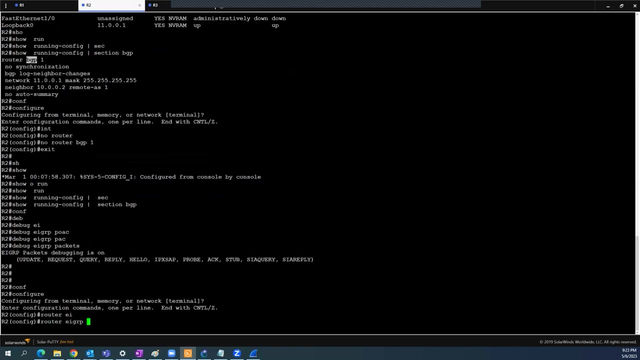 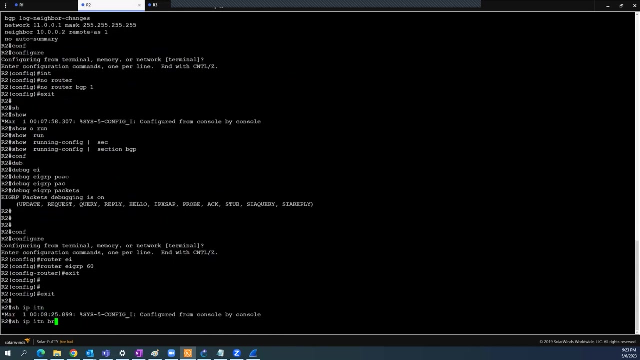 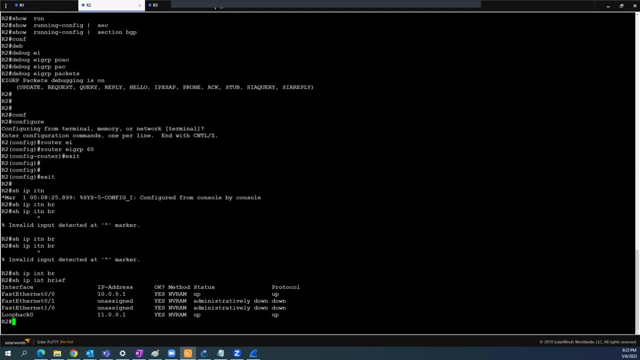 now router pgp1. so if i give show, run section bgp, if i do a debug phrp packets, so router vagrp. let me give an autonomous number, system 60, and i give show ip interface. show ip interface. show ip interface 3.. so i'm running 10 network and 11 networks. so 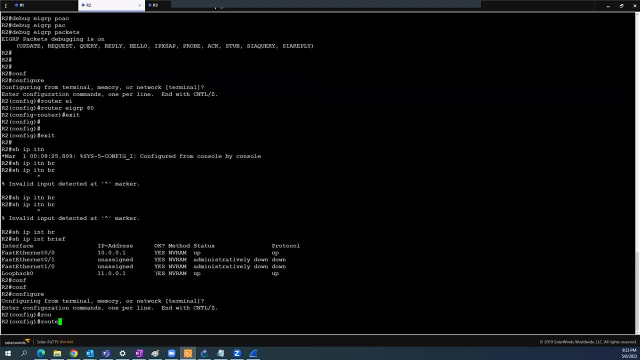 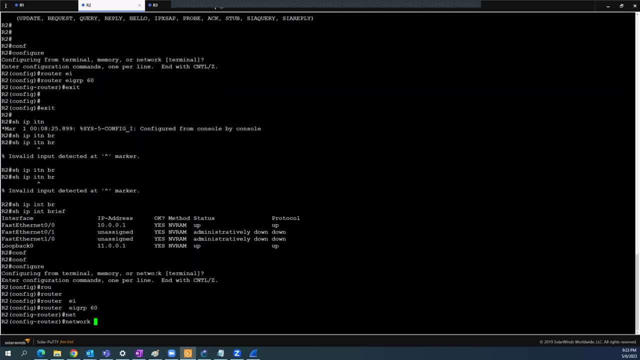 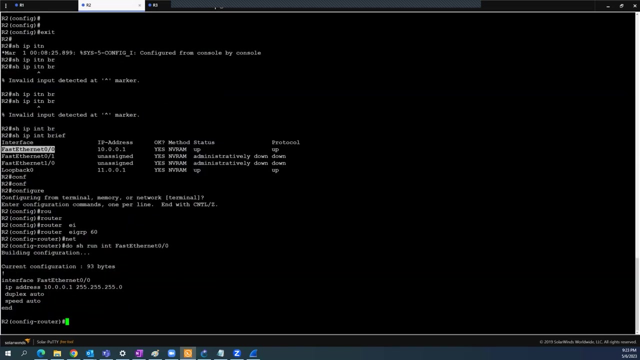 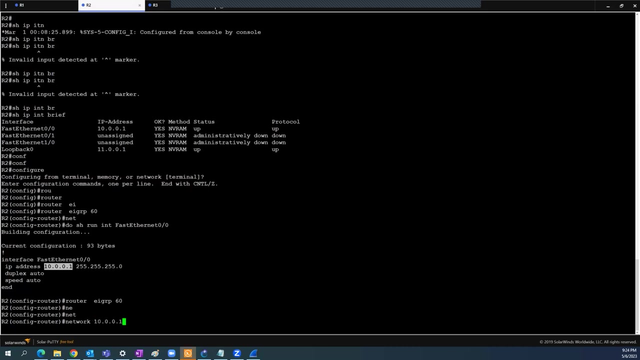 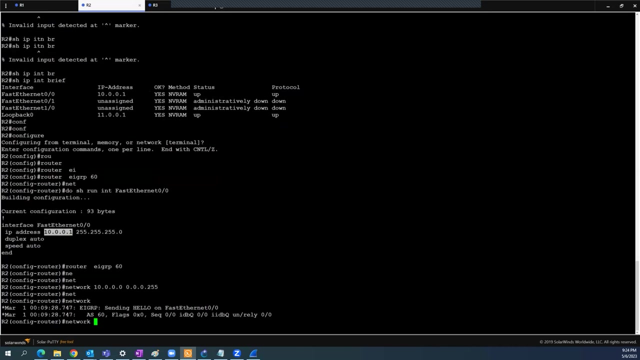 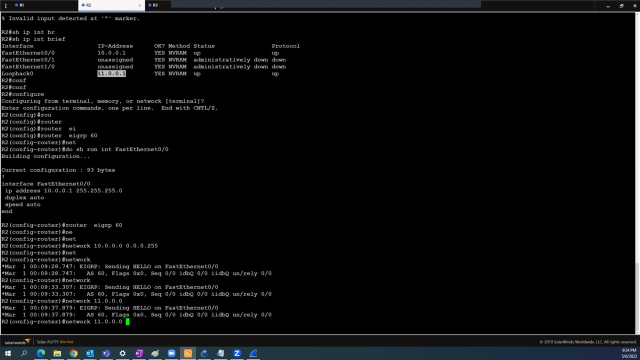 dr eagrp 60, so my network is 10 000 and my wildcard mask. do you show 1 interface pasted the 0, 0, 0, so My network would be 10.0.0.0 and 0.0.0.255 and 11 network, the subnet mask for slash. 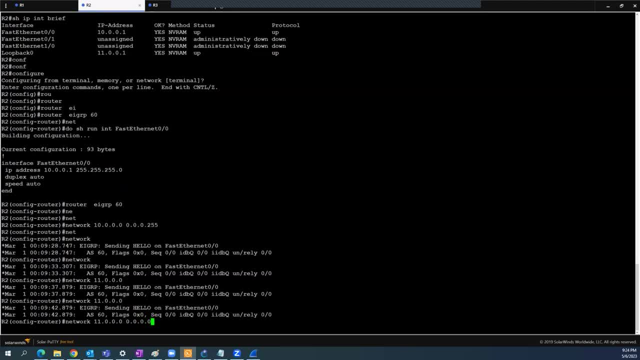 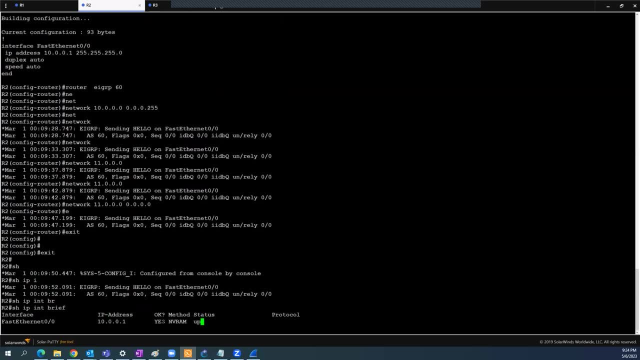 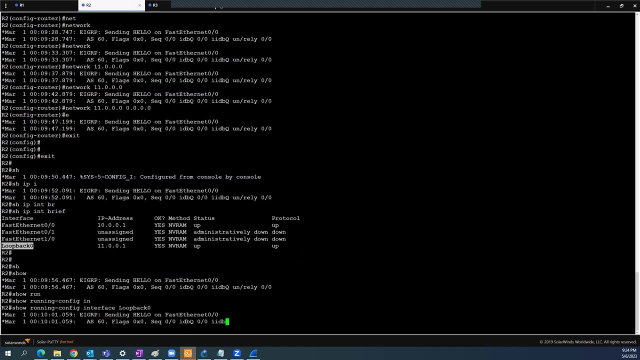 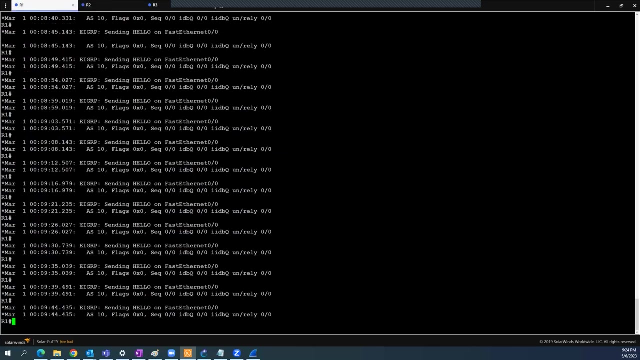 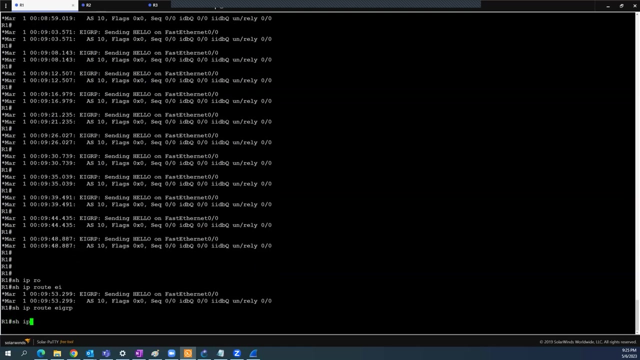 32 is all zeros. I guess that is my loopback. I'm sorry for that. so my network address is not correct. okay, let's see what I see here. show IP route. yeah, I'll try to, Julie, we went out. 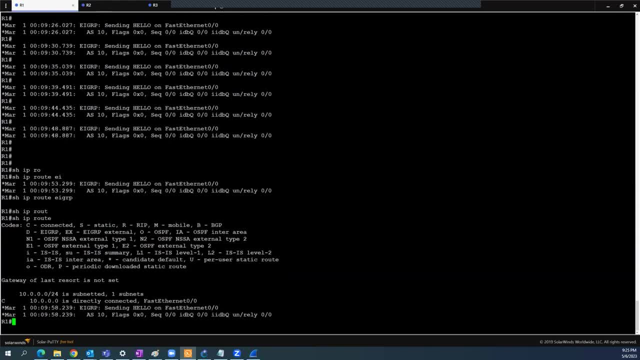 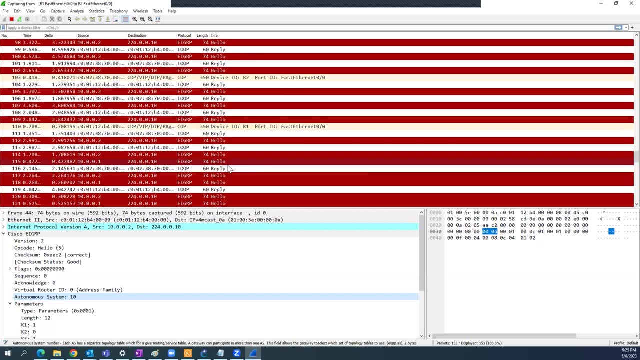 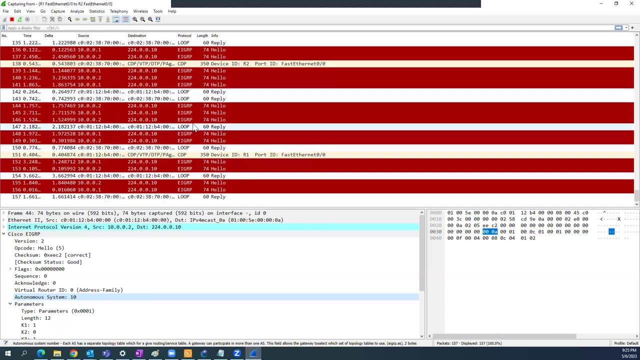 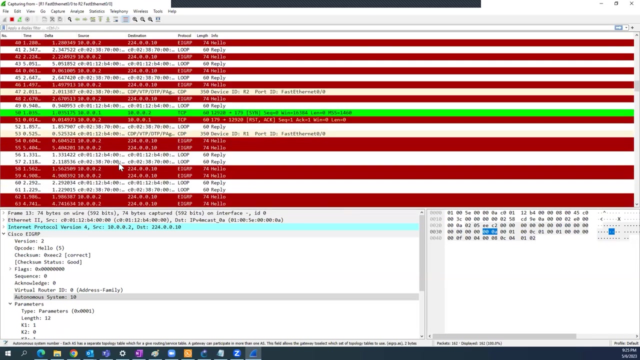 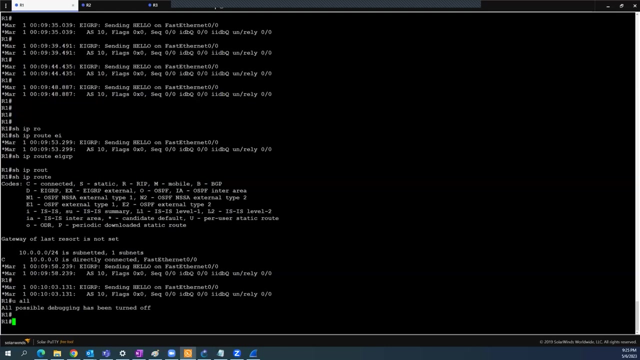 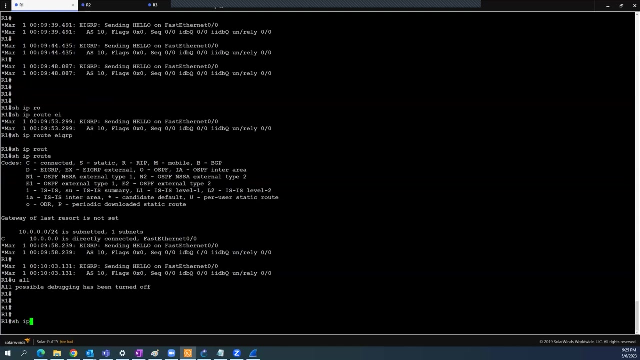 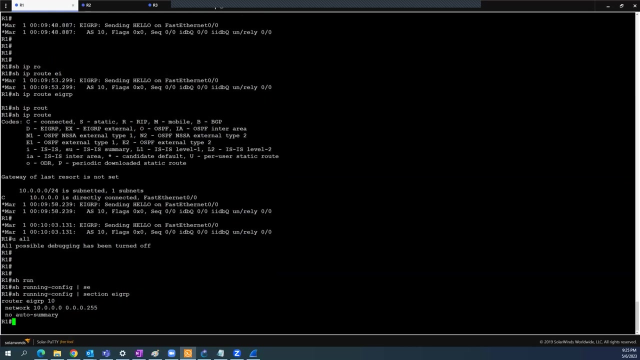 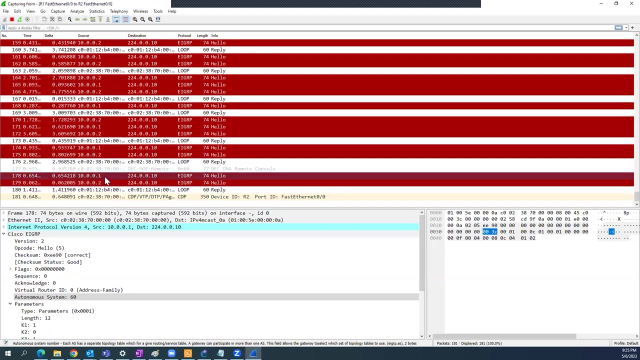 so what I see here. so still, I didn't form a neighbor ship here. yeah, because my Autonomous number system is incorrect: Show run section EIGRP. So it is still sending in hello. Both are sending in hello to the multicast address. 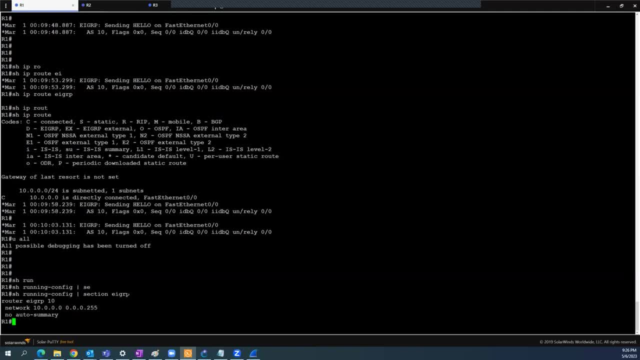 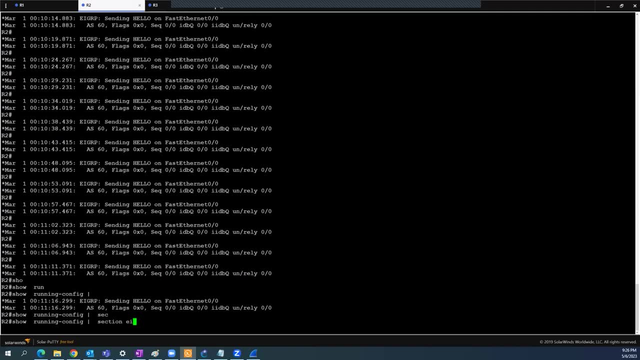 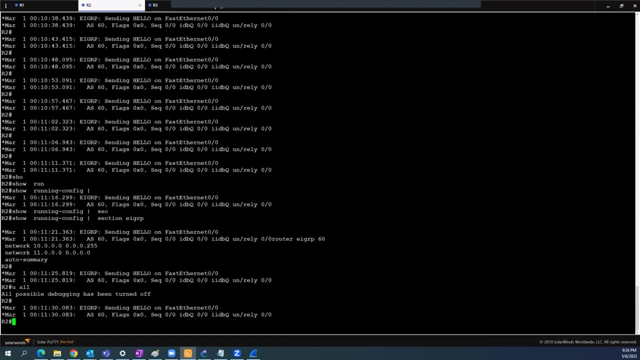 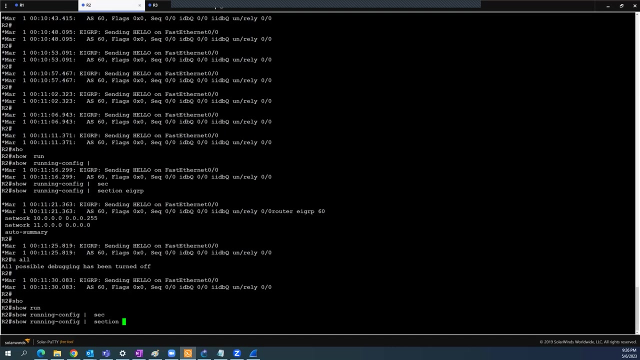 One to team team Next and AF relay is sending the survey question thickening to staticнул vaccine Next and the message is sending to AF an Congress survey by the American Essex Pharmaceutical Administration, But it will still send to AR. 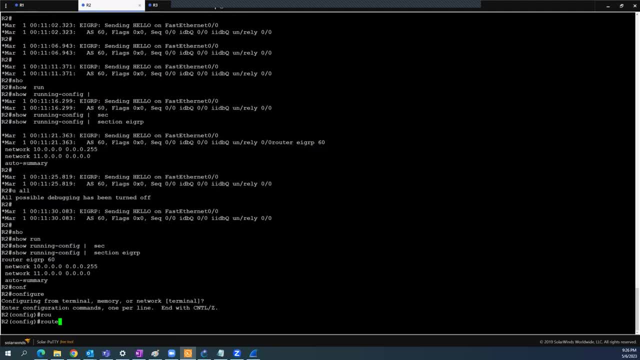 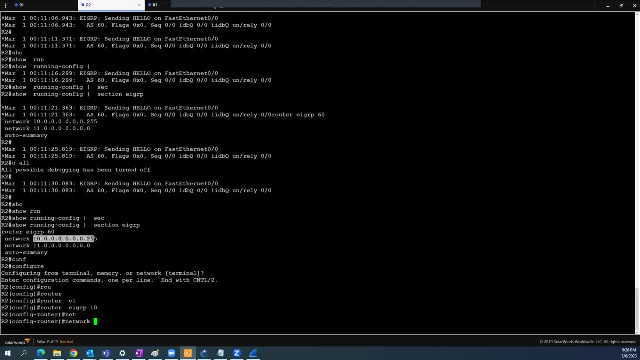 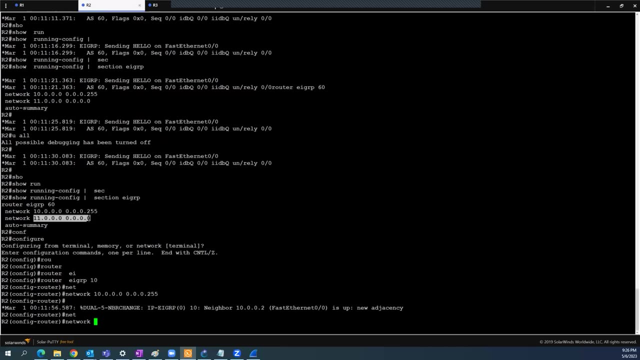 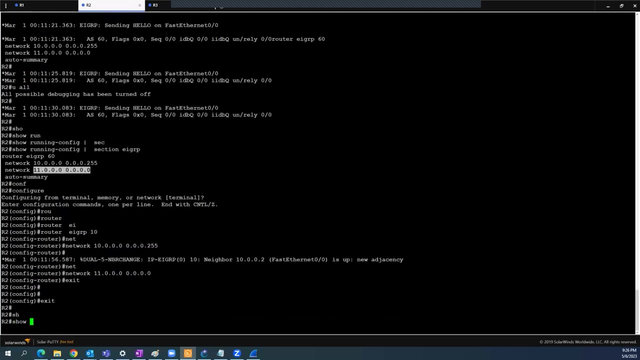 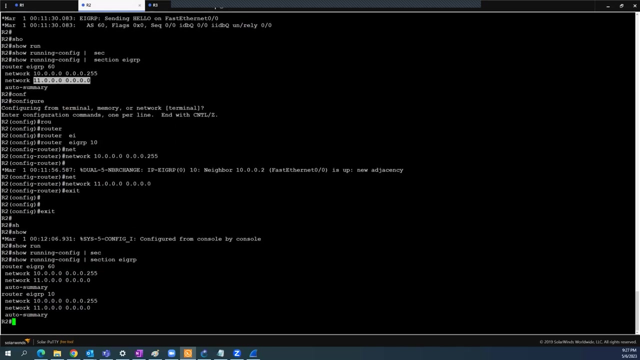 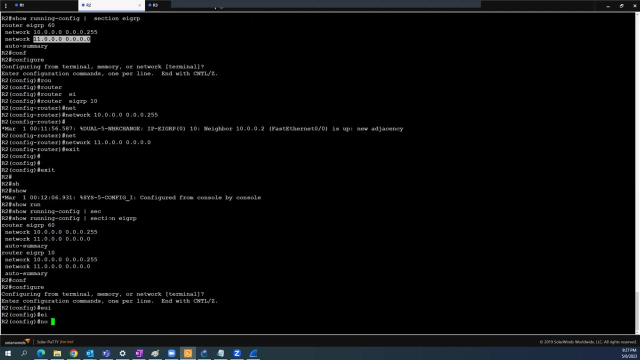 which didn't send the Zapf result. So I'm going to change the network by NLRI and I see the adjacency is up and if I give show one section EHRP, So I'm running two EHRP process. so I'm going to delete router EHRP 60.. 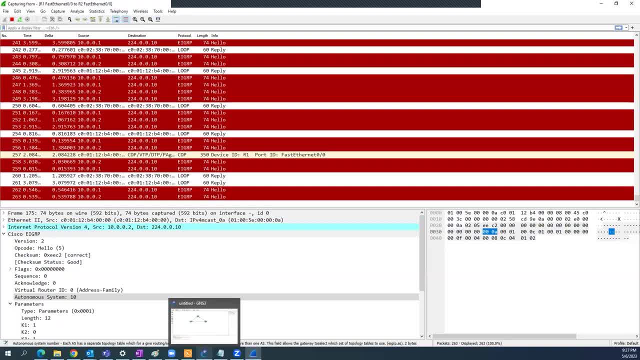 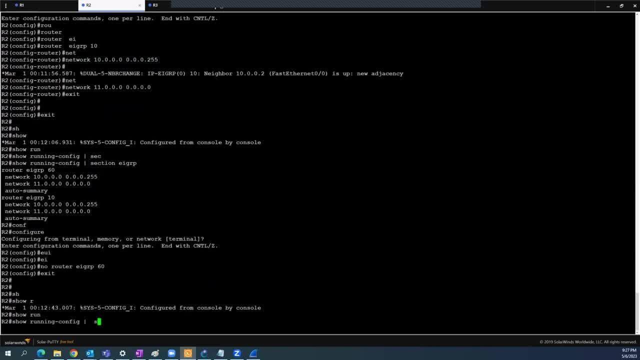 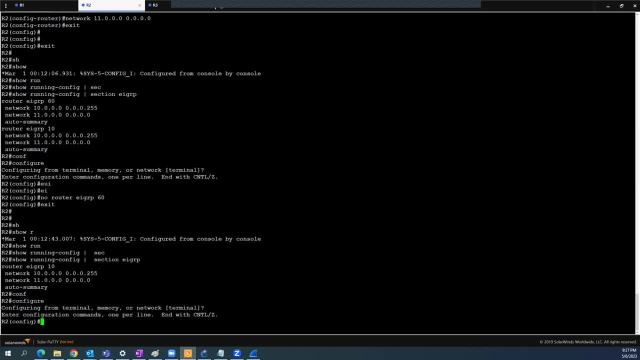 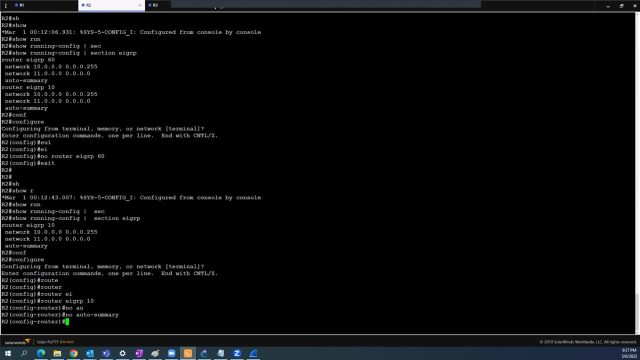 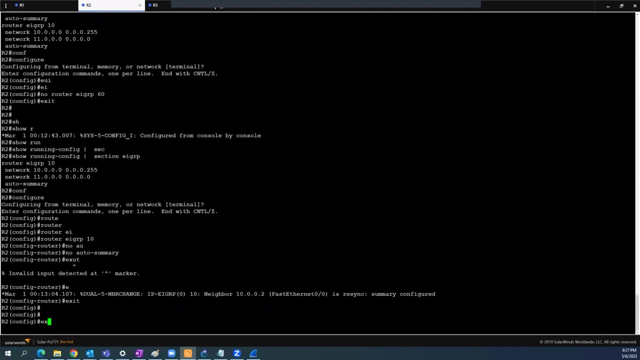 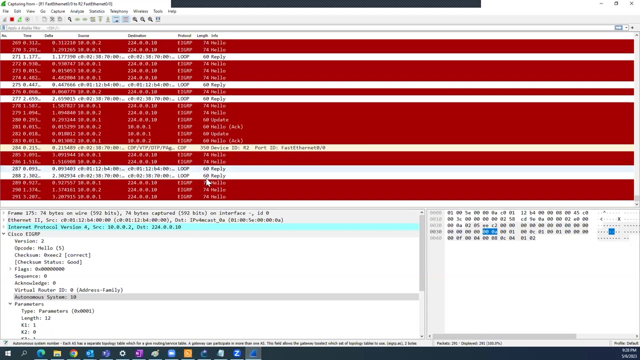 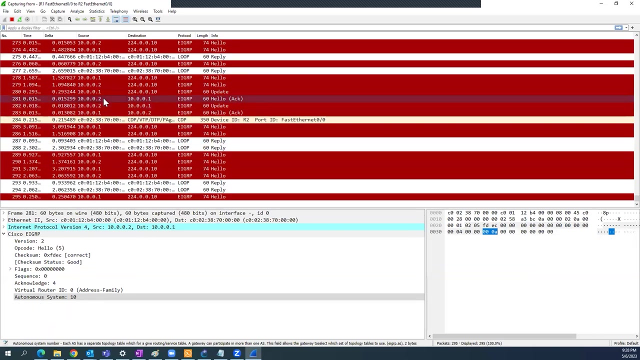 Configure router EHRP 10 and turn off autosummary session. no autosummary. If you see, now I can see an update that's been exchanged between 10.0.0.2 and 10.0.0.1. 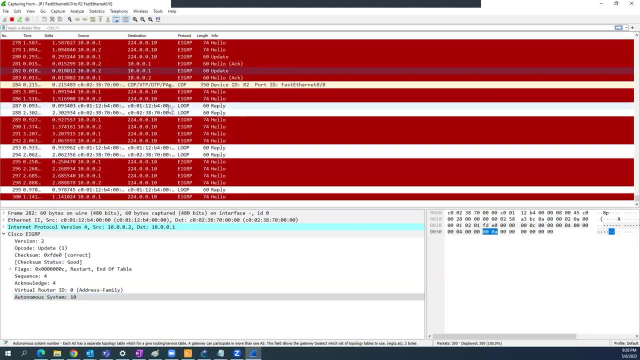 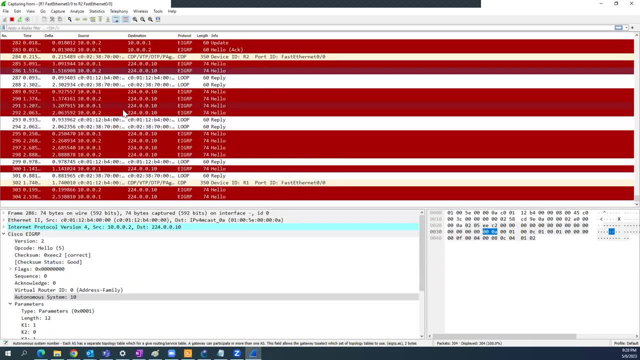 and I can see the autonomous number system. So earlier my autonomous number system is incorrect, so I didn't form a neighborship at all. I think that is fine, So I'm going to update the database. at the moment I'm going to use the tesla to test the data. 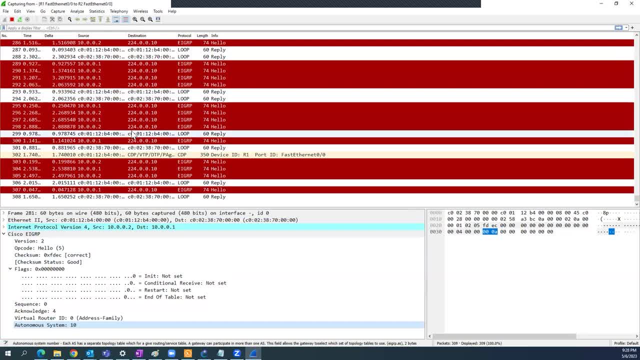 So I'm going to do that. So the details are there. I am waiting for the data entry. I'm going to see that an error has been created in the database. I can see that the channel is not working. This is an error. nonetheless, I'm not clicking on it. 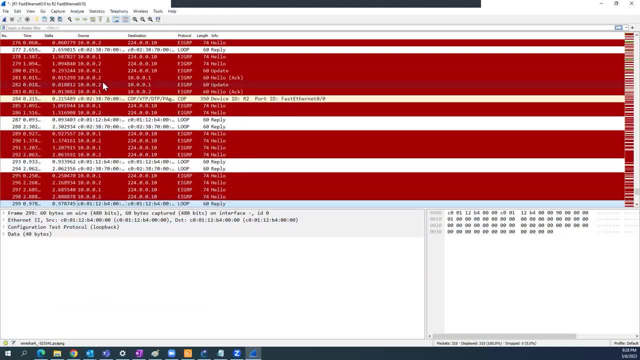 I'm going to close the test and see how it works. So I'm going to push the notifications and image and the data is changed successfully. So now it's working. So I don't have to wait any longer. So the data is checked and I'm seeing the results. 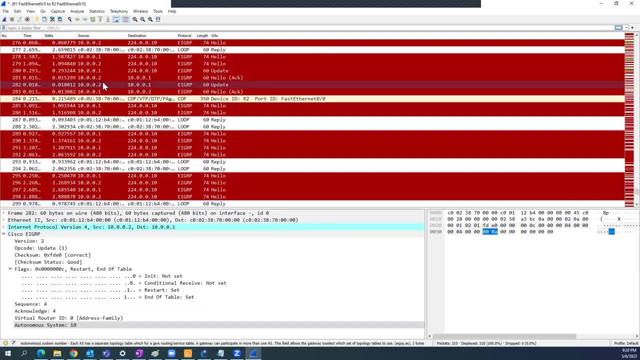 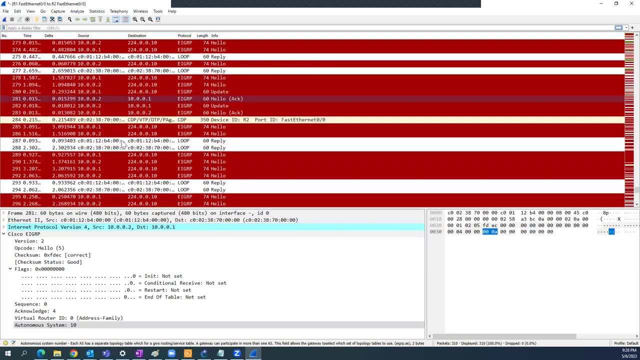 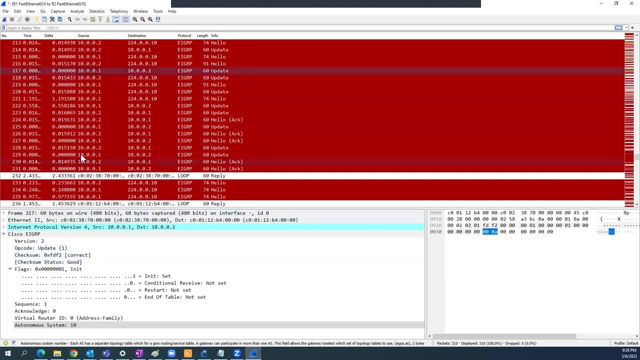 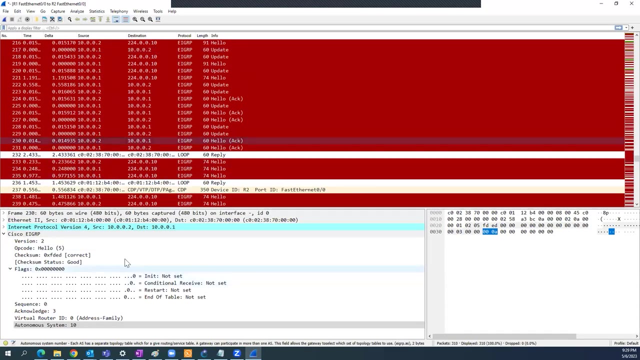 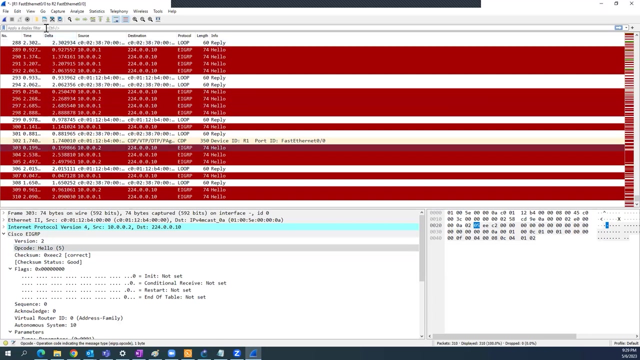 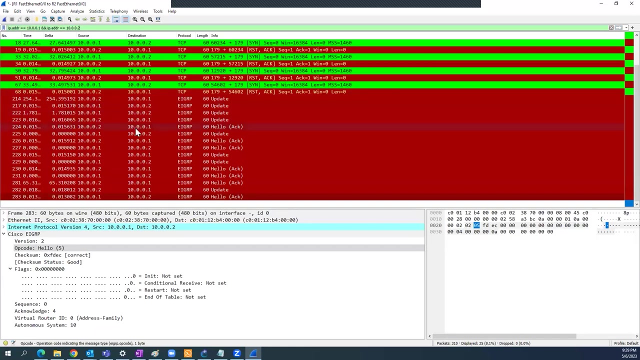 So you guys can see what is happening in the database. It is not working. The data is showing the new network. you ipaddress 10.0.0.1 and ipaddress equal 10.0.0.2. so this is all the bgp connections. 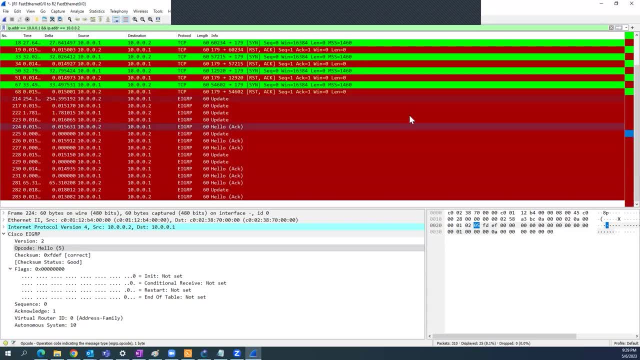 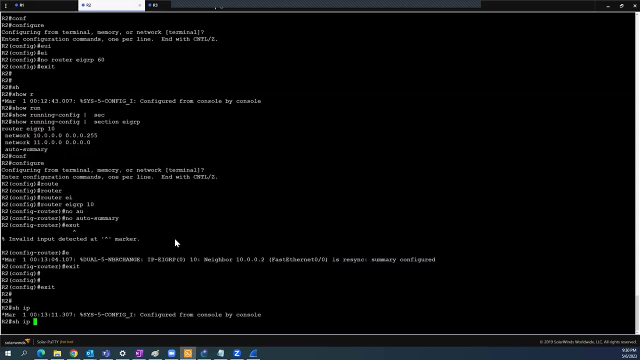 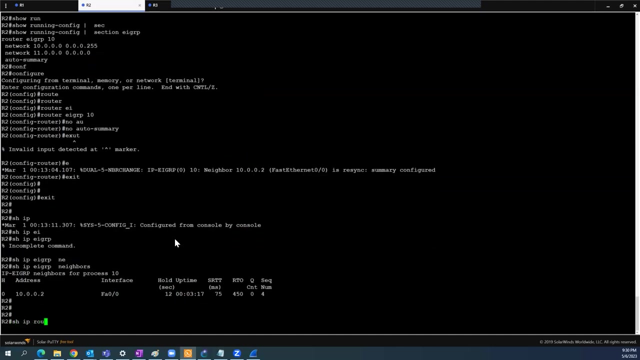 earlier. so i'm not using the bgp anymore. so now i don't see any sin packets. that's been exchanged. all i see is only eigrp and then from both. it says my autonomous number system is stem show ip route, so it prefers a directly connected show ip route. 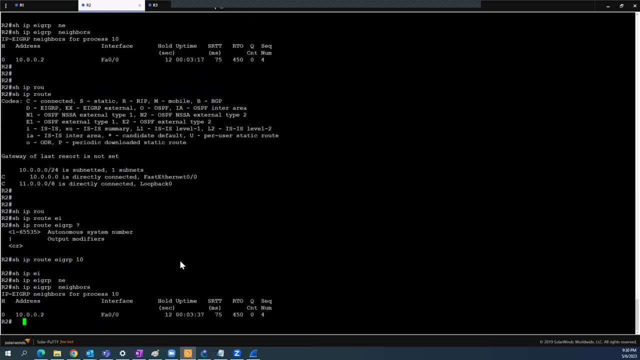 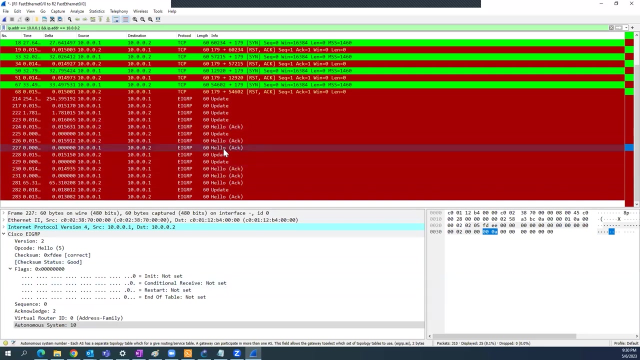 eigrp neighbor. so hold on times 12 seconds and i see the interface where i configured, so where my active bgp connection has been established, and i can see the same thing here. and also you can differentiate your acknowledgement. it says acknowledgement one, acknowledgement two. so whatever the information that's been exchanged,